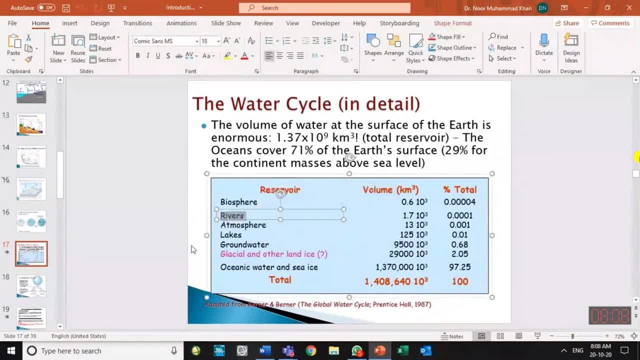 the water which we are using is normally the river water and the groundwater we are using. the river water is 0.0001 percent of the total water. 0.0001 percent of the total water. in quantity terms, it is about 1.7 thousand kilometer cube. one points 1.7 000 kilometer cube. 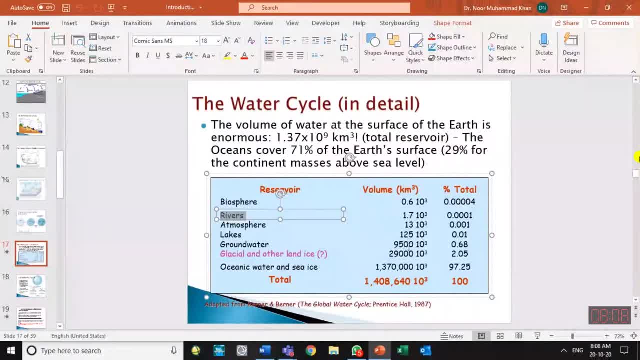 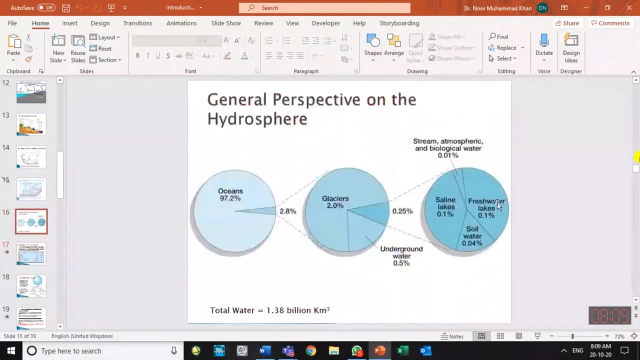 while the water in the ground, which may be saline, which may be fresh groundwater, has both kind of water. so 95 000 9500 000 uh is the reservoir available as groundwater, groundwater a that is about 0.68 percent. out of this 0.68 there is some fresh ground water and there is some 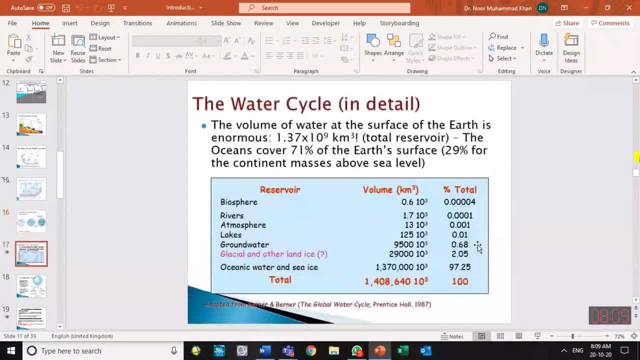 saline groundwater. not all is fresh and fresh and saline, i think i told you. if the desired starts at less than thousand ppm- hope everybody knows what is the ppm. if it is thousand parts per million desired starts or less than that, we say: what is fresh, good for agriculture purpose, fresh or saline with respect to agriculture. 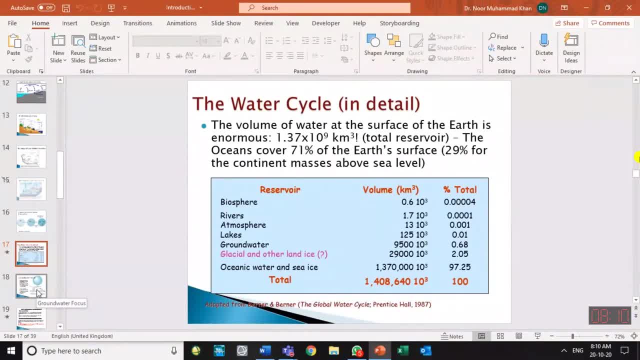 with respect to drinking less than hundred ppm or more be requirement. there should be no smell. drinking purpose, agriculture. thousand ppm. we call it fresh water. fresh water is fresh water. fresh water is fresh water. resources in rivers are quite limited and we are harnessing, we are using this resource. 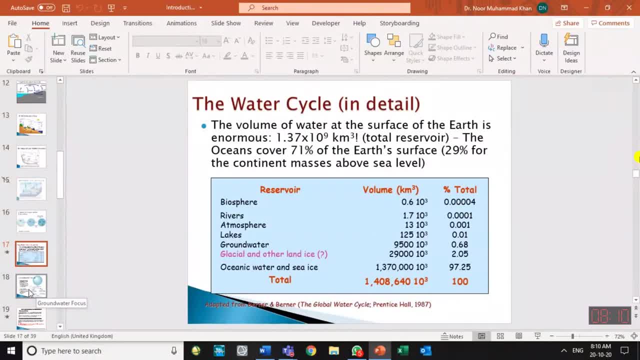 in the first instant. when this is not available at a place, then we go towards groundwater because we have to lift it up. surface water, we use it through gravity without any excessive energy, artificial energy. we don't have to apply so much. we stop it, we store it, we release. 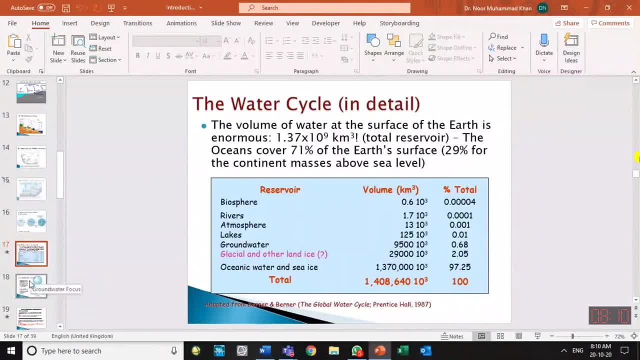 it most of the time through gravity, while groundwater may have a lift that number, but that is when we need energy. so initially, animal energy used to be employed, and now mechanical energy and electrical energy, motors and pumps are being used to lift the groundwater. so it will be. 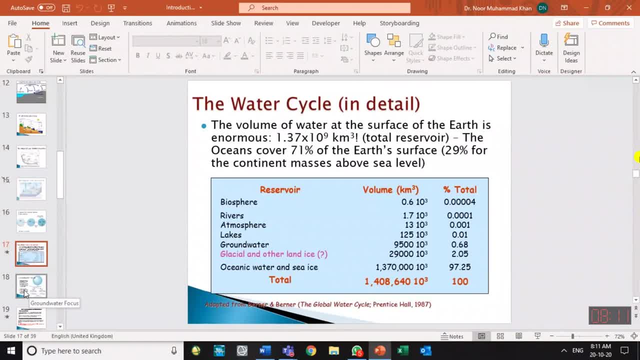 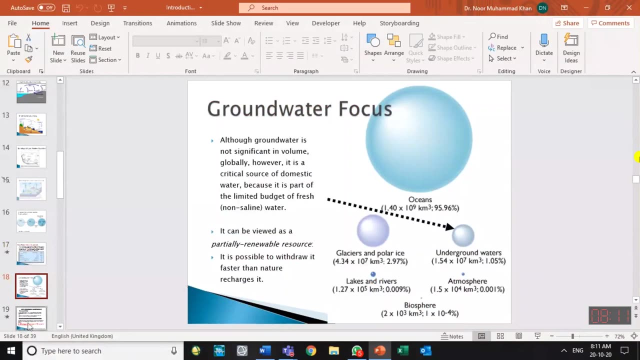 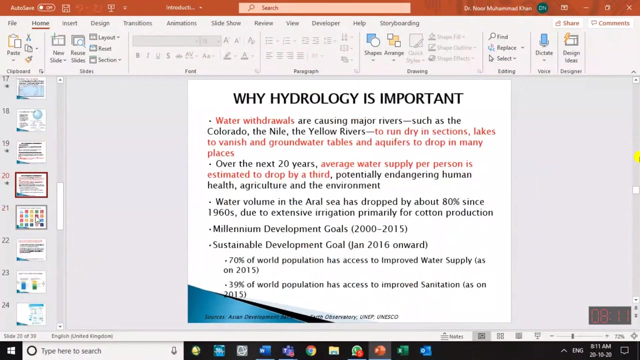 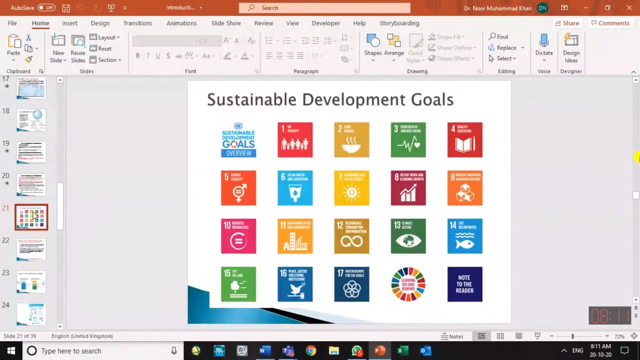 extensively use order groundwater most most of the urban water supply to the cities and the villages, most of the supply to the cities is the source is ground water. okay, volumetric terms then. importance of the water. sustainable development goals: this is not directly hydrology. sustainable development goals scenario: world have thought that all the countries of the 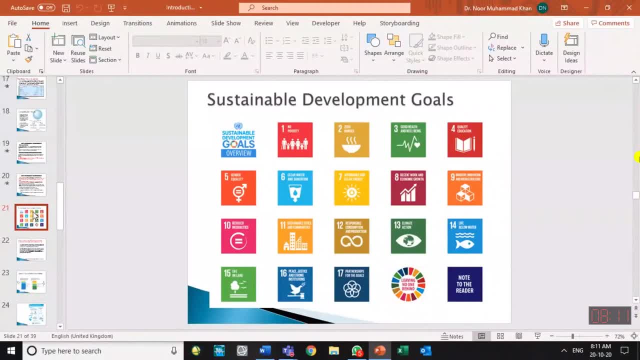 world have thought that if we set some goals for us, that is good, we will be moving in a focus direction, joined together under the umbrella of United Nations. and then they fix some goals. initially they fix some goals, I think in 2000. they call them Millennium. 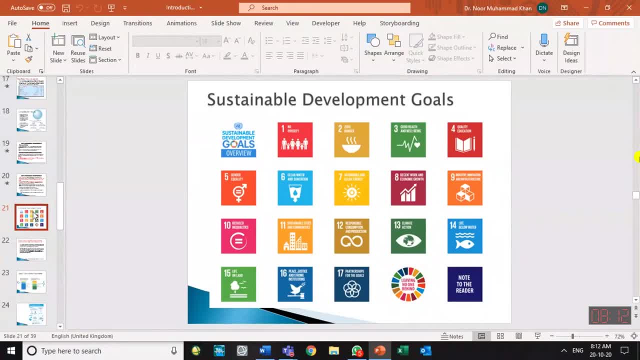 Development Goal. later on, when those goals time period was finished, they fix the goals for 15 years. 2000 say 2015. so in 2015 they joined again, they met again and they reviewed their progress and there were some good success stories and they continued the way of development through fixing. 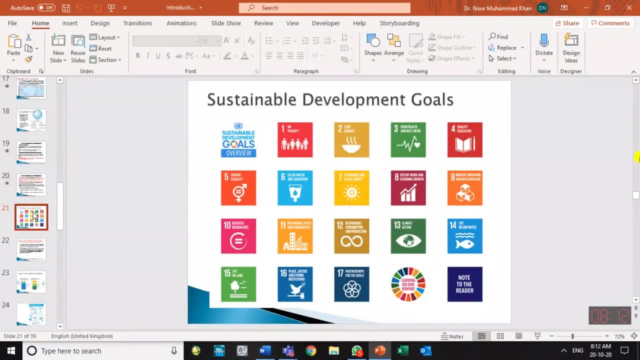 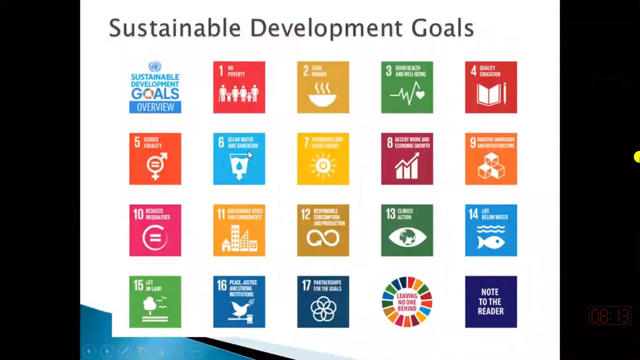 some goals, so now they call these goals are sustainable goals, sbg, sustainable development goals. so there are 17 sustainable goals. one goal is directly related to water. that is goal number six, if you see these goals. one goal is directly related to water: provision of the clean water and the sanitation. sanitation is providing some facilities so that the 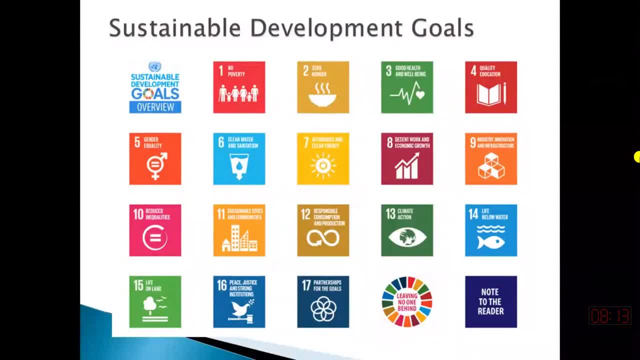 sewage water. the surplus sewage water from the, from the developing sewage water from the urban areas can be safely disposed of to the destination or nala river. so that is sanitation. so bulk of the humankind has not yet achieved the safe sanitation facilities. and a big, a big 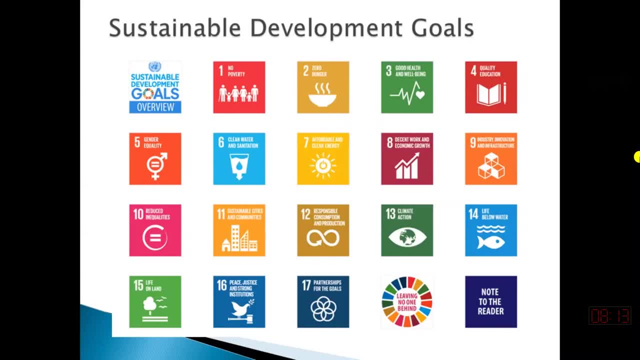 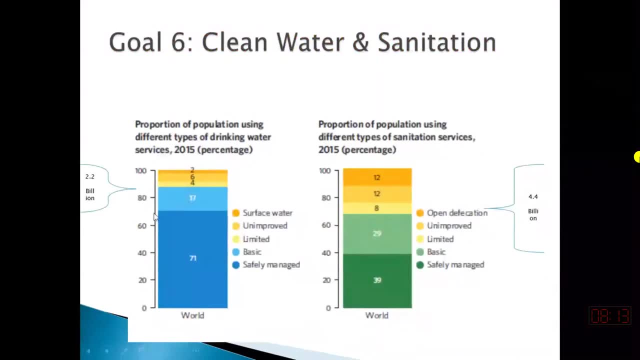 proportion of the population of the world don't have access to safe drinking water condition. in 2015, this was a condition that 71 of the population of the world had access to safely managed drinking water. city, which were only relying on surface water. percent of the work getting 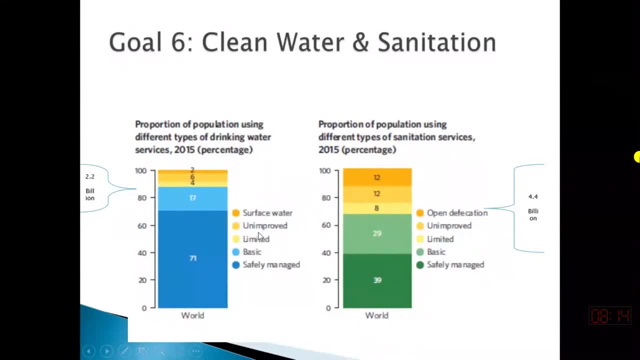 work on surface water, so In Pakistan people are still relying on surface water in many areas like Jolistan and Thar. There are ponds there which are also dependent on Corona. Unimproved water is available and some people have water with limited improvement. 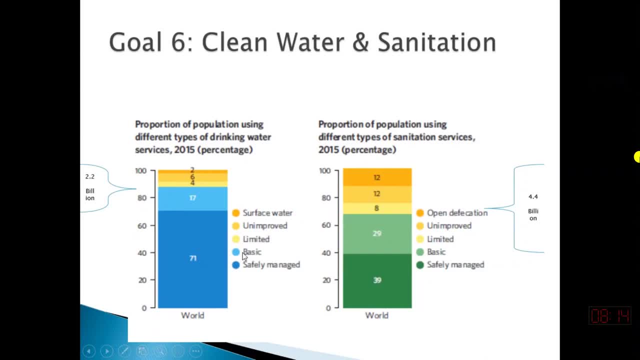 Basic facility of water is available, but not safe. 17% of the world have access to safe drinking water And you think that water is a basic necessity. Without water we cannot live. Not 100% have access to safely managed water. 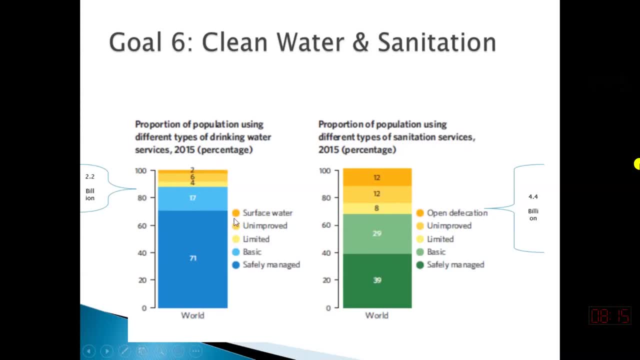 Sustainable Development, Goal 6 says that we have to provide safely managed drinking water To all of the population. If we look at sanitation, the right hand column shows the conditions of 2015.. Only 39% of the population had access to safely managed sanitation facility. 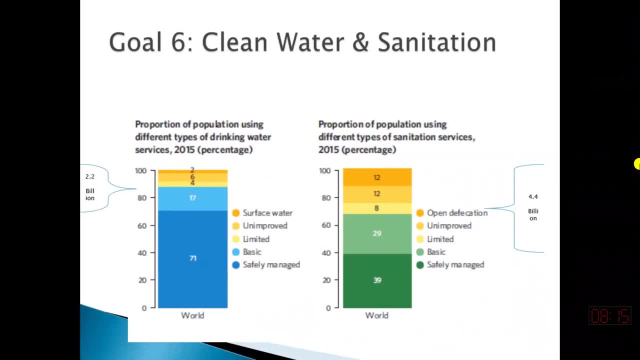 Safely managed means that our sewage disposal system in Lahore or in urban areas in which sewage material is taken away from the area through a sewage pipe, Then it is treated, And then it is used, And then it is released to the natural bodies like rivers. 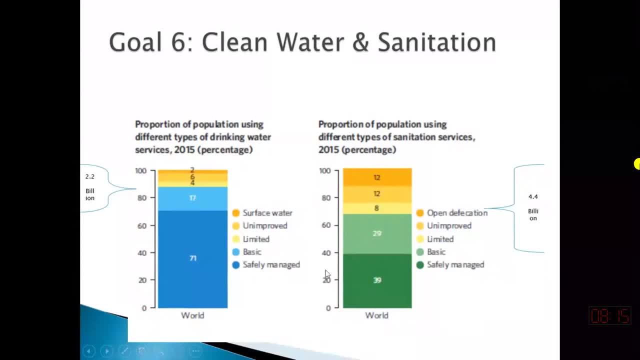 Only 39% of the population have the safely managed sanitation facility. If we look at it, if 7.5 billion is the total population of the world, then almost 2.2 billion do not have safely managed drinking water. Out of 7.5 billion, 2.2 billion do not have safely managed drinking water. 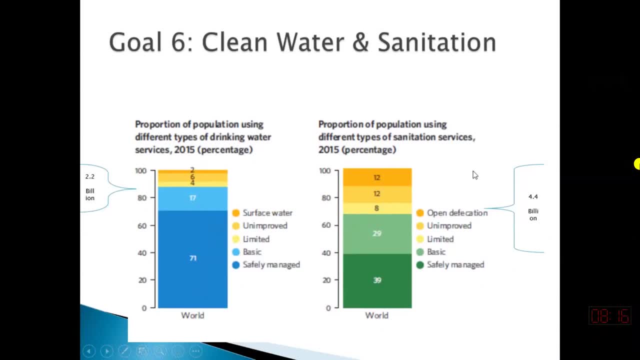 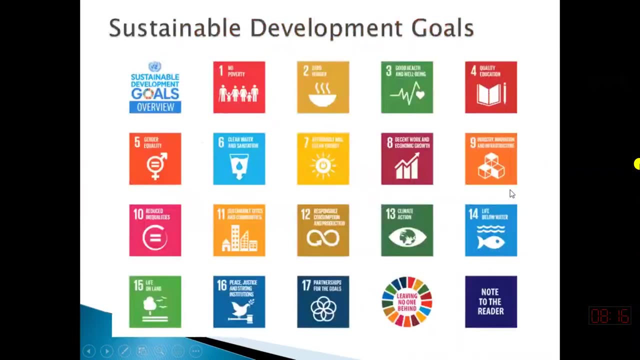 And 4.4 billion do not have access to safely managed sanitation facility. So these were the conditions. when they said SDGs, They fixed the SDGs and then they emphasized the countries to provide effort, to put more efforts so that the clean water can be supplied to the 100% of the population. 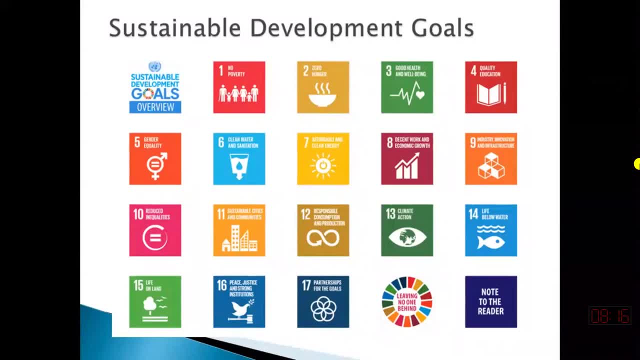 And sanitation facility can also be extended To the double of the current population in the next 30 years. Okay, This goal number six is directly related to the water: Provision of clean water and provision of sanitation facility. This is related to your WASA institution. 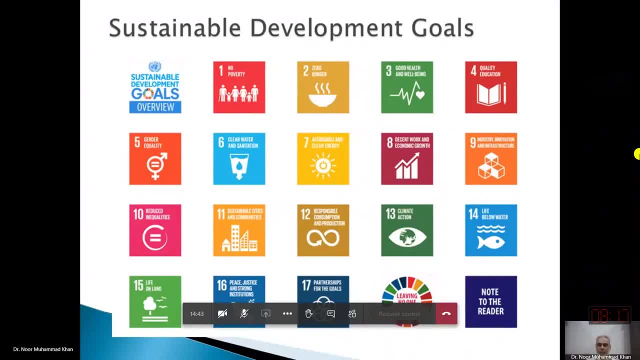 In some places there is an institution of WASA. In some municipalities we call it public health engineering. This is a sustainable development goal. It is related to the main activities of their institution. But if you see other development goals, it has been seen that many other development goals are dependent upon water. 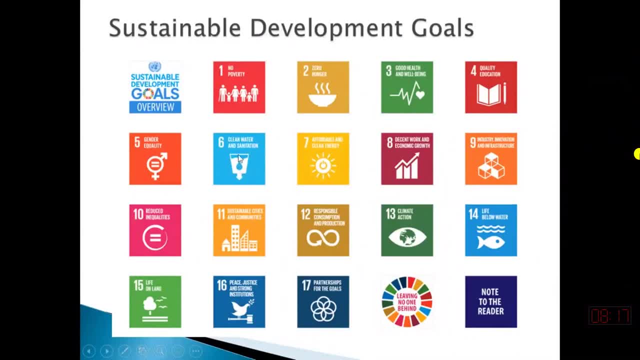 They are highly relying on the availability of water, water resources. Any one of these can you name? which one is dependent upon provision of water? If you look at the Sustainable Development Goals, the first one is related to poverty. They want that there should be. 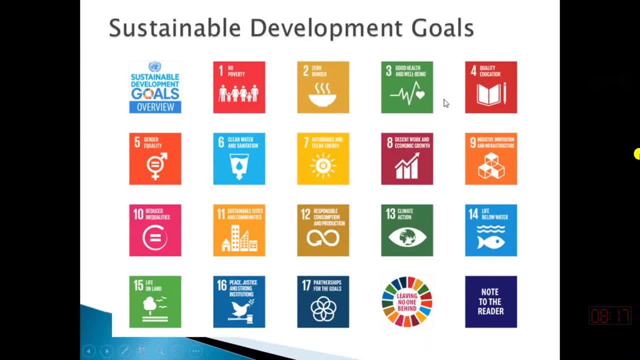 They want that there should be no poverty. Anybody have idea how to define poverty, How to define whether a person is poor or not poor. The access of basic facilities: sir, This is a general thing, right? They have quantified this. 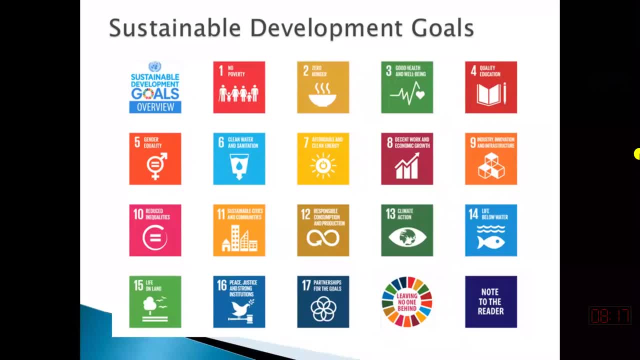 Yes, sir, Anybody else. This is a general thing that there is no basic facility. No one will say that basic facility is this or that. The definition is that if a person or a family, if a person or a family don't have earning equal to one dollar a day, 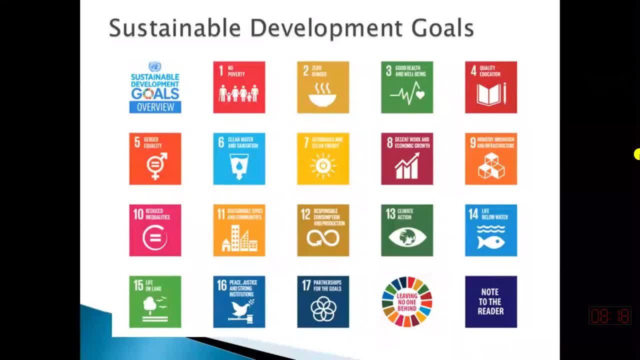 how much? One and a half hundred rupees. Nowadays it is 60 rupees. Then they say: they categorize it as poor person. So if a person has earning less than a dollar, so they say that he is a poor person. 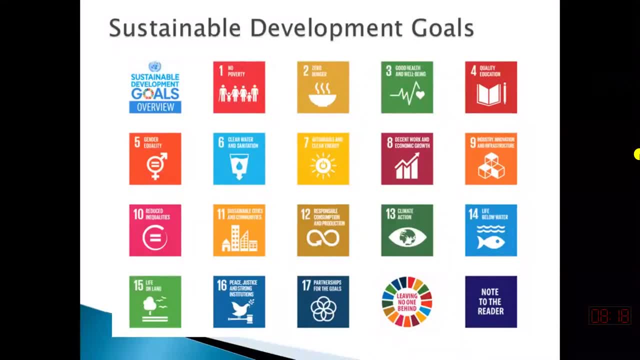 People have also defined it Once in the era of Shaukat Aziz: if he don't get the sufficient number of calories to eat, so they say that he is poor. They used to say that people don't get things in rupees. 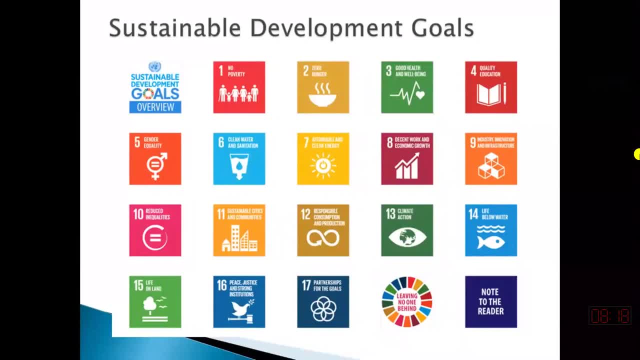 People give food to each other, So they made their definition like this: If he is getting sufficient calories, then he is not poor. If he is getting less than 2500 calories per day or less than 3000 calories per day, 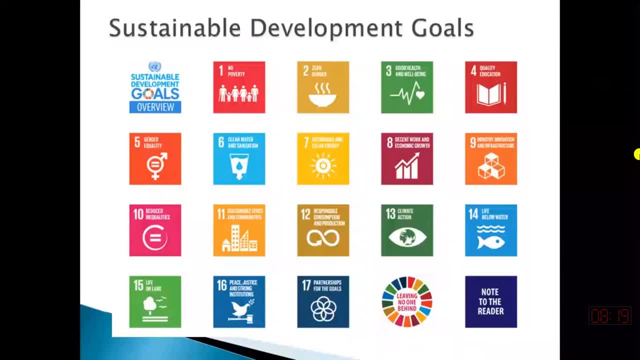 then they consider him poor. But more generic definition, which is considered more, is linked with dollars. If the earning is one dollar per day and the developed countries have more stringent, they say that it is less than two dollars- then he is poor. 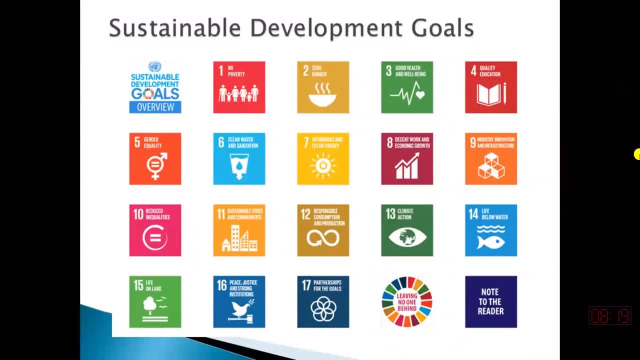 According to this, then they quantify how much population is under poverty. So 30% of Pakistanis say that they are poor. I don't know exactly. You can see how many people are poor. So we were talking about the importance of water. 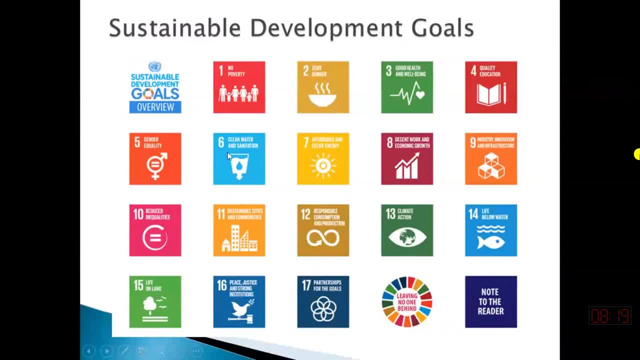 So other development goals are also related to water. So I was asking: can you name any one of them which is related to, which is dependent highly on water? First is poverty. Second is hunger. Third is good health. Fourth is quality education. 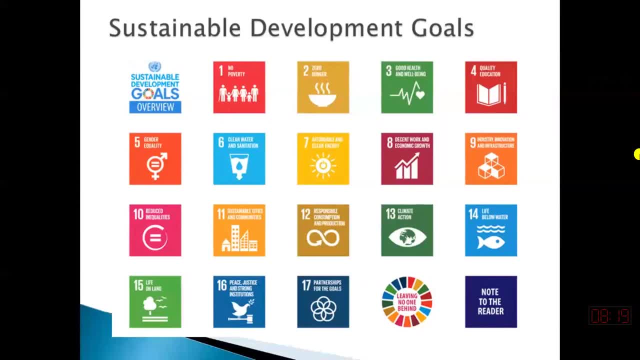 Fifth is gender equality. Seventh is affordable and clean energy. Then what is it? Decent work, economic growth? There are seventeen like this, So can you tell me which one is highly related on water? Dependent on water, Sir. 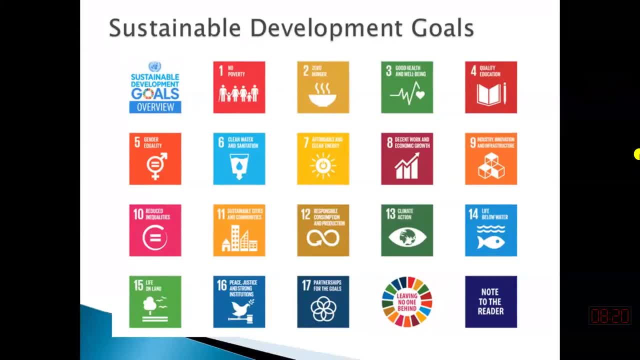 goal number 14 and 15.. The one with clean energy, Fourteen and fifteen, one child is saying. and the one with clean energy, one child is saying. Fourteen is life below water. That is, the natural habitat under water. 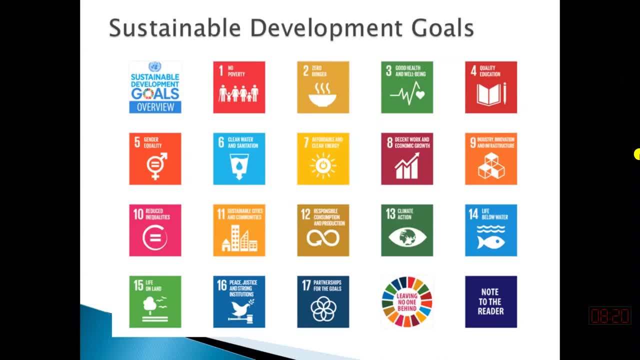 What will we call it Aqua culture? They call it aqua water culture. life there, So life under water, below water. So that is more related to biological species like fisheries, like shrimps, like the food items we try to get from them. 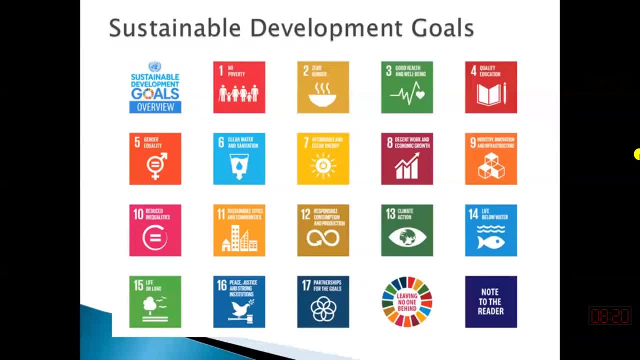 and the variation of that nature. So we can only do this about that water. we have to keep it clean. We should not pollute it. So this is more. our civil engineering concern is to provide water and to drain water. It is not so much linked with that. 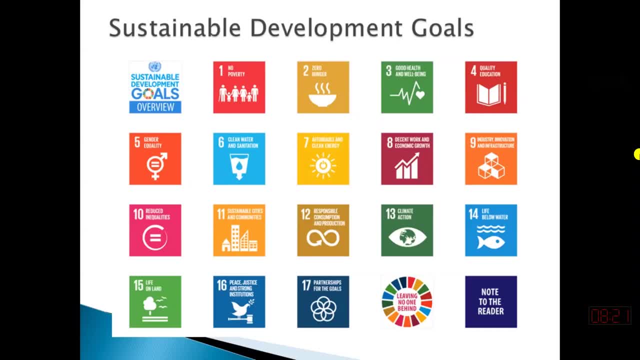 We can reduce it as compared to that Environmentalist who is taking care that pollution does not spread. that is more related to this. Life under water is mostly in oceans. Life under water is mostly in rivers, So in rivers and in oceans. 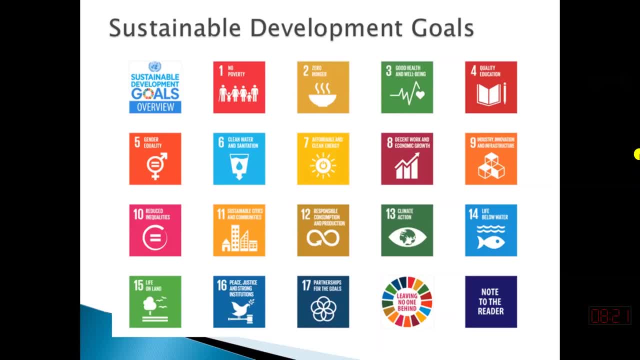 in water. it is related to life, So we can say that if we carry out any development work, it should not be polluting that body of water. So, more related to this. I think this is also related to water, Okay. 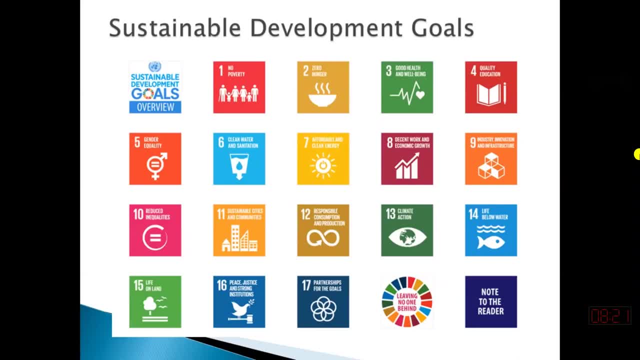 But how much can we interfere in this? We can only protect it according to the environment. Who said seven In clean energy? one of the main source of clean energy is hydropower, So in that sense, our civil engineers and hydrologists. 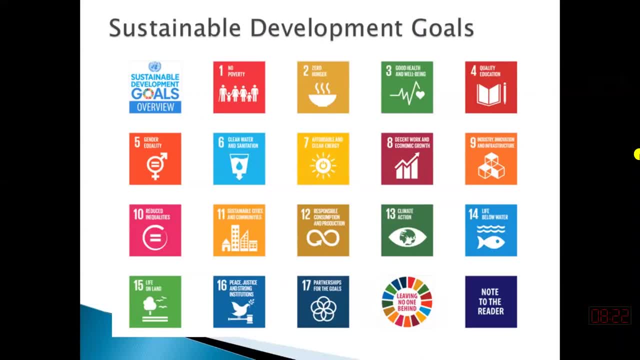 and water resources. a lot of our work is related to the development of hydropower, its planning, So provision of clean and affordable energy. This is totally related to water. Its major chunk is related to water, Although clean and affordable energy. 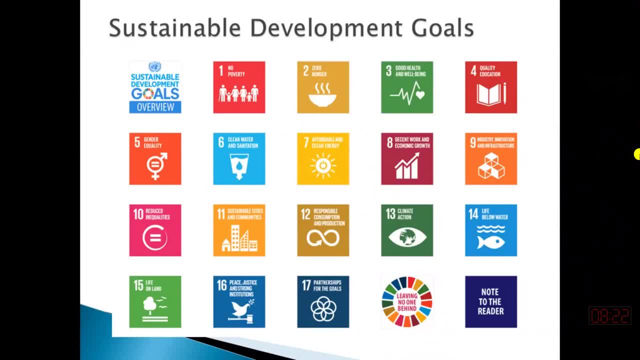 you can also take it from other ways. You can also take it from solar, But maybe that is not yet affordable. You can take it from wind, but that is not still affordable. So the affordable, clean and affordable energy is. a major part is coming from hydropower. 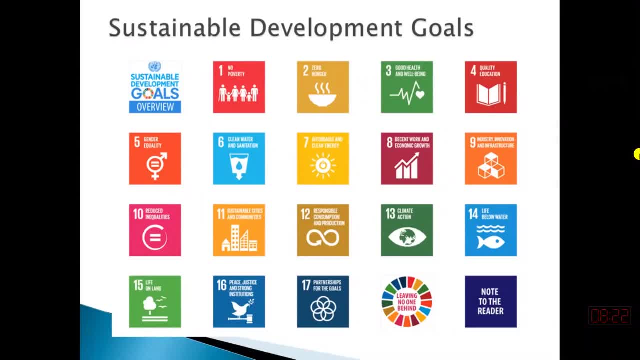 So, according to hydropower, it is highly related to water. Anyone else, Sir, life on land, Fifteen On land, both minutely, minutely, related. More than that, I will say that poverty, zero, hunger, health. 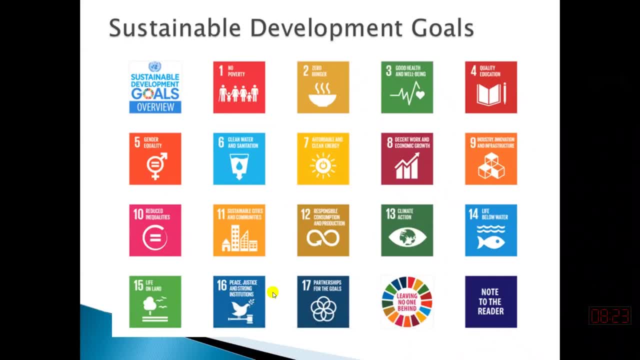 and education are related to water in such a way that the big reason for poverty is that the big reason for poverty is that people do not have good health. The big reason for poverty is that people have a lot, of, a lot of income, which is spent on health issues. 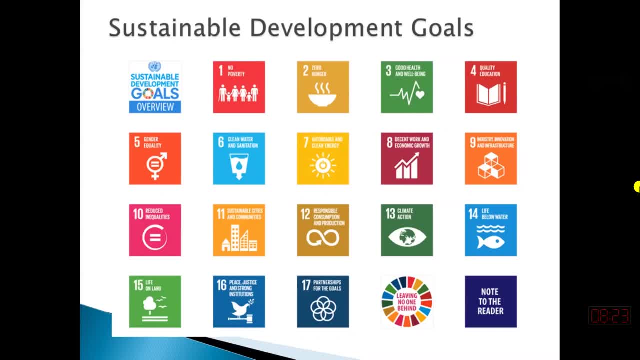 And the big reason for being unhealthy is to drink unhealthy water. The big reason is not having a clean source of water and drinking from a raw source of water and poor sanitation facilities. So what we call water borne diseases is a big reason for our health problems. 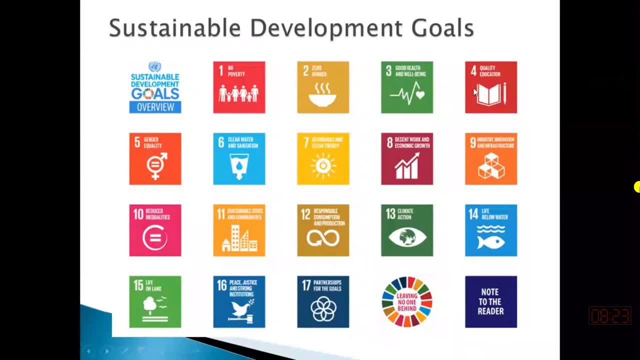 So this? where did this go? health facility: First of all, it is related to water. It is the water expert or water engineer who has to provide clean drinking water and good sanitation facility, which has a direct result that people's health gets better. 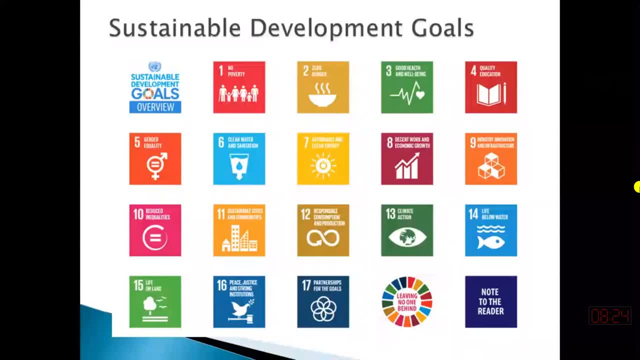 In the area where health is better. even the poverty there will be reduced, Because if a person in a family is unhealthy, then he is a liability He is not earning there. If I am sick for a month a year, then the income of a month will be reduced. 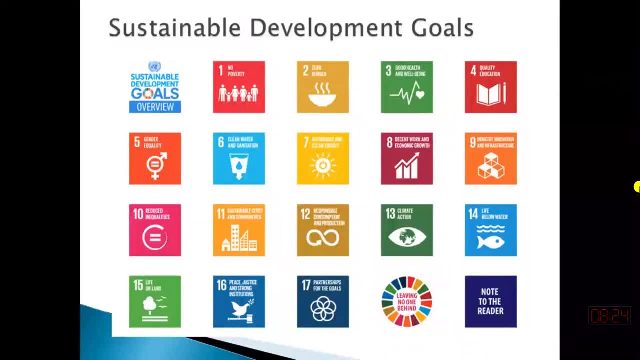 if I am on a daily wage. So in this way most of the population is on a daily wage. So if they stay at home then there is an addition to their poverty. So a big reason for poverty is health. A big reason for being unhealthy is 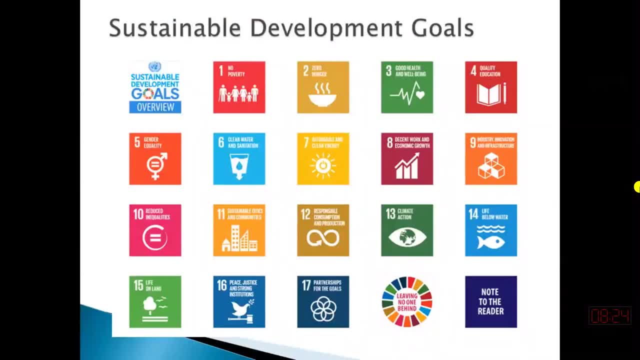 water borne diseases. This is your malaria. This is also a water borne disease. This is your dengue. This is a water borne disease. This is your cholera, which you call Heza Diarrhea. These are stomach diseases. 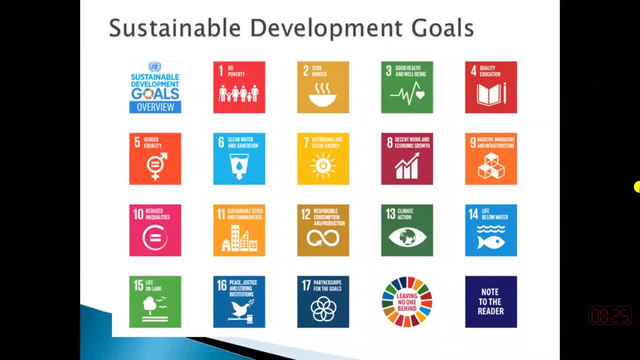 All these bacteria are water borne. So if we improve this, we can improve the poverty condition or the wealth condition. We can reduce the hunger. Poverty leads to hunger. If a person has power, then it leads to hunger. So poverty leads to hunger. 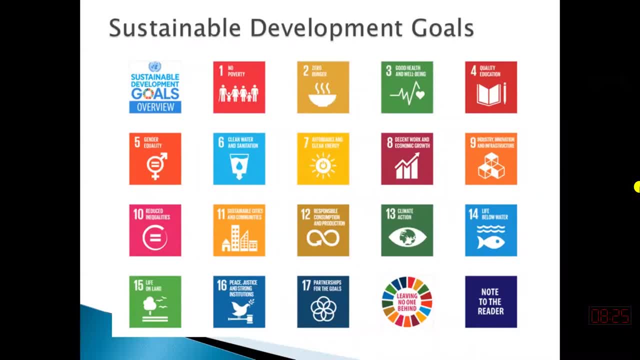 Poverty leads to hunger. And the second relationship of hunger is with our agriculture output. Hunger will not happen at a place where agriculture output is sufficient, Where you get good trees, plants, fisheries, etc. So agriculture is much dependent upon provision of the water facility. 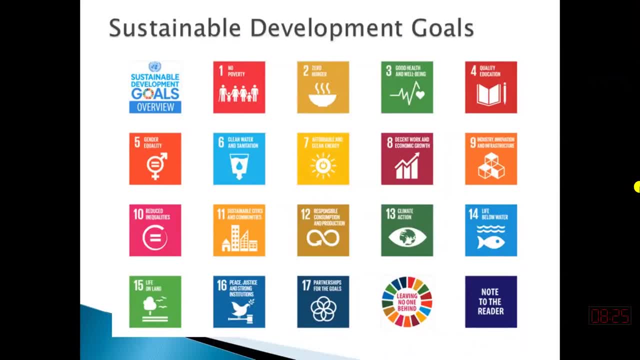 irrigation facility in dry area. Irrigation facility is not required everywhere. Those areas where it rains well, they don't need artificial application of water. Irrigation is an artificial application of water. Those areas where it rains well, they depend upon rain fed agriculture. 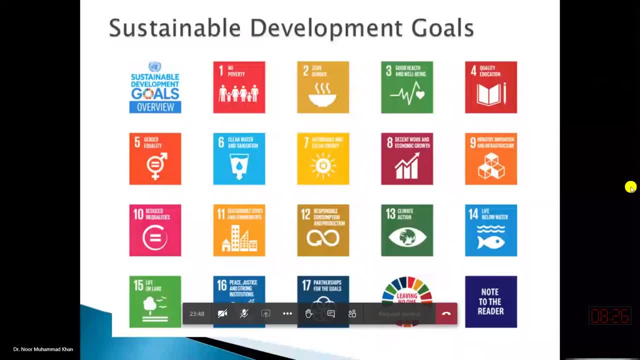 Like the Mariga area, they don't have the canals and channels and barrages for agriculture, But they have good agriculture over there. We will not say that there is no agriculture there. Similarly, the upper hilly area, where it rains well. 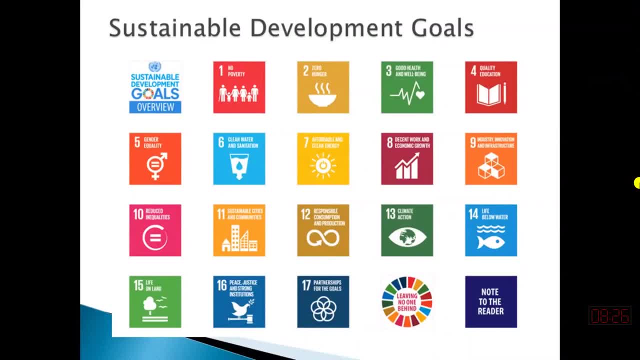 they have good quantity of water through natural precipitation. So the direct relationship of hunger is due to poverty And direct relationship is with the agriculture production of the area. So agriculture is dependent upon water, Poverty is dependent upon water. So we can say that we can reduce hunger. 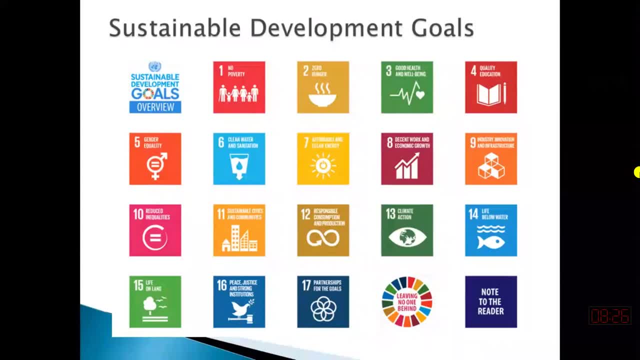 if we invest well in water, Provide good water facilities. So looking at this, the bulk of our development project. similarly, you can relate to others If I say in climate action, water will be very affected by climate, The impacts of climate, 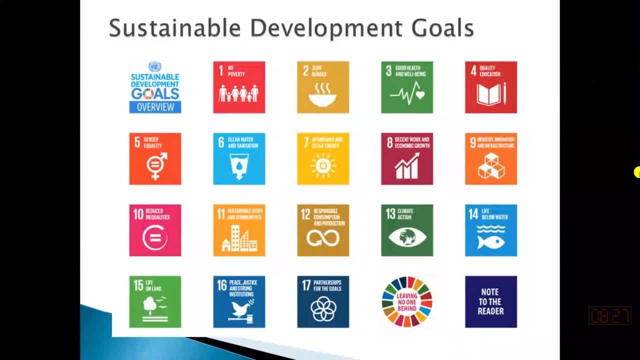 one impact is on hydrology. There are more impacts So in that, in the climate action, the water, people should also be active So that their field, their water, should be least affected And they should be able to provide water to people. 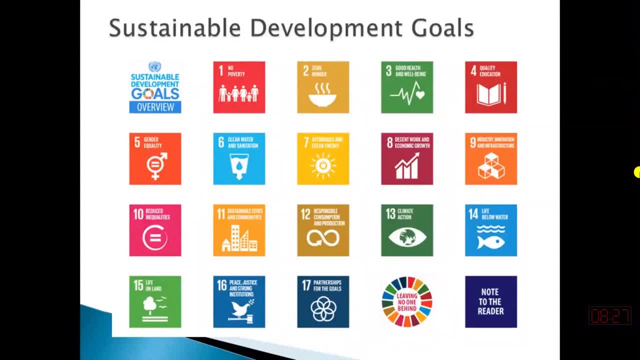 when and wherever it is needed And they can avoid the calamities related to water. They can avoid the destruction or the floods and water related disasters through better management of water and provision of water, Provision of the protection burns and such things. So we have to take climate action. 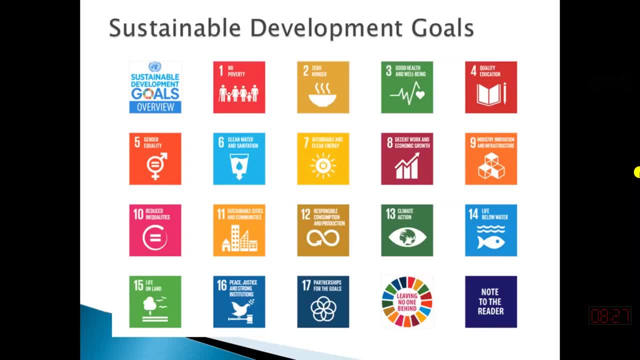 and the water people have to play a lead role in this So that our hydrological sector and water sector should be safe against the bad impacts of climate change. Who else Interact is related to urban. It is very related to civil engineering. 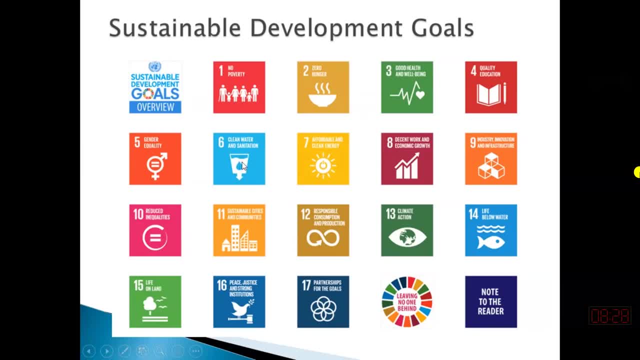 But I will say that water resources are not directly related to it. If you are developing an urban area, then we have to keep it safe against water related disasters too, in addition to other disasters. In this way, many development goals are related to water. 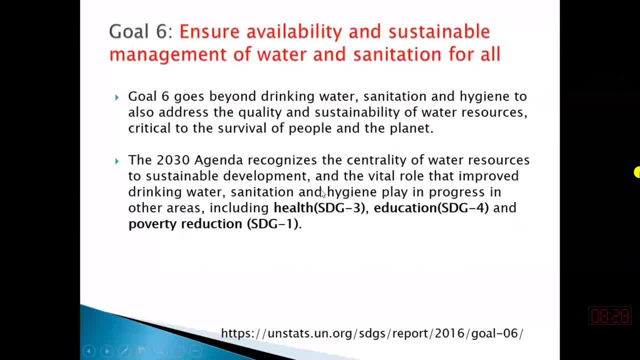 And this is what has been emphasized in the reports of the United Nations. One of them is that water is one of the main agenda of sustainable development goals, And the second thing is other areas, including health, education and poverty. They are much dependent upon. 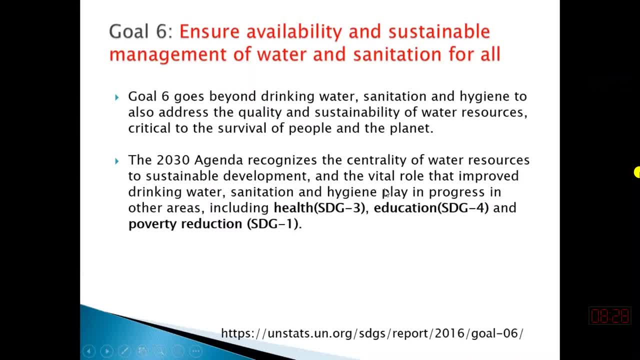 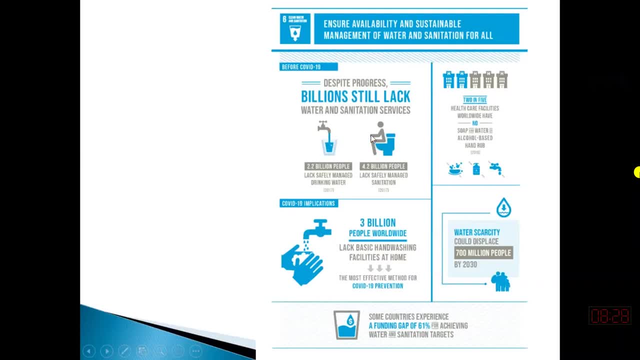 the water resources sector or development of the water resources sector of the area. So this is the message I wanted to give you Yesterday. I saw a recent slide about what is the effect of Corona virus COVID-19 on availability of water and the sanitation facilities. 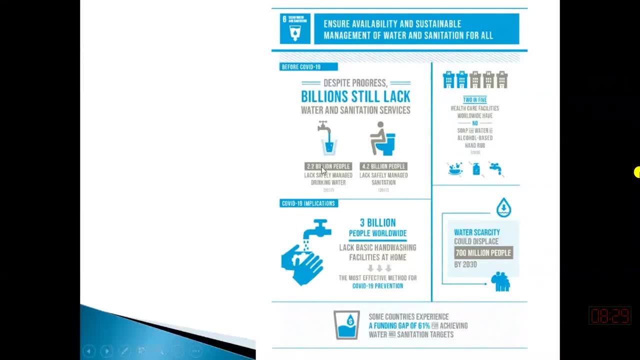 So they saw that before the COVID-19,, 2.2 billion people did not have a safe drinking water facility And 4.2 billion people did not have a facility of sanitation And 4.2 billion people did not have a facility of sanitation. 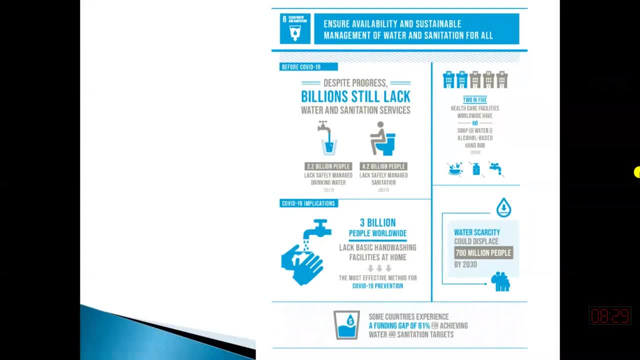 And 4.2 billion people did not have a facility of sanitation Before the COVID-19.. But after COVID-19, what they have found? that about 3 billion people do not have access to safe water so that they can clean their hands. 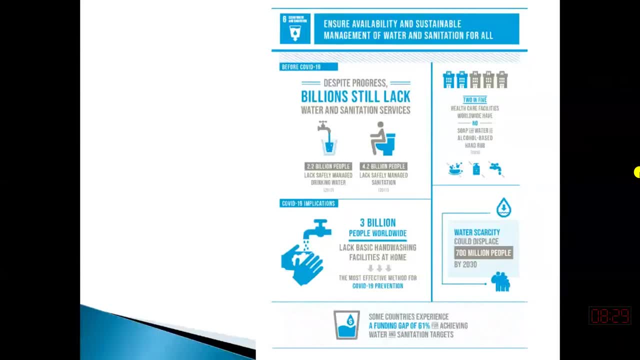 so that they can clean their hands, Because one of the major, one of the major and effective way of mitigating the Corona and effective way of mitigating the Corona, One of the major and effective way of mitigating the COVID-19 is cleaning your hand. 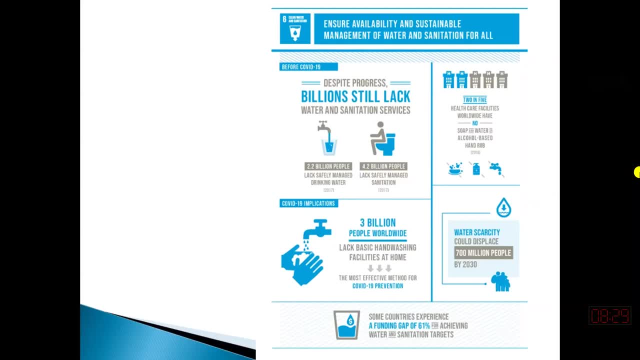 is cleaning your hand for 20 seconds with soap or sanitizer or sanitizer. So if they don't have access to clean water for hand wash- clean water for hand wash- so efforts against Corona will be jeopardized, They will not be successful. 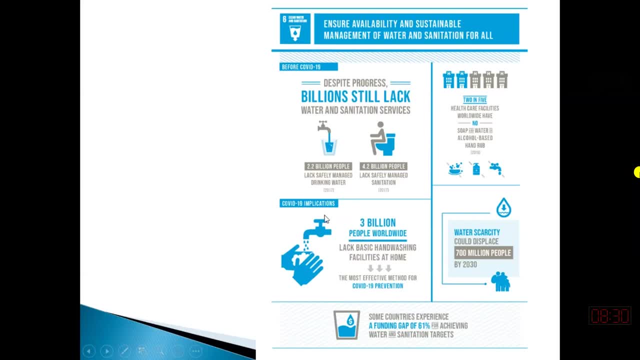 So we estimate that 3 billion people worldwide don't have access and they lack basic hand washing facility at home and they lack basic hand washing facility at home. So there are many houses that don't have this facility that as soon as they come home. 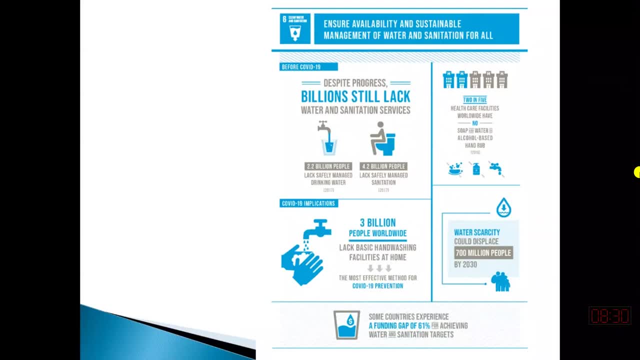 they wash their hands. As soon as there is a doubt that they have been exposed to the Corona virus, they should wash their hands. They don't have this facility. We have to provide this facility as water experts. But the subjects like Hydrology, 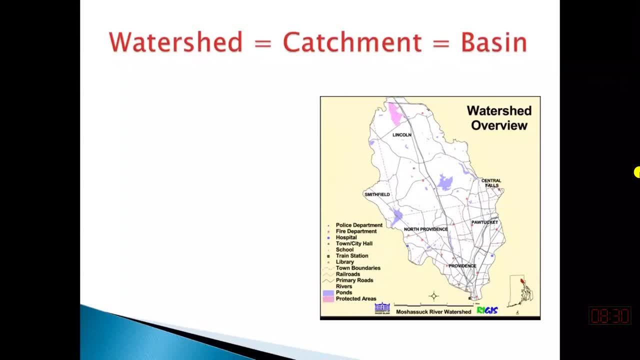 will play an important role. So that was done last time. You were also informed about watershed. Anybody will tell me what is a watershed area. What is it? What is a watershed area? All the area which is contributing to flooding. Repeat it. 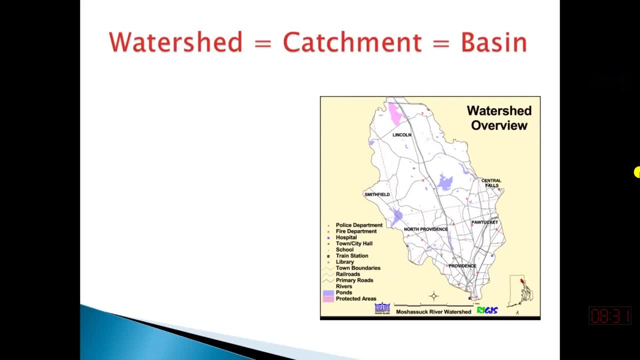 All the area, which is all the area which is contributing in providing water, all the area which is contributing are draining water. at a certain point, definition are, its limits will be changing. so watershed is uh area of land that drains water, uh and other things, sediments and dissolved materials- to a common outlet. so you, you must. 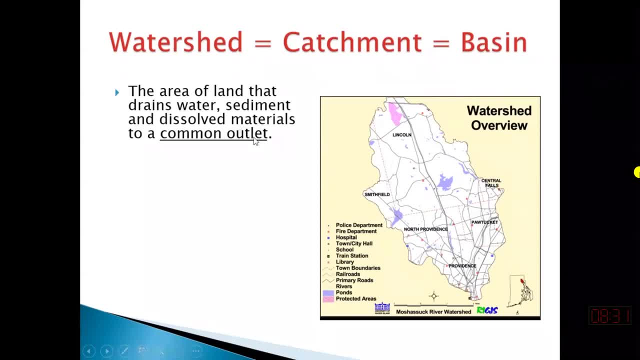 specify that with reference to an outlet, with reference to a point, outlet is nothing but a point which is draining water, for example, uh, along the river, i can take any section and i can say this is the outlet of the upper area and all that area which is contributing water at that point. 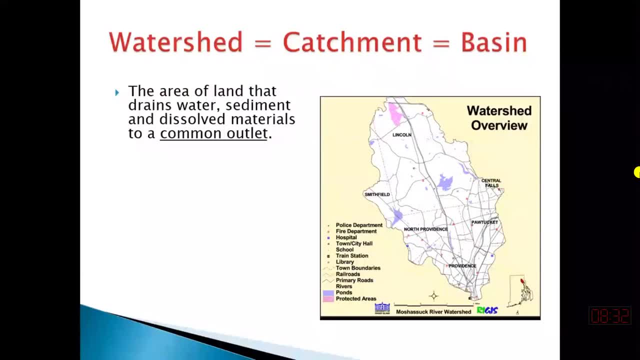 at that outlet. that will be watershed for that outlet. if i move a little bit down, i'll move a little bit up. watershed area will be changed. so watershed area or catchment area is with respect to an outlet. without outlet you cannot define a watershed. so all the area which is draining water are contributing water at a certain point. 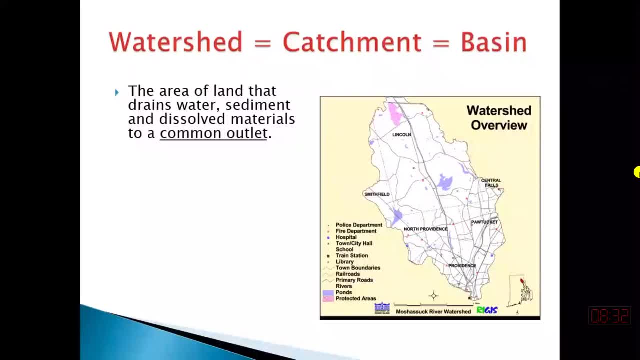 so that will be watershed. they are separated by the watershed boundaries and their size do change from place to place and we mention them in area units. uh, within a watershed we can have many sub watersheds and a big watershed which is draining water to ocean, our permanent water bodies. usually we call that. 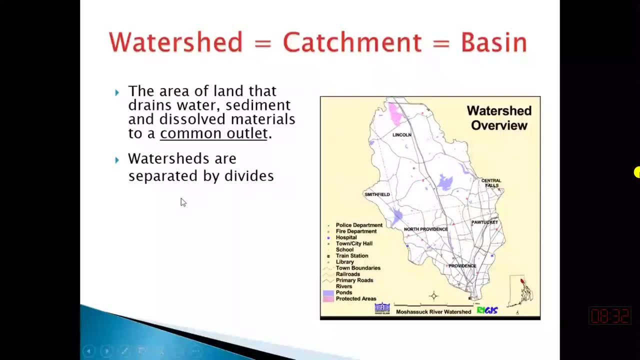 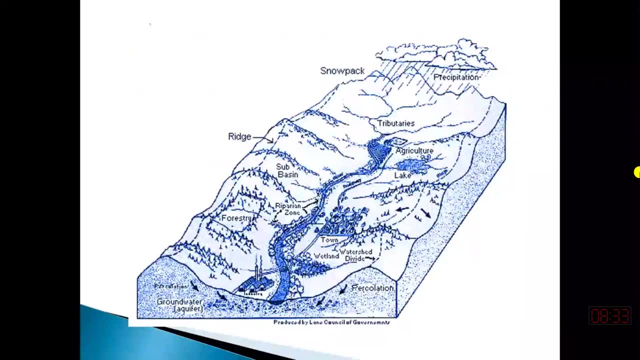 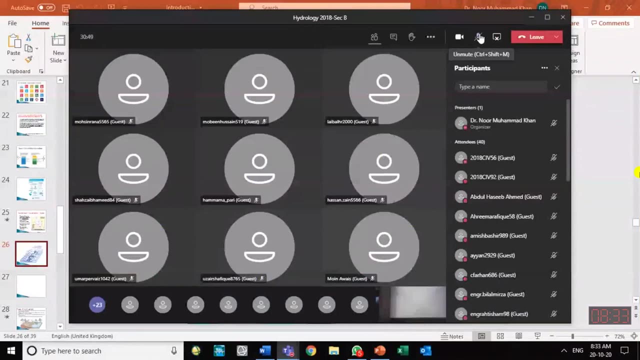 watershed as a basin, a watershed which drains water to a permanent water body. we call that watershed as basin that has the the. okay, please note this difference, that base sun watershed catchment. conceptually they are same. so basically water is drained out. how come does itreto glamorize the surface of the modelS1? 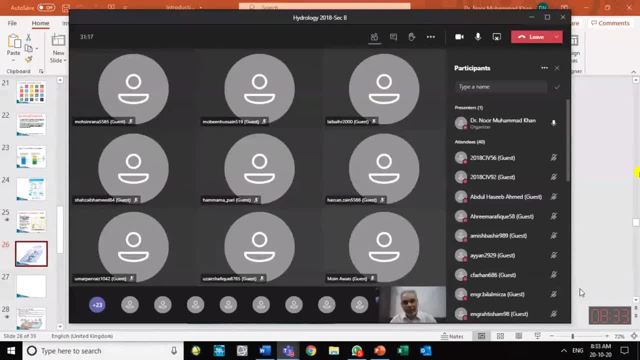 wellness community Beim. so do want to discuss the wash are what agua is done. він basin is that area which is draining water at the outlet, and usually outlet is a permanent body of water, like ocean, while watershed and catchment can be for outlet, which is any place within the catchment. so that's the reason that you 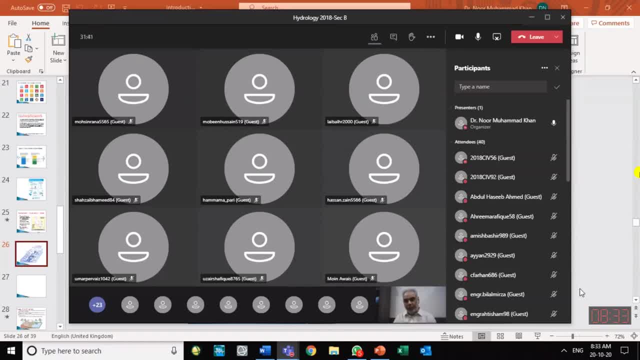 will be listening the words like Indus basin. when we talk about Indus with, we say this is a basin, but you will not hear the word Ravi basin or Satluj basin. so because they are not draining water to a permanent water body like ocean or a reservoir, they are draining water. Satluj, Ravi, Chenab, Kabul, they are draining. 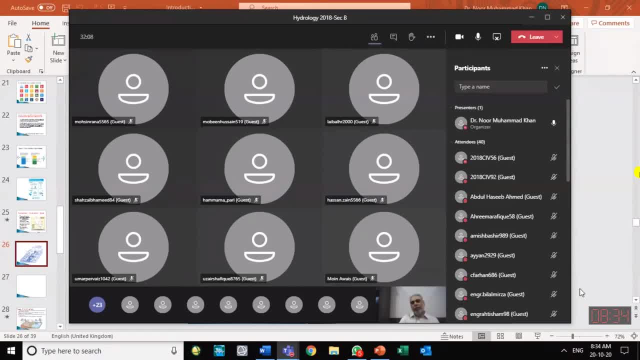 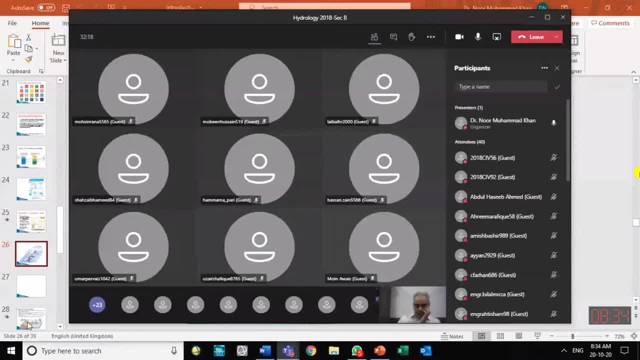 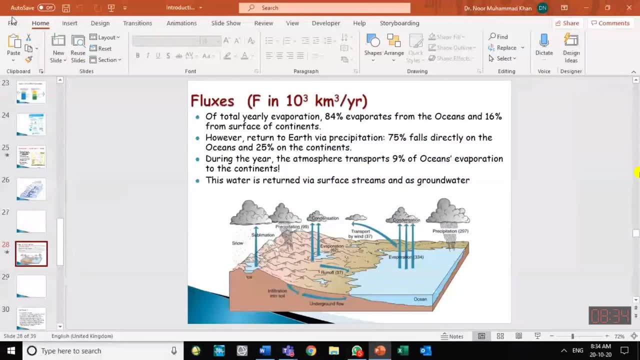 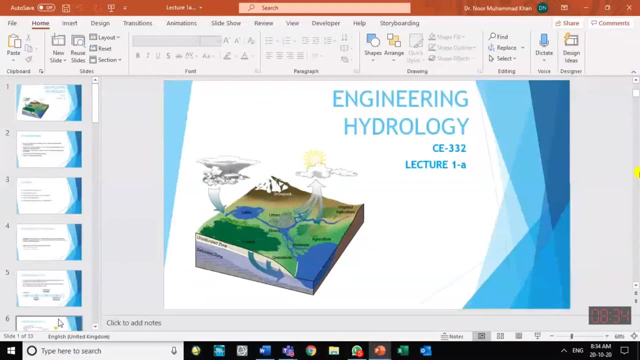 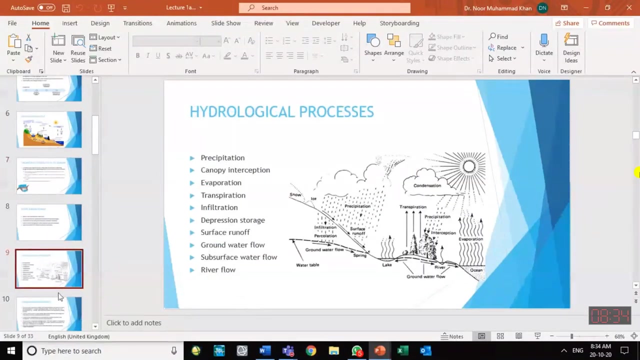 based on the Indus, so after imagineh, when we used in Save a museum, something is connected with water. it will give in conversation with a water jonah, really happy to talk with you about it. but I also would like to talk about about On the topic of marine environment and 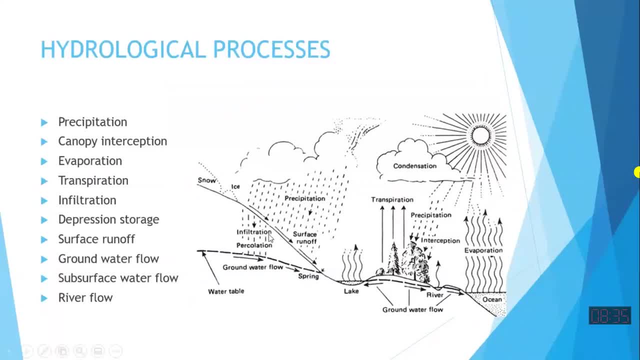 on the topic of marine environment and it creates a whole lot of things which it creates a whole lot of things which flat line vision of the ocean, the flat line vision of the ocean, the charging water to the ocean also. then we have to provide a decent These processes. you have already some of them, you are encountered with some of them, you have already studied and we have to revise them. 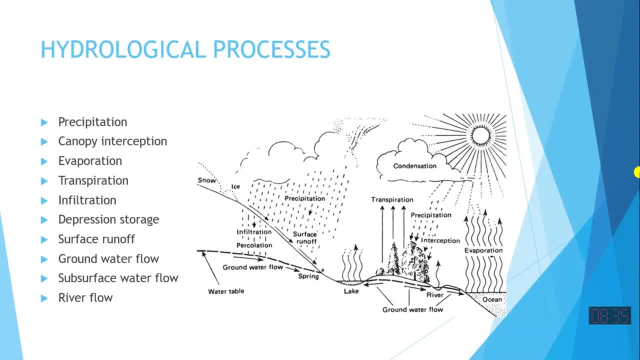 So precipitation, canopy, intersection, evaporation, transpiration, infiltration, depression, storage, surface runoff, groundwater flow, subsurface water flow, river flow. So these are some of the major components or processes within the hydrological cycle. Water which is flowing in the hydrological cycle, water which is moving in the hydrological cycle, will be going through one of these components of hydrological cycle or one of the storages of the hydrological cycle. 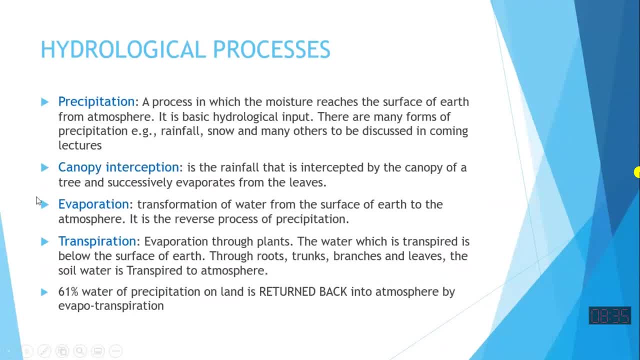 If we see this component one by one, precipitation is the process in which moisture reaches the surface of earth from atmosphere. When water comes from the atmosphere to the surface of earth, we say this is precipitation. So it includes rainfall, it includes snow, it includes hailstorm and other ways of movement of water from the atmosphere. 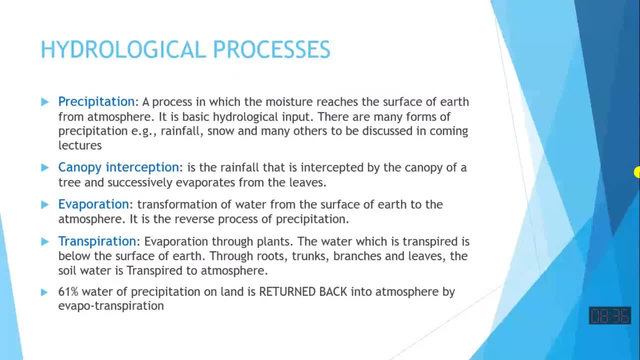 So this is a major input to the surface water of the ground, of the earth. Inverse to this precipitation, reverse to this, is evaporation. This is the third one: Transformation of water from the surface of the earth to the atmosphere. So precipitation comes to the earth because of the gravity force. 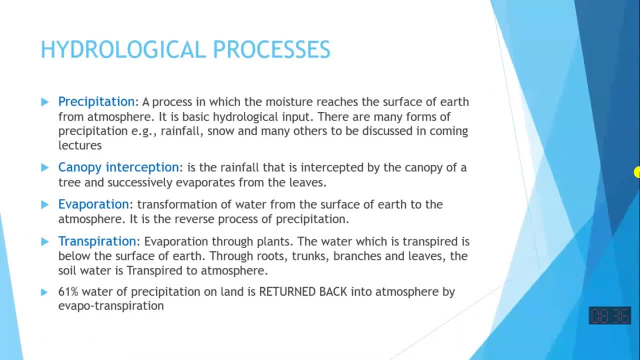 Evaporation goes to the atmosphere because of solar energy, and because of the solar energy, sufficient energy is available and the molecules of the water are changed from liquid phase to the vapor phase. And then they because of their low density, And then they because of their low density. 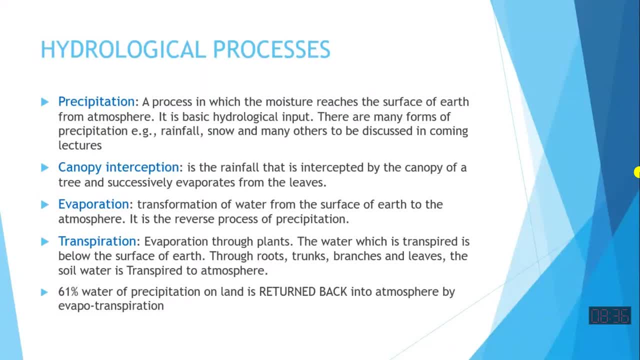 Because of their buoyancy they move upward. So evaporation is transformation of the water from the surface of the earth or surface of earth. Water surface is bio-septane- Earth contains land and water bodies- So from the surface of earth. if water moves above to earth's atmosphere in the form of the vapors, we say this is evaporation. 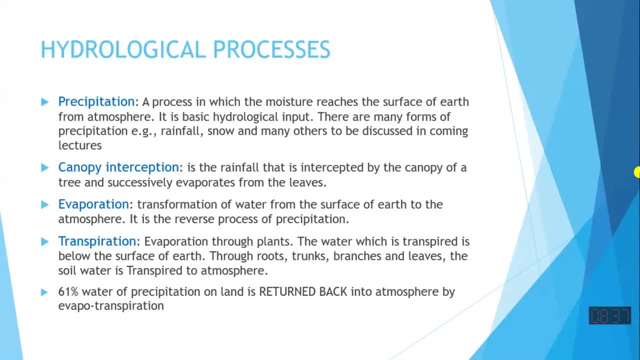 Okay. other processes are canopies. Other processes are canopy interception. Canopy is the cover of vegetation on the earth. If you look at the earth from the satellite, wherever there is vegetation, you will see that you will not be able to see the bare land. 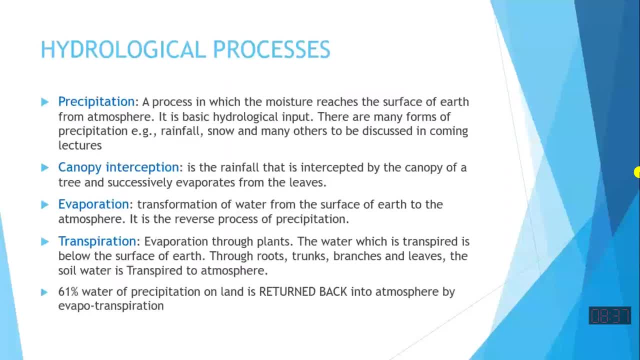 So you will see, there is a canopy like thing. You must have seen a canopy in Shamia, or a tent, or you must have seen an umbrella. So these trees, leaves are working as a canopy for the ground. So when precipitation occurs, not all precipitation water or rain water reaches to the ground, reaches to the earth immediately. 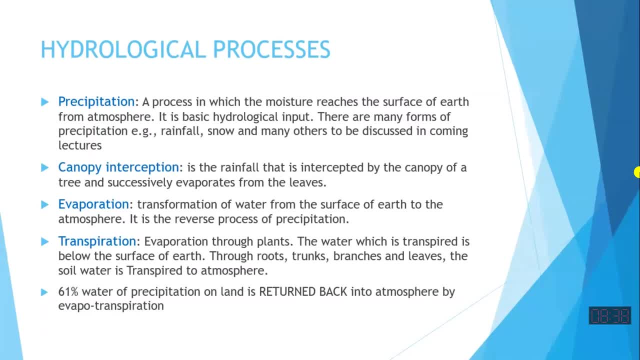 Some of that is intercepted or stopped by the canopy of the trees and vegetation, So that part of the water which is held by the vegetation cover, so that we call as a canopy interception That quantity of water. we call as canopy interception, It's the rainfall that is intercepted, which is not reaching to the ground. 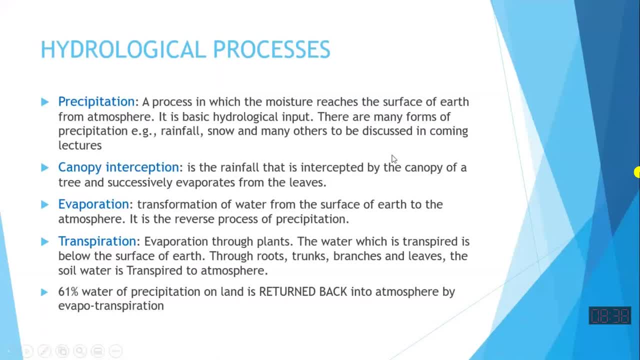 It is that part of the rainfall that is intercepted by the canopy- And now you know, canopy means canopy of trees, canopy of vegetation. So that part of the rainfall that is intercepted by the canopy of the trees and vegetation, And later on, successively, later on, either it evaporates back to the atmosphere or it drips down to the ground. 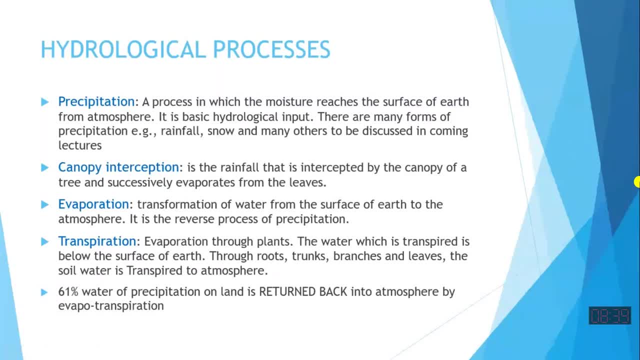 The bulk of it goes back to the atmosphere through evaporation. A leaf has intercepted some droplets of water, So either it will come down or it will go up. So canopy interception has two phases. Either it will evaporate back or it will drip down. 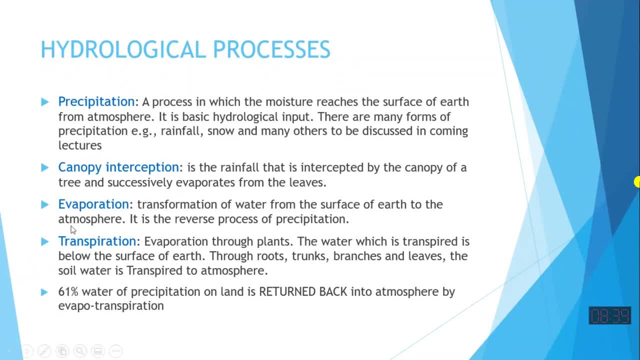 So transpiration is similar to evaporation. I think I told you earlier also It is the evaporation through plants, leaves Through plants, the evaporation of the. so that is called as transpiration. It is estimated and you have seen in the hydrological cycle figure also. 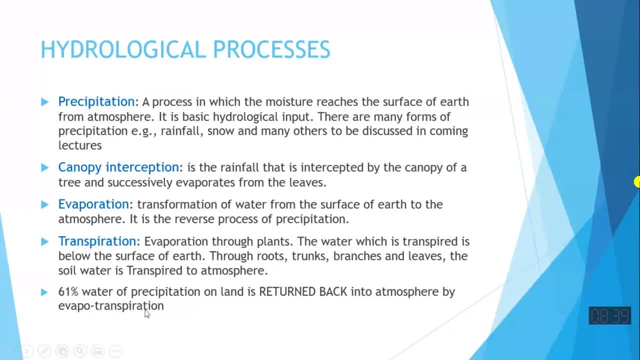 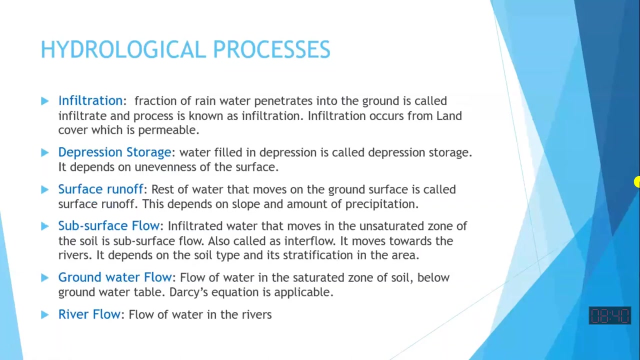 That out of the total rainfall on the ground, on the land, Out of the total land precipitation on the land, 61 parts goes up in evapotranspiration. So that is combination of evaporation and transpiration. So infiltration is that component of the water which comes to the ground. 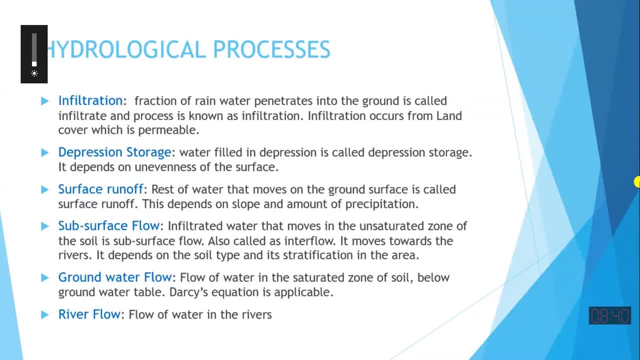 And then it seeps into the earth. Fraction of the rainwater that penetrates into the ground is called infiltration. That is one of the main source of inflow to the ground water Ground water reservoir which we have seen that 0.68% of the total earth water is ground water. 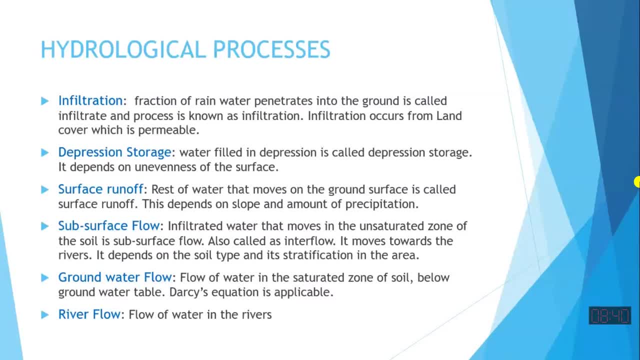 Which was about 9500 thousand kilometer cube. Today we have seen in the table So 9500.. So the bulk source of that ground water is because of the infiltration of the water from the ground surface. So if all the earth was impermeable, 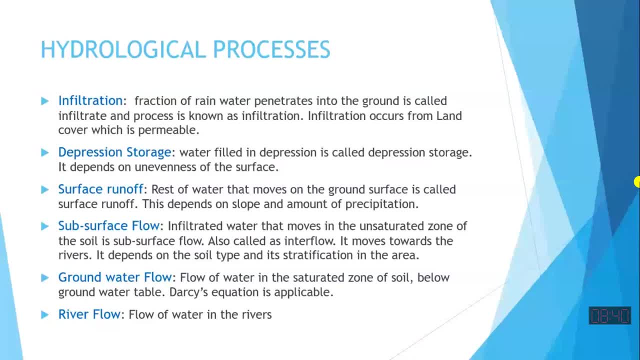 Then ground water body would have gone. This would have vanished away. So it is the impermeability of the soil which allows water to penetrate into, And then it is stored in the underneath storage of water, which we call as the ground water storage. 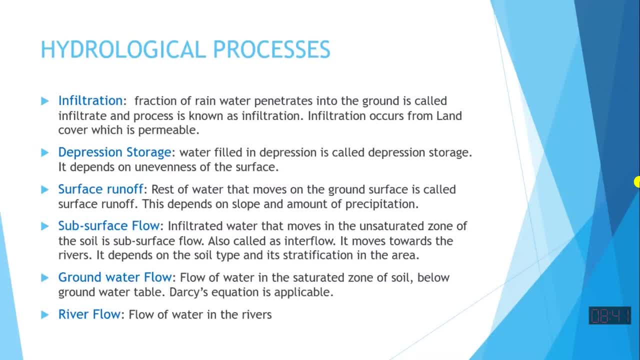 So infiltration is fraction of the rainwater that penetrates into the ground. It infiltrates And the process is known as infiltration, And the water which goes is infiltrate water. If it is permeable, then infiltration occurs. So from here another study starts. 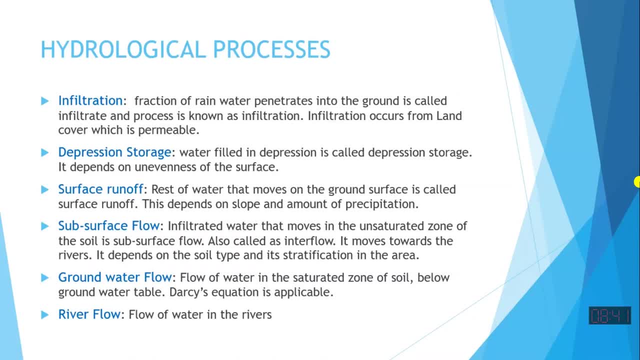 If we change land cover, If we change land cover. Land cover means what is covering the land. Sometimes land is covered by the crops, Sometimes land is covered by forest, Sometimes land is covered by bare soil, Sometimes land is covered by roads. 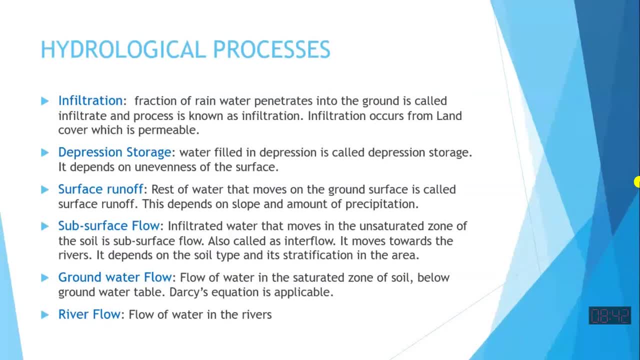 And sometimes houses. So if we change the land cover From natural land cover to artificial land cover, Then infiltration change, Then ground water resources change, Then water available on the surface change, And such studies are. now we are doing it for different catchments of Pakistan and other areas. 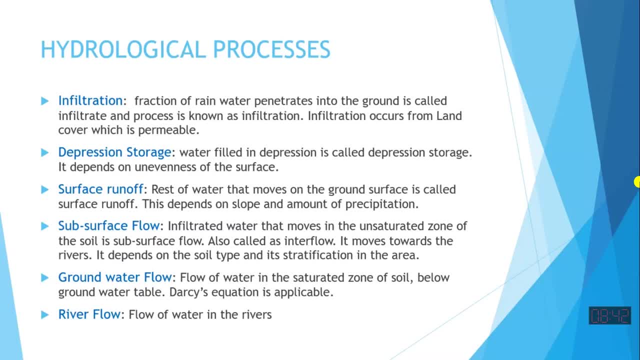 Effect of land use change on availability of surface water in Rawal Dam catchment. Effect of land use change in Khanpur Dam catchment: Those reservoirs and dams which are built specifically for agriculture purposes. For those, if we have chances that the availability of water will effect because of the land use change. 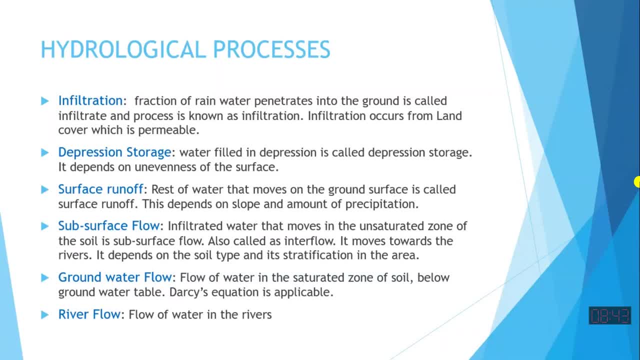 Then such study we carry out as master study or as consultation studies. So few master study you can see carrying out this factor. If land cover change, What will be the effect on the ground water? What will be the effect on the surface water? 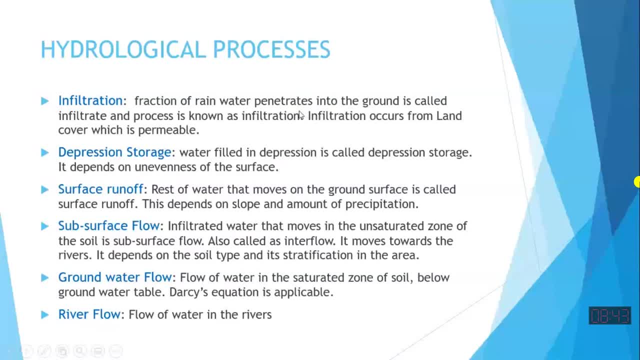 How we can mitigate it. But you should be knowing at this moment that If you change the land cover from, for example, bare land to the crop land, Infiltration will change. If you change it from crop land to forest, Infiltration will change. 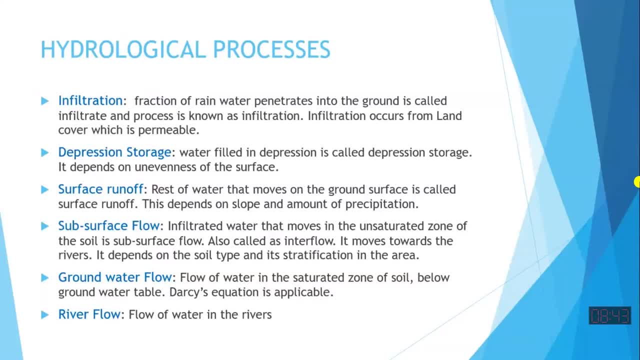 If you change it from these three to urban area, Infiltration will change And if there is more urbanization, Infiltration reduce. surface water increase Out of the total precipitation. water Infiltration reduce if you change from the natural cover to impermeable covers like roads and a building. 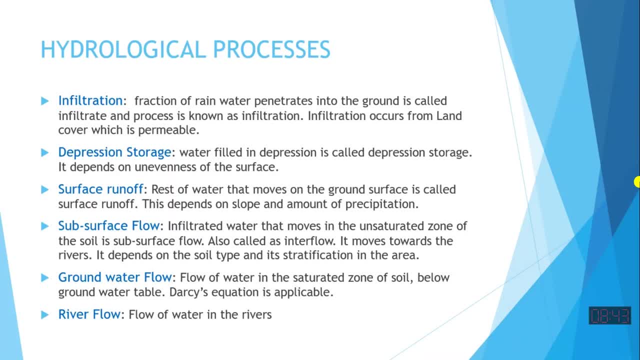 Then infiltration reduce and then surface water enhance And more floods and more flows will be seen over there And you will be seeing the ground water table is going down, down, down. Reduction in ground water table will be happening over there. So such studies we people are carrying on. 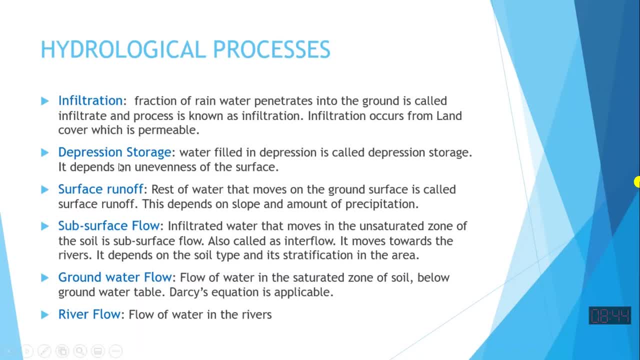 Through our research study, Depression storage When water occurs. So our topography, our natural land surface levels are not smooth. At some places there are hills And at some places we have depressions. The depression area becomes natural lakes, Natural bonds, natural lakes. 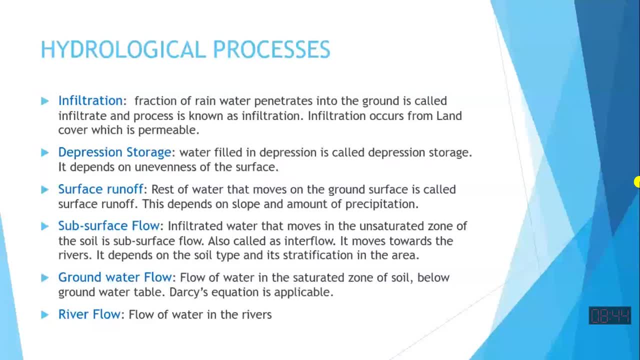 So some water is stored in these depressions, Depressions, Depressed area, And we say the reservoir or natural lake or bond has been formed over there. So that should be also accounted for when you are accounting the all aspect of water in the hydrological cycle. 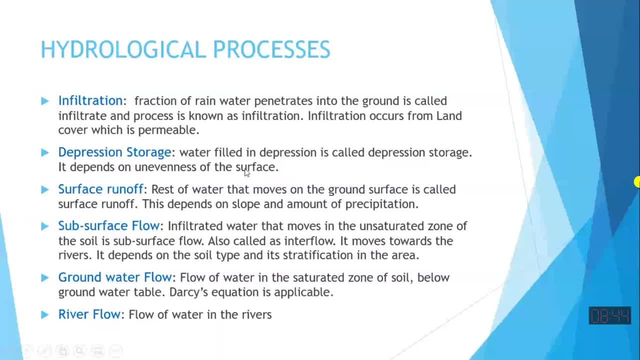 Depression storage is one of the water storage which is not reaching to the river immediately. For example, if you are carrying a water budget estimation And you say that 100 mm of the rainfall occurred In a certain area, So you will be trying to see where that 100 mm of rainfall is going. 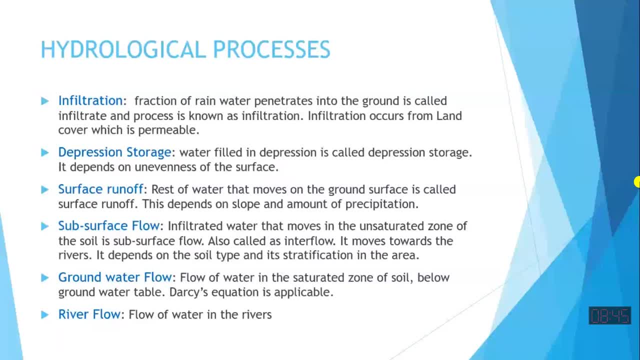 So when you will see that river gets so much water, Ground water gets so much water, There may be some leftover water which you are not seeing where it goes, So it can be depression storage, Which is holding water in its storage for some time. 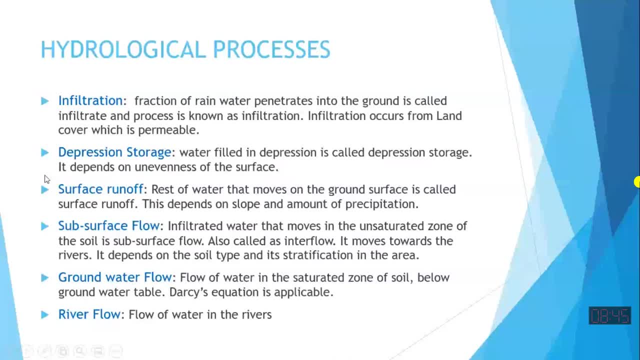 And then that water is going into ground in the later stage And evaporating to the atmosphere In the later stage. So depression storage is an important factor in hydrological cycle. So when infiltration have been done, Some part goes to infiltration, Some part goes to depression. 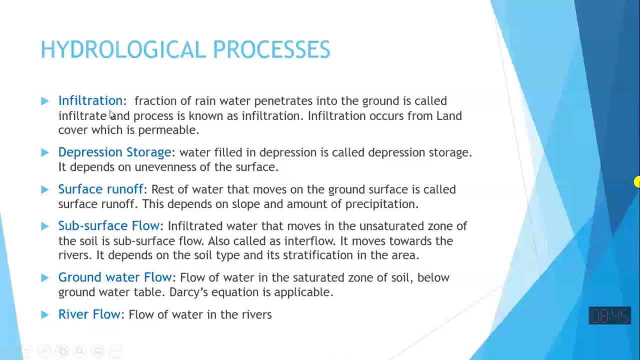 Some part is evaporated back, Then excess water starts flowing on the ground. So we say that excess water is the surface water, Surface runoff, Runoff, Surface runoff: Rest of the water that moves on the ground surface. We call that as surface runoff. 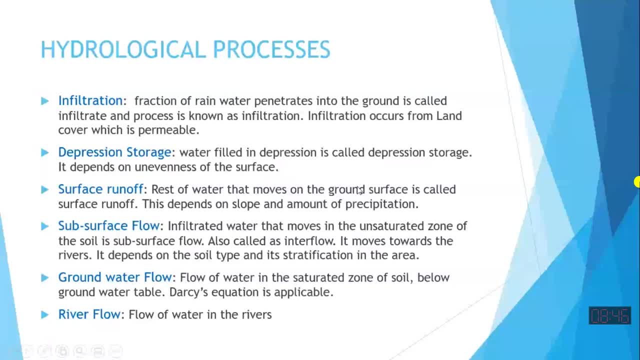 And how much will be the speed of that surface runoff? How much will be the quantity? that depends upon the type of the surface: If it is impermeable, If it is porous. It depends upon slope of the surface, If it is steep slope. 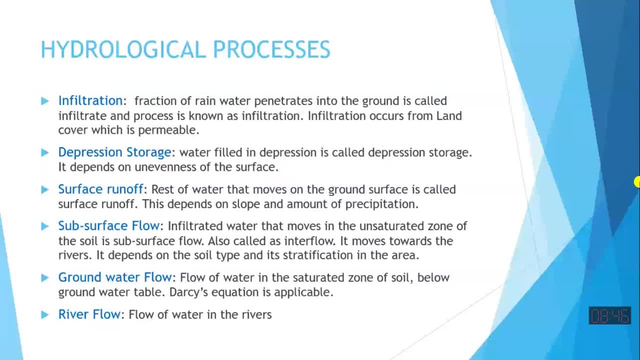 Runoff will be high speed. It will be going out of that area immediately. If it is mild slope, Small slope, Then it will be moving out slowly. So surface water, Surface runoff occurs And also the surface flow occurs. The infiltrated water goes to the soil. 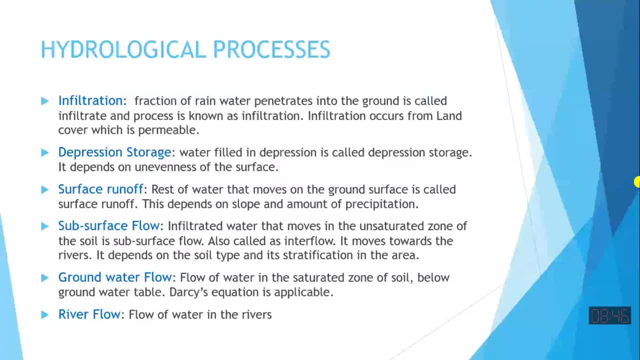 And it joins the ground water. So some part remains as moisture in the upper part of the soil, And that part of the soil is usually not saturated, And some part reaches to the lower layers of the soil, Which is considered as saturated. 100% of the pores are filled with the water. 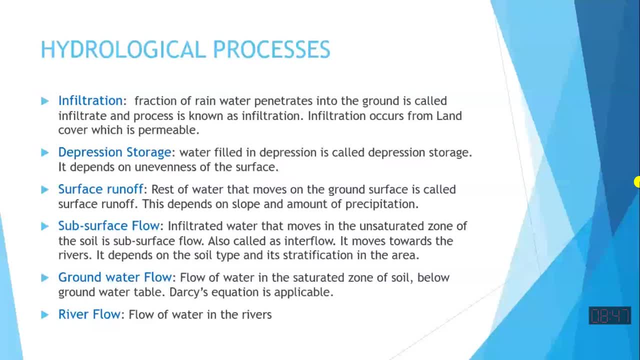 So that part Which is 100% saturated, We say this is the ground water, This is the ground, Although all the water is under the ground, But we have divided it into two components. If you see the picture In this picture you see: 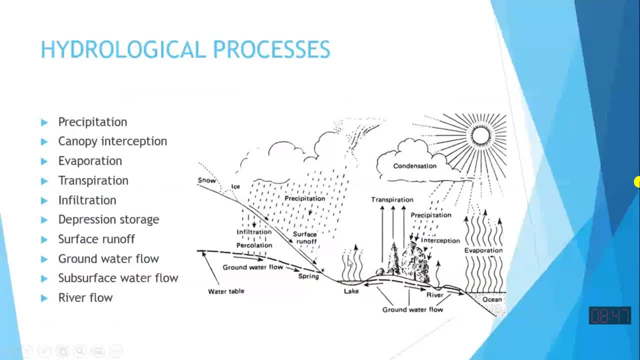 This is the surface of the ground. Hopefully you are seeing the mouse. If this is the surface of the ground, Water infiltrates. So all this underground layers Can be divided into two major layers. One is that component of the soil Which is 100% saturated. 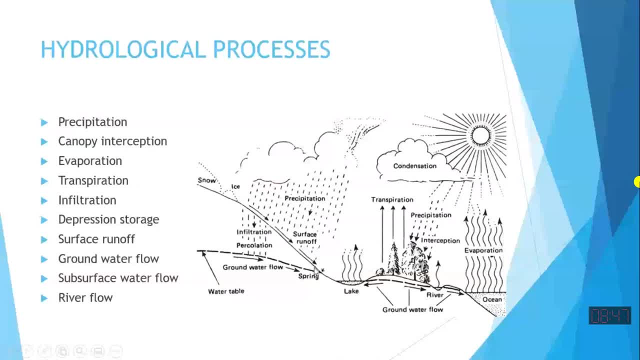 And that is named as ground water, While the upper part of the soil, Which has the soil water, But it is not 100% saturated, So it is partially saturated. We call this part as surface moisture, Sub surface moisture, We call this moisture and this water. 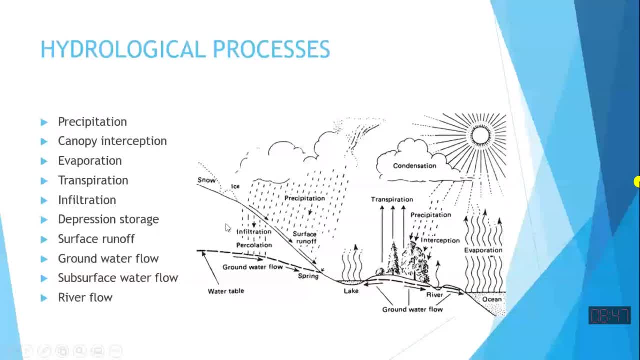 As the sub surface moisture. So this is the surface of the ground And this water is the sub surface moisture. Water flows from both parts. Sub surface moisture also flows In the direction of the gravity And the ground water also flows In the direction of the gravity. 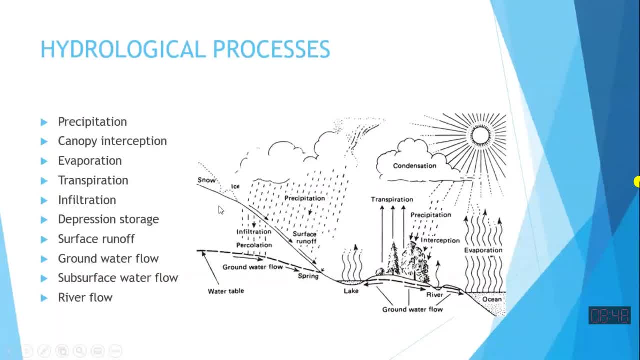 Understand, Water in the soil Moves vertically downward also. It moves horizontally also In the direction of the gravity, So that two things are called as Sub surface flow And the ground water flow. So that should be distinguished From each other. 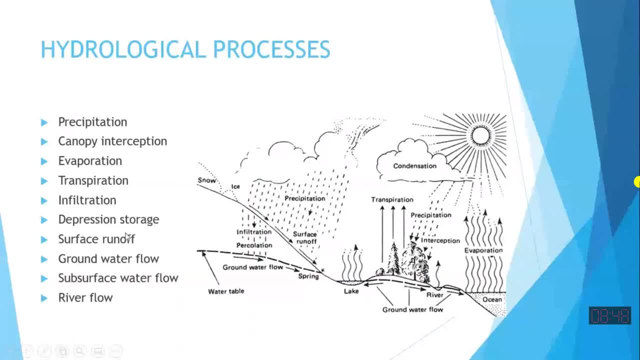 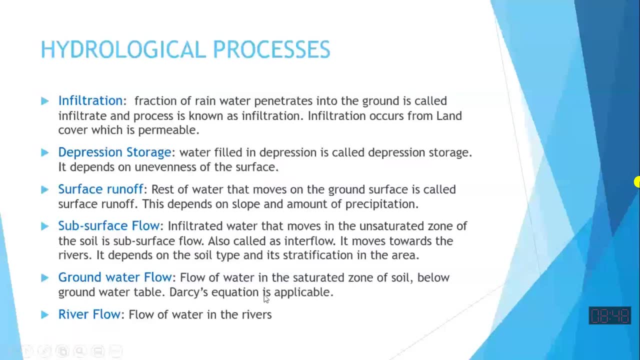 One is sub surface flow, That is, the flow of water In the unsaturated zone. One is the ground water flow, That is the flow of moisture In the saturated part of the ground. Flow of water in the saturated zone of the soil. 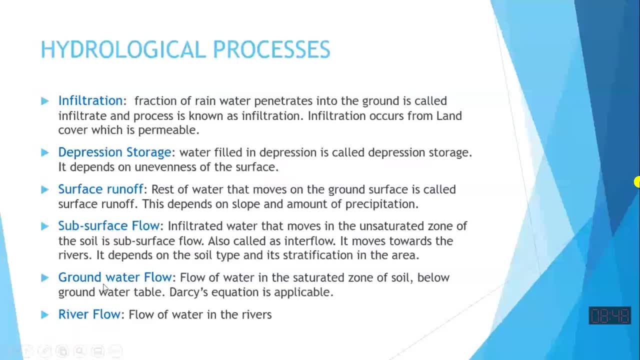 Is called as ground water flow, While flow of the water In the unsaturated zone of the soil Under the ground Is called as sub surface flow. Sometime we call this sub surface flow As inter flow, The flow between the ground. 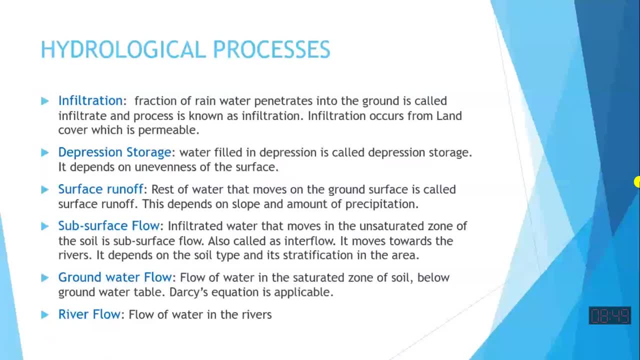 And between the ground water, Inter flow, Intermediate flow Or inter flow. It moves towards the river, It moves towards the gravity, And usually rivers are Towards the direction of the gravity. So how much will be the flow quantity, How much will be the speed of this flow? 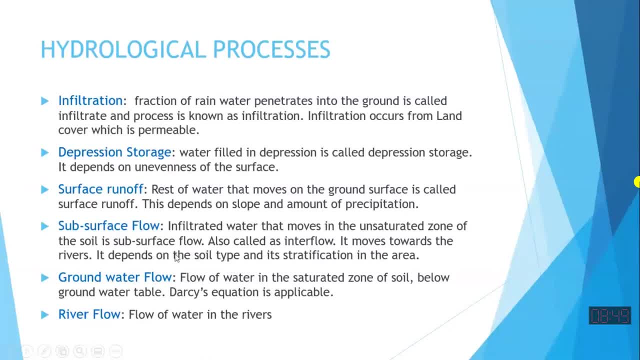 It depends upon the soil type, It depends upon the head available For movement For ground water flow. We use Darcy equation: Q is equal to C, I A, C, I, C is R, K, I A. K is the permeability coefficient. 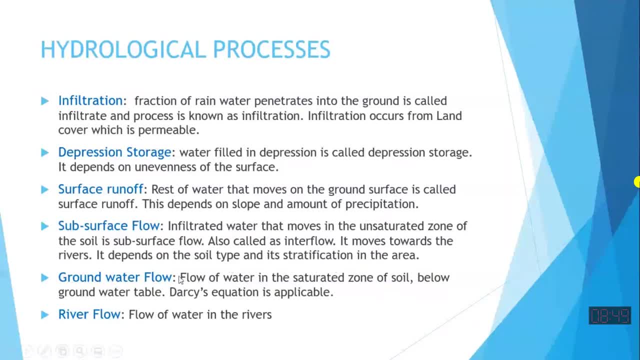 I is the hydraulic gradient. A is the flow area. It will be informed to you When we will be studying the ground water flow In more detail, And then surface runoff When it is combined together And make a form of a channel. 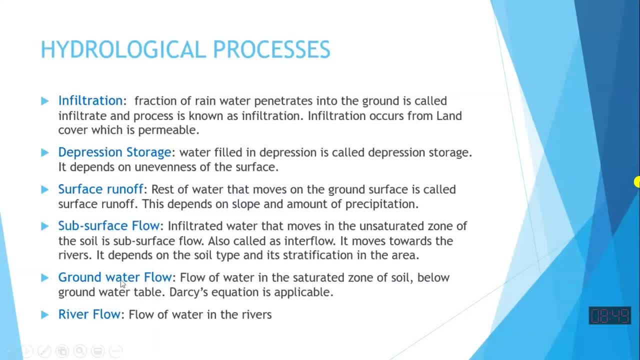 So then Surface runoff, That will be called as river flow When the surface runoff Becomes of so much depth That we can measure it. So then we say: now it has become the shape In the form of the channel. So then we say: this is a channel flow. 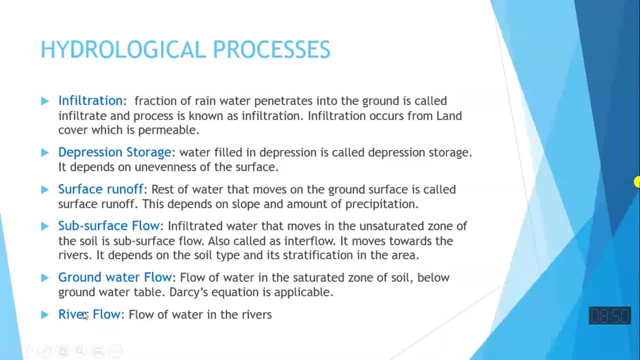 Or river flow. So This is also surface flow, But we distinguish it from Surface runoff. Surface runoff we consider as a thin sheets flow, While the river flow. So it is a river flow Which we stop In the reservoir or dam. 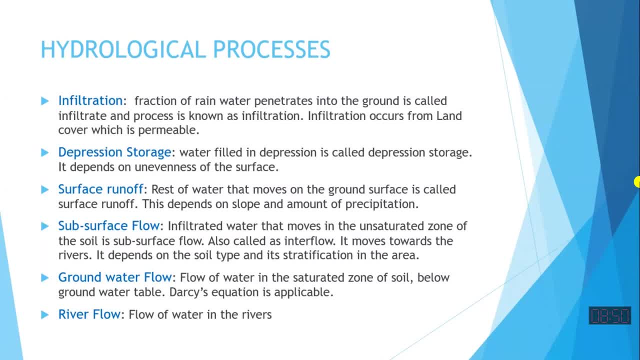 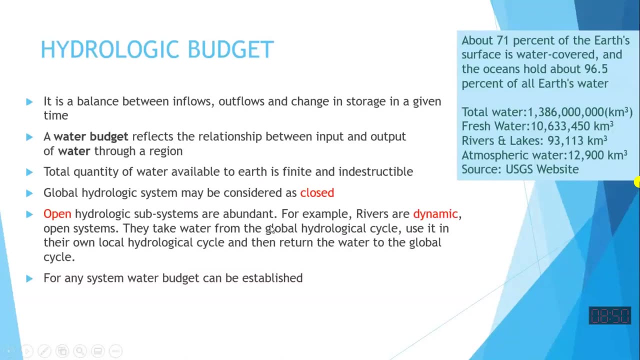 And then we divert it In the canals And then we use it for Beneficial purpose. So As a hydrologist We are assigned usually duty To budget this water, See how much water is available In what part of. 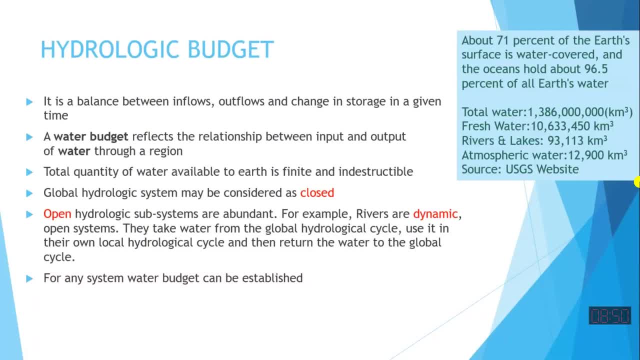 Hydrology, The cycle. So some budget Figures are Repeated over here. For example, if the total water is 1.38 billion km3.. Fresh water is only 10 million km3.. River water is Even less. 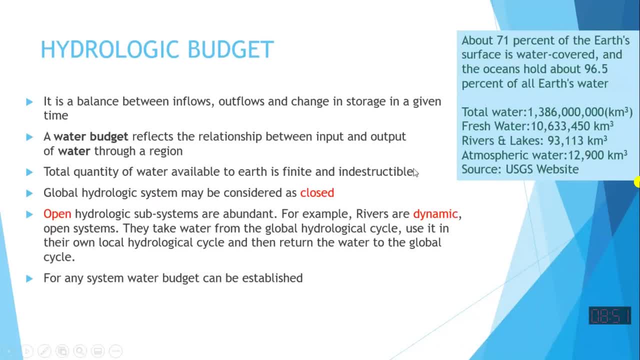 93,000 km3. So Although it is 71% Of the total surface of the earth. But fresh water resources Are quite limited, So Quite often We have to budget this water, And we should know what is a budget. 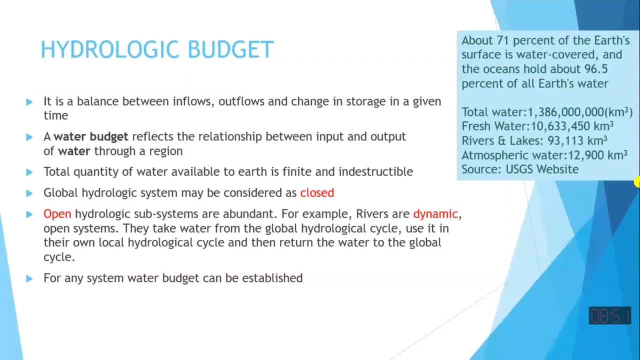 Budget is In general terms. Budget is the statement of income and expenses In general terms. In general terms, In economic terms, When we say budget Income and expenses statement, We have university budget In the board or in this sheet. 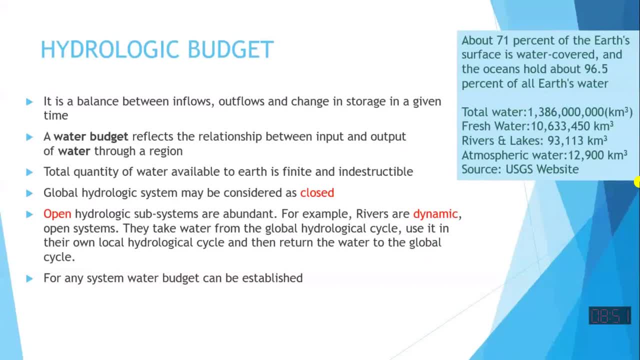 They will be telling How much is the income of the university, How much is the expenses of the university? What are the balance? Balance can be plus, Balance can be negative. When there is negative balance Means we have to borrow from somewhere. 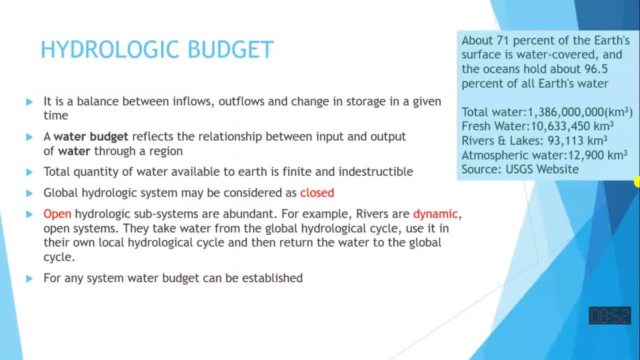 So similarly we have budget of Pakistan, But in hydrology Budget means Statement of inflows and outflows And the net availability of the water. Statement of inflow and outflows Part of hydrological cycle Or for the whole hydrological cycle. 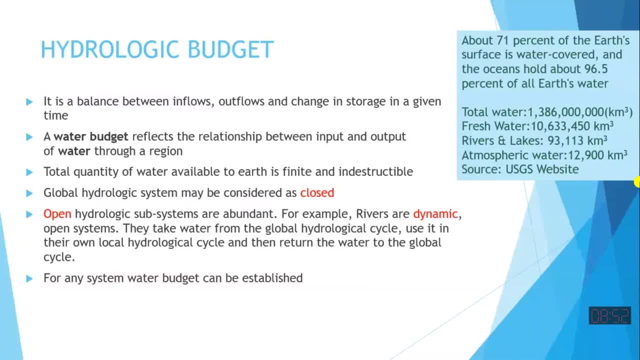 So budget Reflects the relationship Between input and output of water For a region For a part of hydrological cycle And Why we have to do it, Why we have to make a budget, Why we have to Estimate these values. 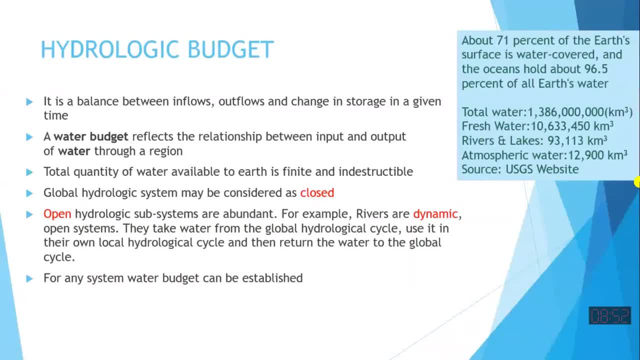 Any answer for that? Why we make a budget, Why we work hard. We will tell you: Measure the river flow, Measure the groundwater flow, Measure the groundwater level. Why? Because it is a limited source. Then what? Ok To quantify. 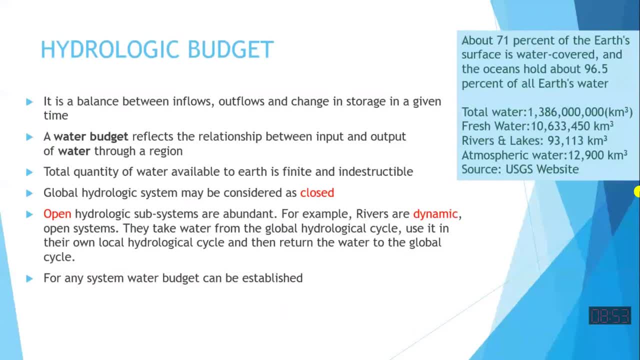 You cannot manage a resource if you cannot measure it. You cannot manage a resource if it is not measurable. So for better management of water resources we have to measure it and then we have to account all its components and we have to see which part we can use it more efficiently. 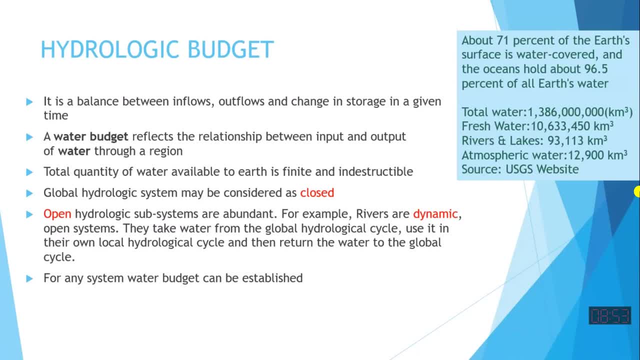 and which part is already under high stress of its utility. So to better manage a resource, we have to measure it first, and after measurement we equate how much water is in flow, how much water is out flow, and stating such things is actually we are talking about budget, of that. 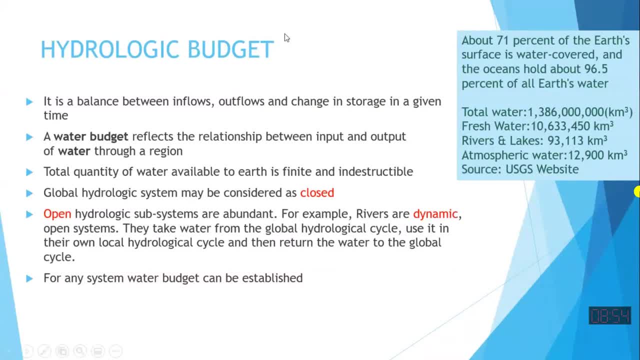 So we can consider that, if we consider our global hydrological cycle, if you think about the hydrological cycle of the whole globe, including the ground, earth, oceans, atmosphere, So this is called a closed system with respect to water. It is not closed with respect to energy, but with respect to water it is closed system. 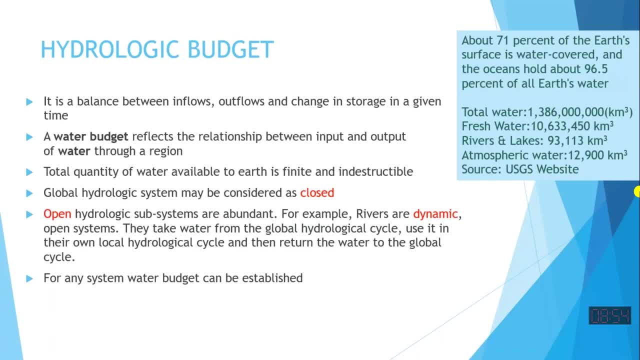 What does it mean? It means that water does not enter into this system and water does not leave this system, So quantity of water in global hydrological cycle is more or less constant. So that's why we call this system as a closed system, while if you take a part of the hydrological 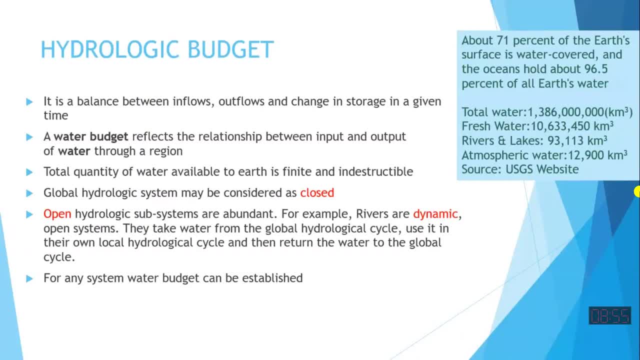 cycle, or you take a length of the river reach, or you take just the ground water, or you take just boundary of a country, So that system is not considered closed hydrologically. For example, if you take a 100 kilometer length of the river, you cannot say this is closed. 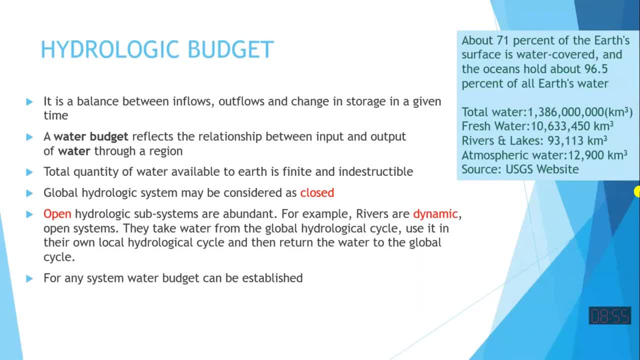 Water is not coming to this reach and water is not going out of this reach. No, not possible. So, with respect to hydrology, we can say that a system is closed system if no inflow or outflow is going out of the boundary of the system. 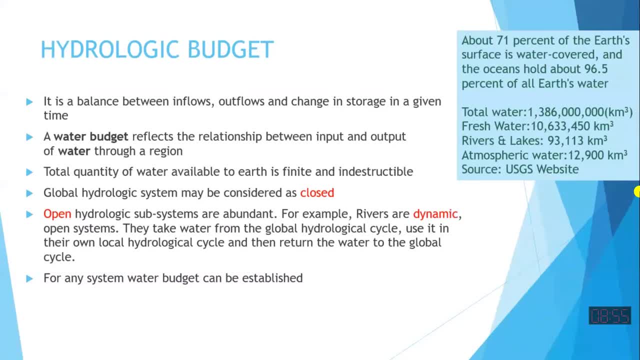 But if it is, its boundaries are porous, So it is closed. So it is closed. It is getting some inflow or releasing some outflow out of the boundary, So we say this is open system. So most of the water budget problems are with respect to open system. 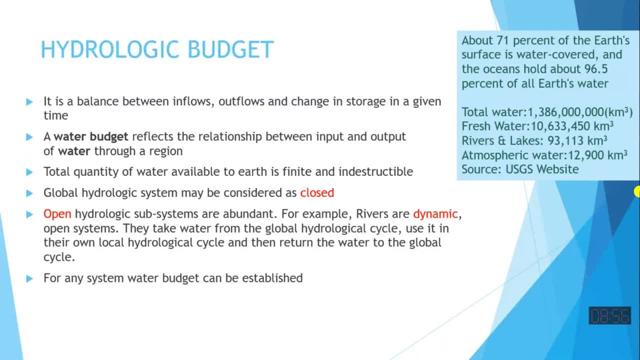 We either I will be talking about. tell me the budget of Pakistan. tell me the budget for Punjab. tell me budget for river reach from Tarbela to Chashmabiraj, So things like that. Tell me the budget of the Ravi from Shadra to Baloki. 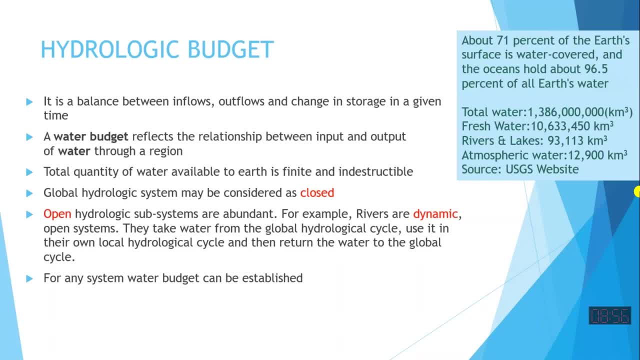 So these are the open system. It will be getting some water inflow, It will be getting some outflow, It will be releasing some water downstream, Some water will be going to the ground underneath, Some water will be evaporating. So with respect to that river, it is very much open system. 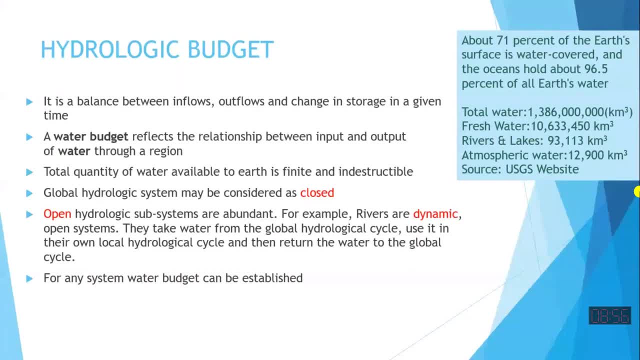 So we should understand two kinds of system. One is called as closed system, one is called as open system. Usually component of the hydrological cycle are open system And we can establish water budget for closed system also and water budget for open system also. 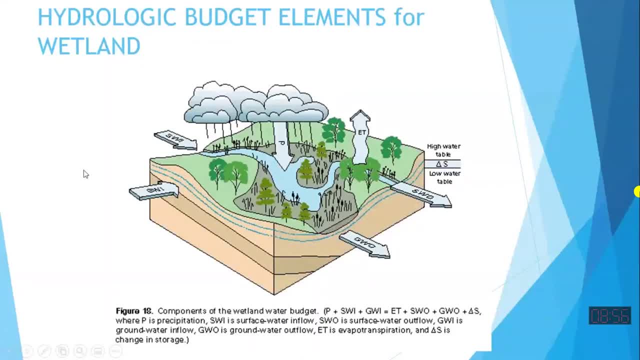 So if we have to make a water budget for a watershed or a part of a watershed, this is part of a watershed with respect to surface water. if we talk about watershed or catchment with respect to surface water only, I am not talking about atmosphere. 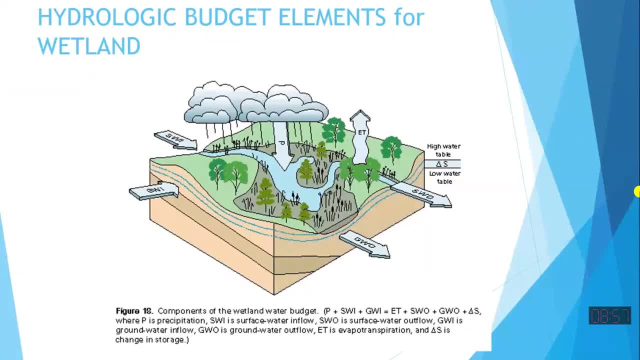 I am not talking about ground, Just surface water, that a watershed is closed if there is no transfer of water from other watersheds. sometime we transfer water artificially, sometime naturally river is coming, okay. so watershed can be considered as closed system with respect to surface water if it it has no trans watershed transfer transfer of water. so 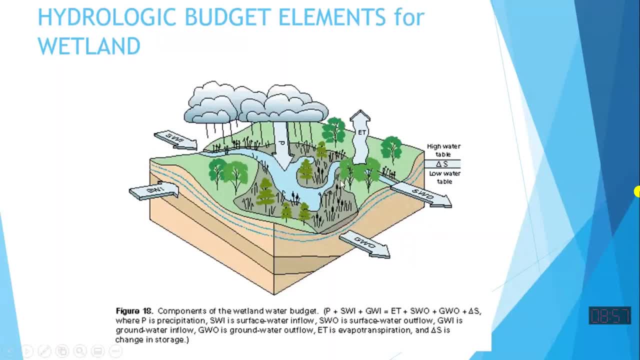 in this watershed. here's the river in this wetland area. wetland area is that area in which most of the time water is standing, like Delta area coastal regions. so most of the time water is wetland habitat over there and they have got it in a perspective view three. 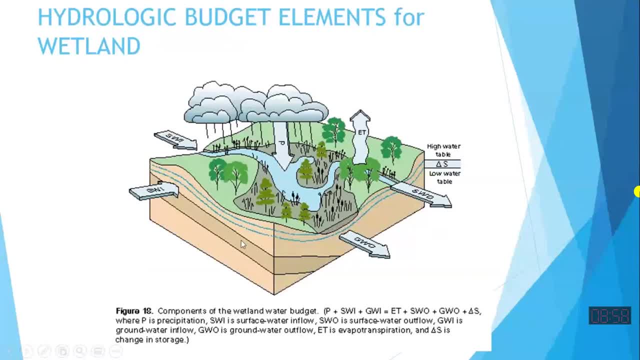 dimensional view, you can see that the water is coming from this watershed and you can see the layers of the groundwater over here. you can see the surface water over here. so they are telling you if you have to estimate the budget or if you have to write the equation or quantity of a budget of 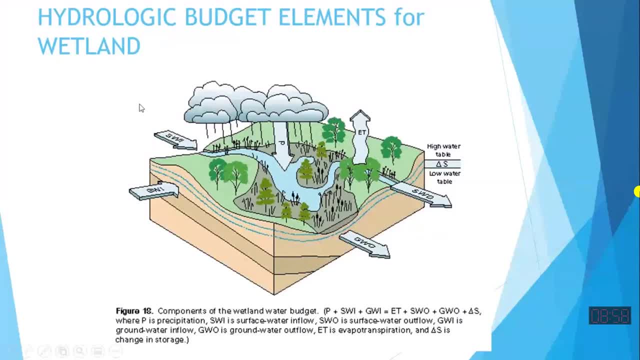 water in this area, so you have to take into account these components. for example, this wetland is not closed at upper boundary. water is flowing from here, upper part, to the lower part and going in this way, so it is not closed over here. so you have to quantify how much is water coming through the surface. 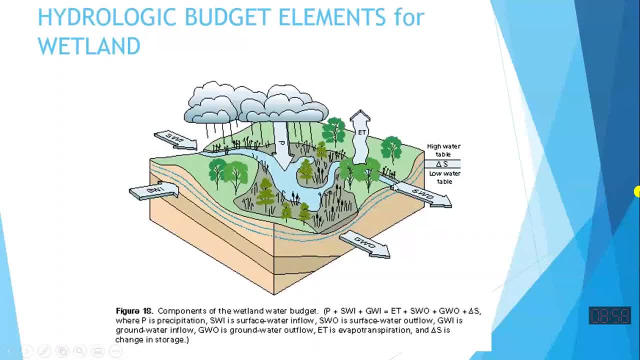 water is not closed at the downstream boundary so you have to quantify or you should have knowledge of water going out in a certain time period out of this area under the ground water is. there is not impermeable boundary vertically, so some water will be coming from the side area or it will going. 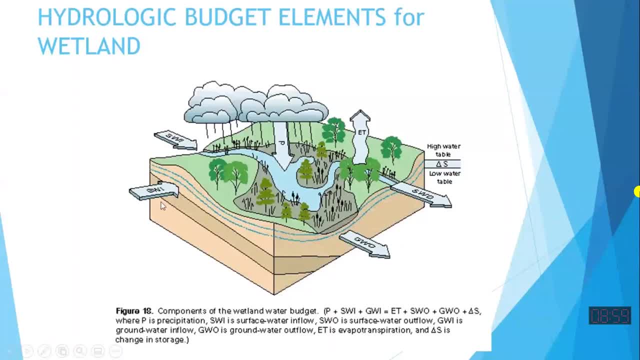 towards the side area. so we have to take into account these things. at the moment we don't know the quantity, only consider what we have to account for. we have to take into account. so some water will be coming from atmosphere. you have to take into account that is a precipitation. some water will 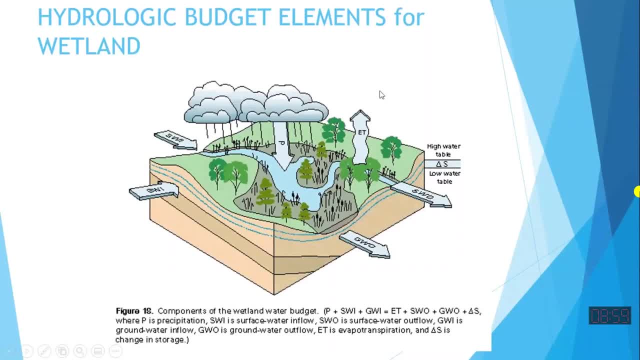 be going back to atmosphere. we have to take it into consideration. that is our transpiration, soil moisture and depression storage. so all of these, if I call storage, so soil moisture and the storage in this area will not be remaining constant previously. let us say all the soil moisture if I combine together all the water which was standing in the depression storage, if I 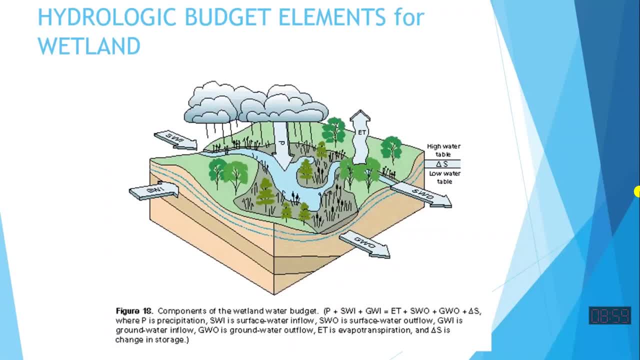 combine together if it was storage s1. so after a certain time period that storage will change. it will not remain constant. so change of storage I have to take into account. so these are, through figure and through labelling, different parts of water. we are trying to tell you what components. 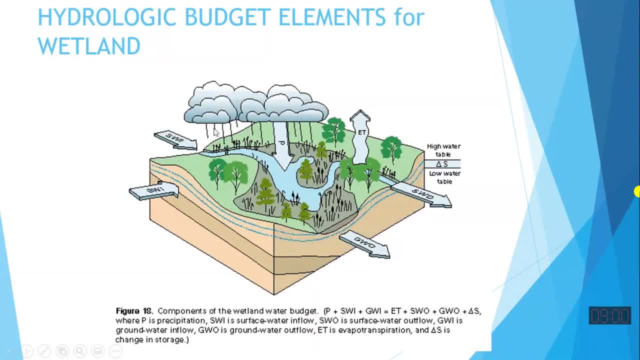 of water you have to take into account. take into account if you are budgeting the water in this area, so you should be able to name them, you should be able to identify them, you should be able to know whether it is inflow for this area or it is outflow for this area, for example, if i am making the budget for this surface water. 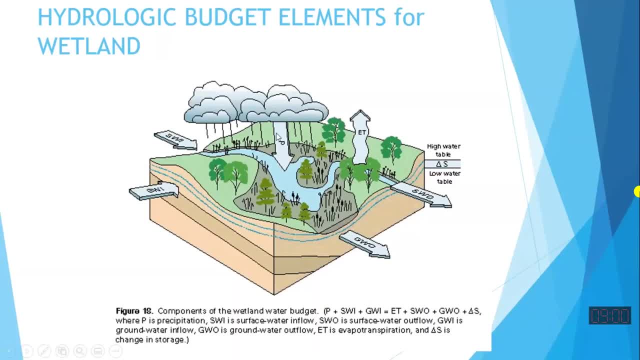 precipitation is inflow. but if i am making budget for atmosphere, understand this thing. if i am making budget for atmosphere, then precipitation is outflow for that system. but if i am making budget for the surface water, then precipitation is inflow for that. similarly, infiltration to the soil. 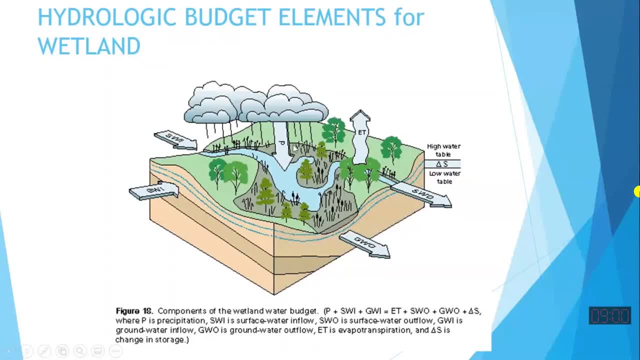 is outflow for the surface water. infiltration to the soil is outflow for the surface water system, if i am considering surface water system, but it is a kind of inflow for a body, for a person who is considering only the groundwater system, for a groundwater system. 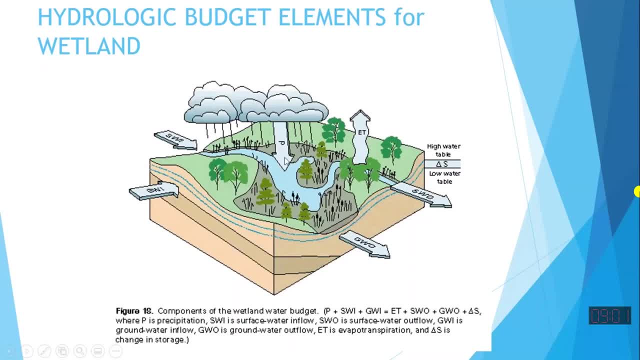 infiltration is inflow. so you have to recognize the component and you have to recognize- and these are easy to recognize- what system you are studying. you should understand what are its boundaries. so anything coming to that boundary is coming into that boundaries. inflow anything leaving out of that bond. so these boundaries you have to define yourself. 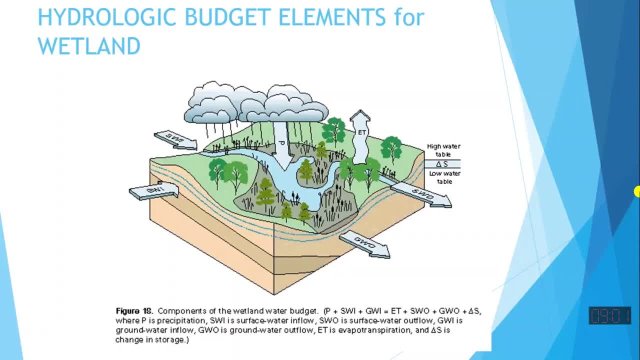 depending upon the problem you are solving. if you are solving the budget problem for the whole hydrological cycle, so then your upper boundary will be a space, the top of the troposphere. we consider that most of the hydrological activity occurs in the troposphere, that is. 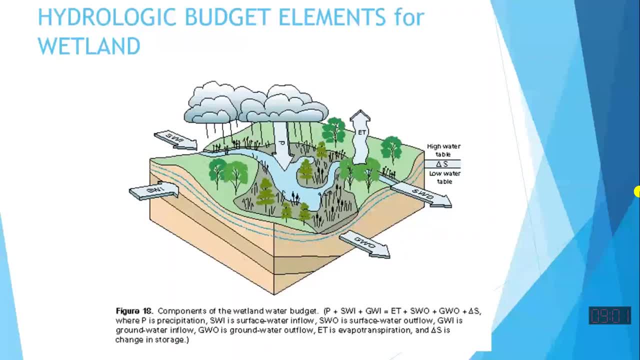 about 10 kilometer long depth of the atmosphere. above that hydrological activities are very less significant, so our metrological activities are less significant. so boundaries you have to fix yourself. if you are talking about the whole hydrological cycle software area, is that the lower area in under the ground maybe? 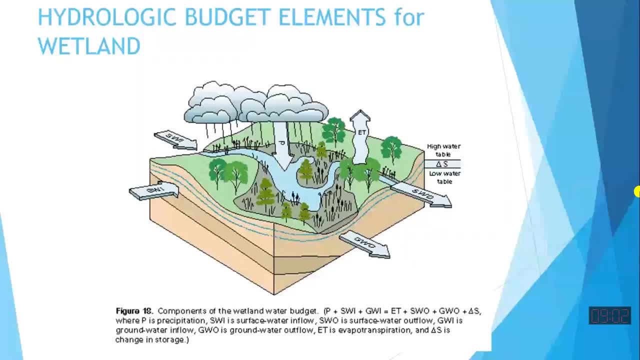 you don't need to go to the center of the earth. you the upper part of the groundwater table, below which no effect of inflow or outflow will happen within your time period of analysis, so that can be considered as a lower boundary, for example, if you have a groundwater system in which you are. 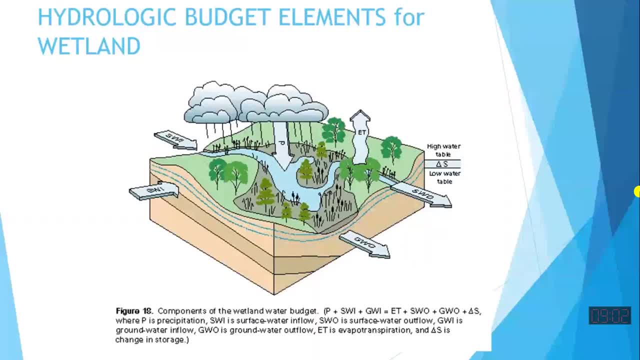 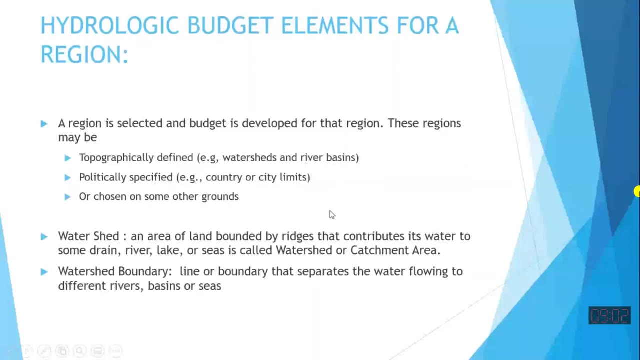 horizontal boundary. similarly, you have to see if you are considering the whole globe. so the whole globe is your boundaries on the surface. so, considering the boundaries of the system, you can understand which one is in flow, which one is out. so I take a break over here and then, if you have any, if you have any, 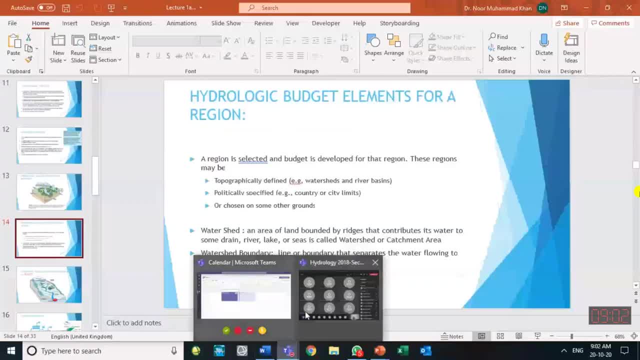 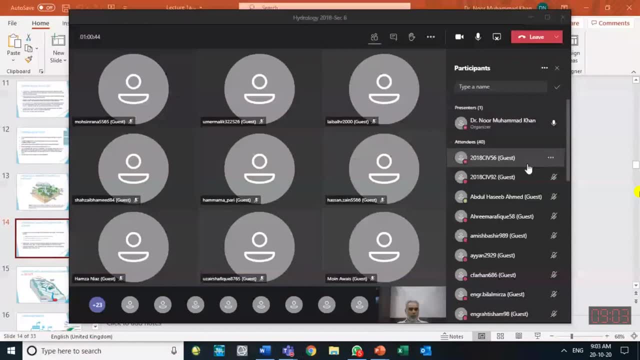 question. you are welcome to ask it now. I forgot to record it, so maybe after the break we can record also. at the moment, 40 students are there, so are you with me? are you getting something? any questions, any queries which come to your mind, you are welcome. 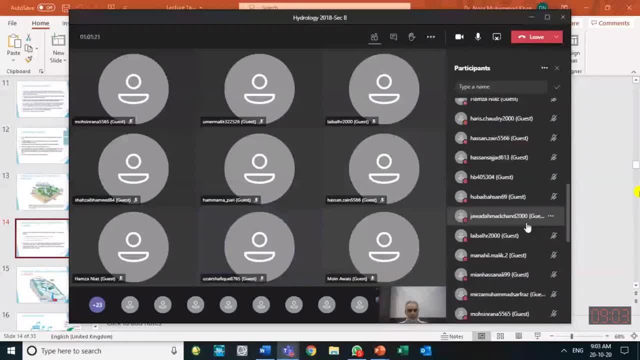 hibernet. what is going on? how is your studies going, Sir? I am going well. ok, you would like to join the university? on the campus, yes, sir, this is a family, so you can study on the bed. no, sir, on the campus. on the campus, friends are going. we are missing something. 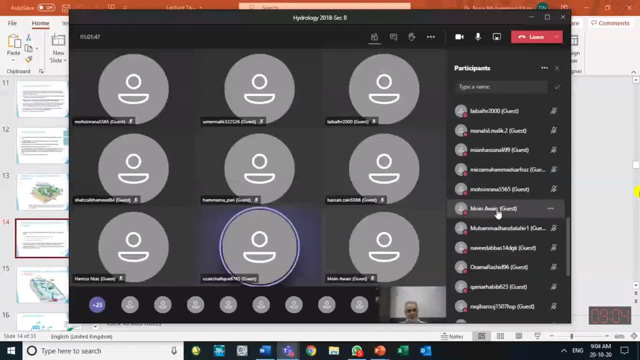 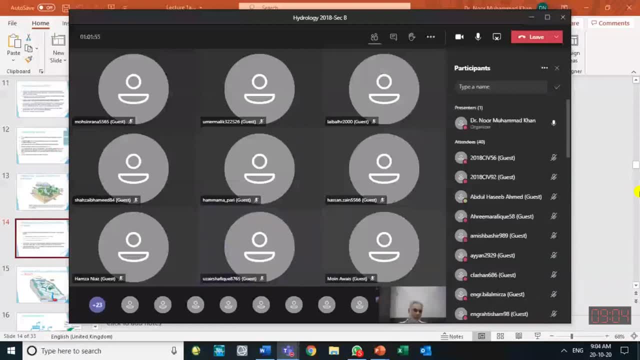 are you missing Bhola's canteen? yes, sir, sir, we are missing everything. ok, may god help us to come to normal conditions. see you at. it is 9. if you have any question, you are welcome. any question, any problem? ok, so I will join again at 9.15. 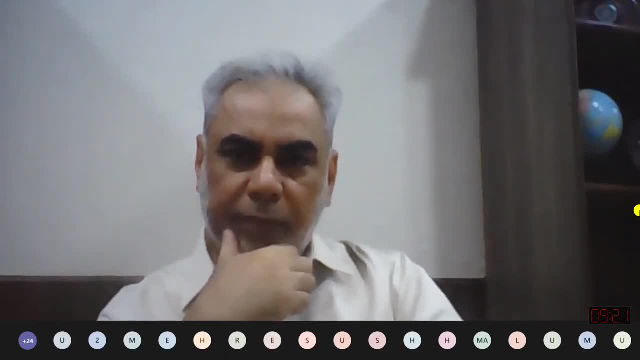 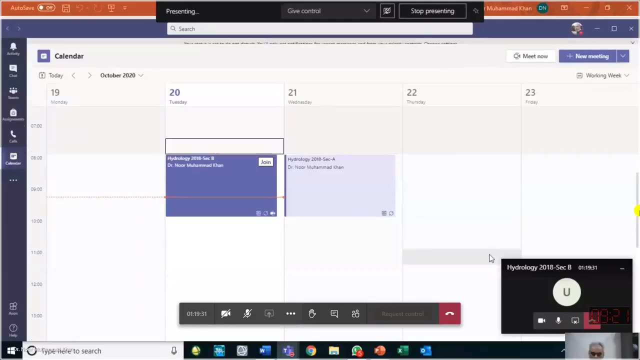 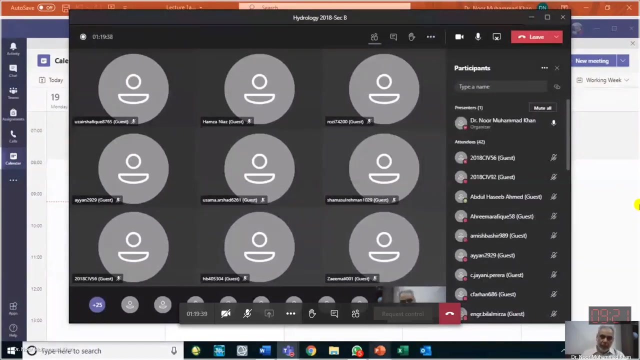 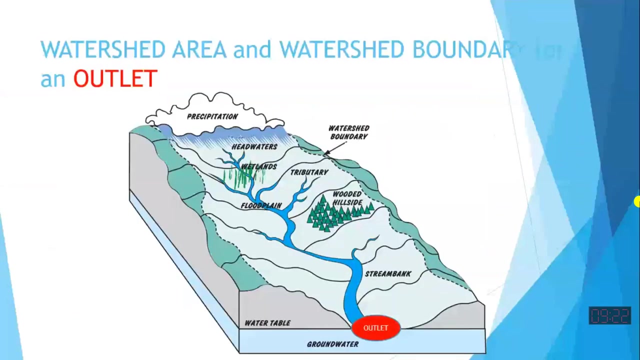 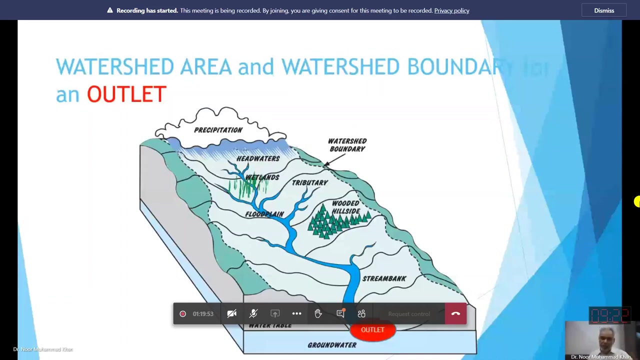 ok, welcome back after break. I am starting the recording. I am coming back to the presentation, so here I have shown outlet and catchment. if I change the location of the outlet, if I bring it over here, so catchment will not be then remain same, then catchment will be only that area which is contributing water at the new location. 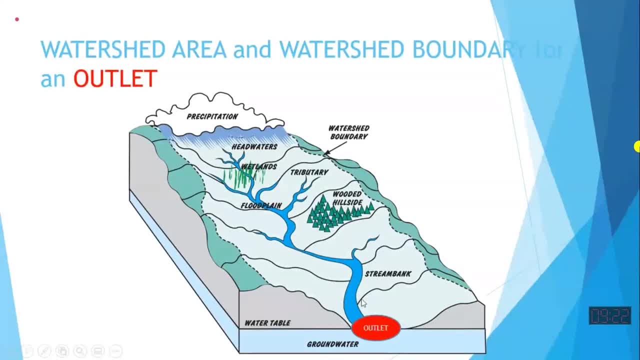 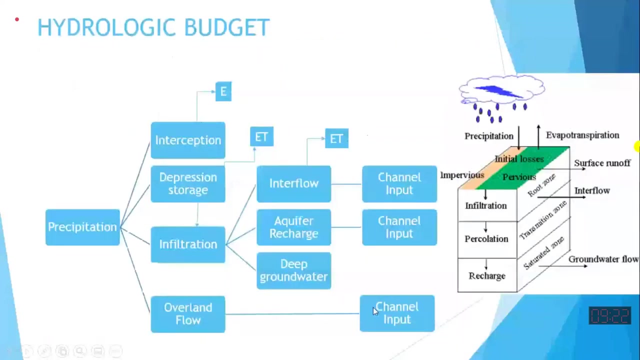 if I move this outlet to- if you are seeing the mouse location- to a small river end over here. so then catchment will be only that part which is providing water to that outlet. so that will be only catchment. have you got it? so catchment is dependent upon location of the outlet. 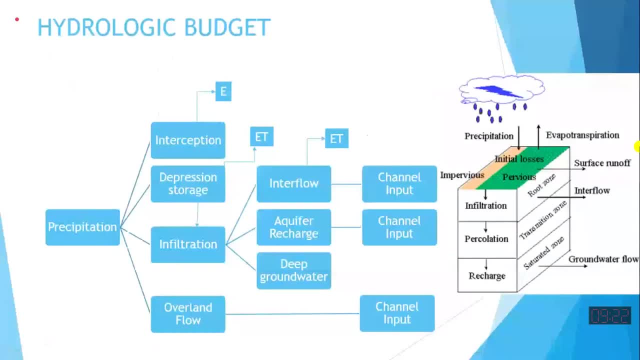 this hydrological budget. when precipitation occurs, what happens to it is in a flow chart form is shown over here. precipitation occurs in: some is intercepted, some is evaporated, some goes to depression storage and from there some is evaporated, some is infiltrated, some directly infiltrates. 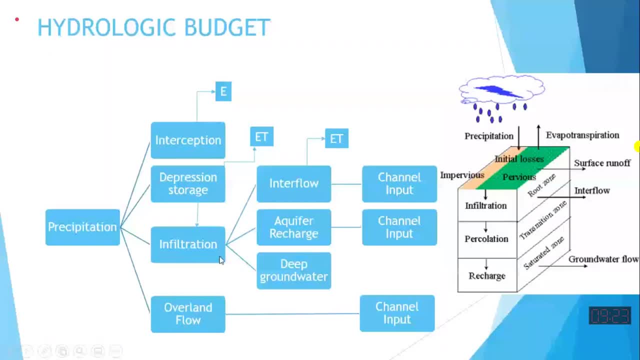 some over land flow and then becomes channel flows in the infiltration there is inter flow, there is deep ground water which occurs so, and then that underground water also sometimes comes back to the surface water as a channel into springs. so this is another way to show different processes. 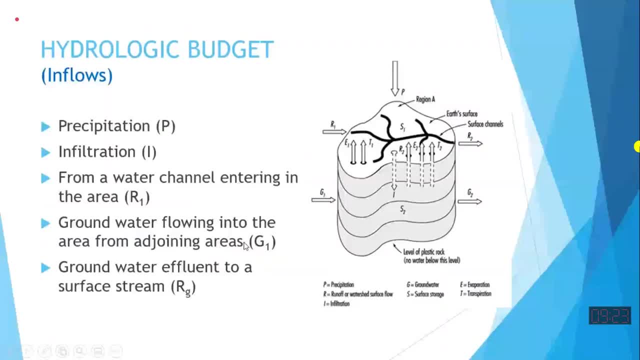 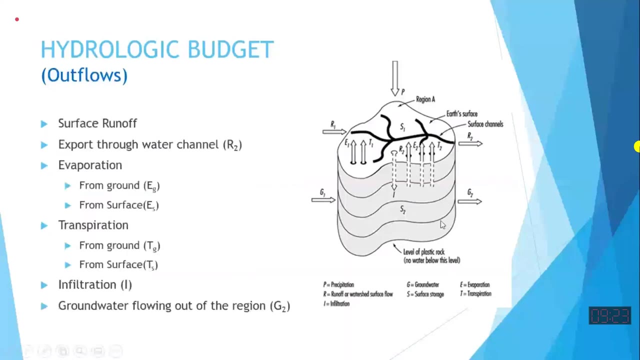 so if we have to make a hydrological budget for a certain catchment, then you can see what are the inflows. in the next slide we will be showing you what are the outflows and what are the storages. there can be three types of things. 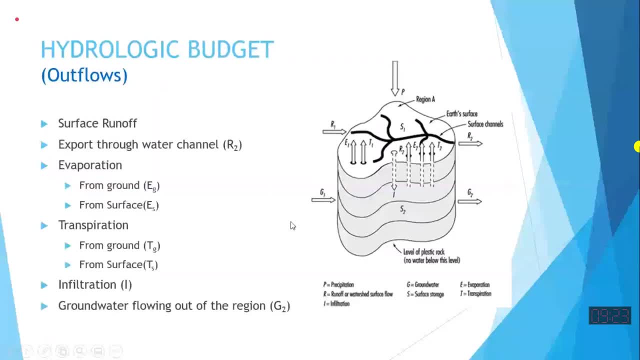 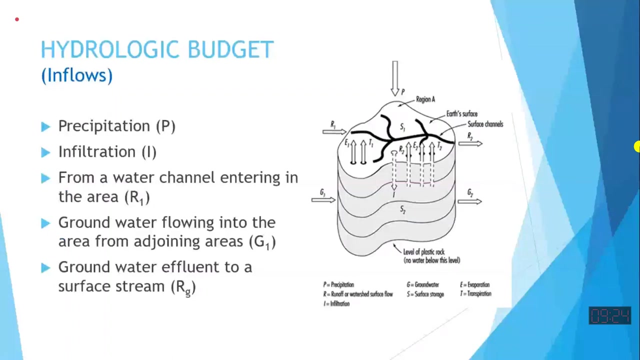 in writing an equation for hydrological budget. and I already told you, hydrological budget is a statement of inflows: water inflows and outflows for a certain region or certain area or a certain component of hydrological cycle. so we have to identify inflows, we have to identify outflows. 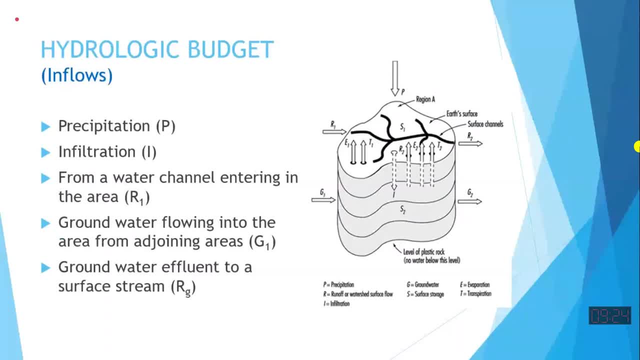 we have to identify storages and then we have to quantify them. first we identify them, then quantify them. sometimes we say, oh, this component of budget is very minute, I can ignore it. sometimes we cannot estimate it and we find alternate way to estimate it. one benefit of writing a hydrological budget equation is: 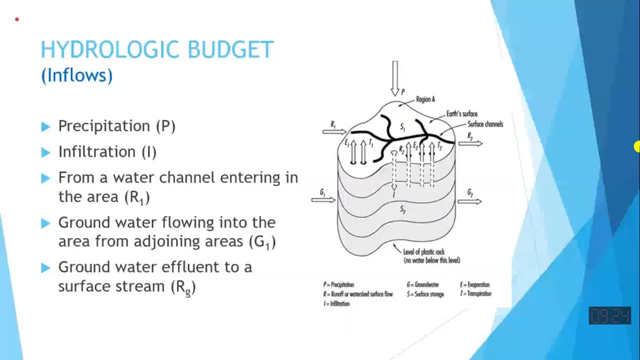 we can use an equation to find one unknown if all the other part of the equations are known so far. so okay, we go step by step. what can be possible inflows? if we have to budget, we have to write the budget equation. what are the possible inflows? 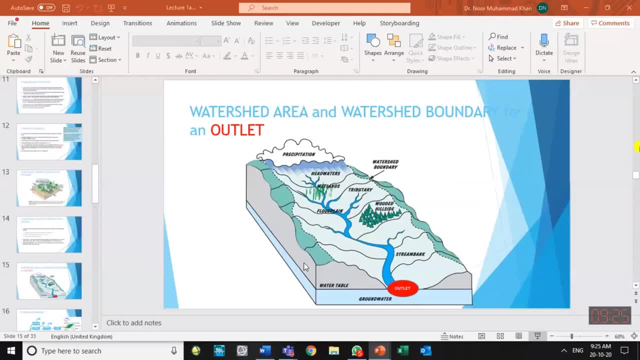 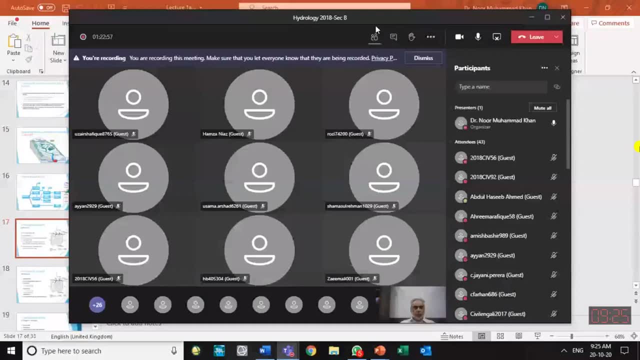 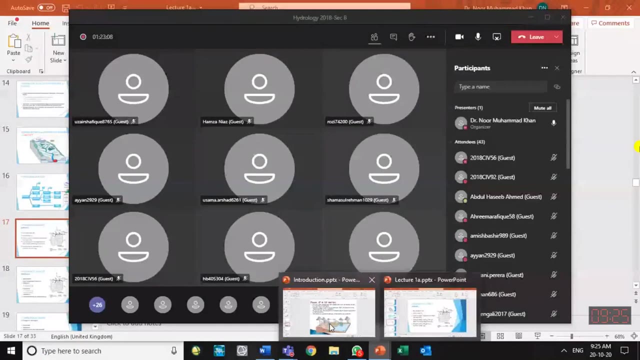 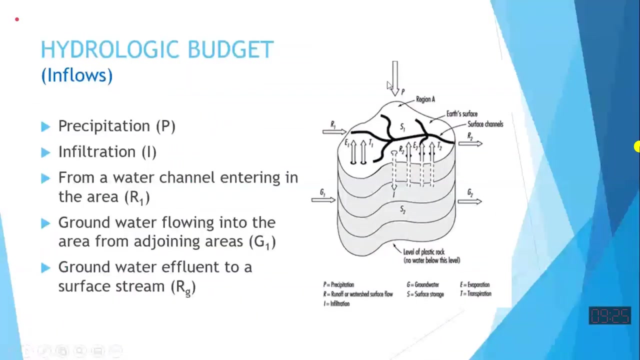 so those are written over here. at the moment, 43 students are there. you are recording this. hmm, so precipitation will be most of the time. for our hydrological part, surface water and the ground water, precipitation will be considered as inflow, while also the infiltration will be considered inflow. 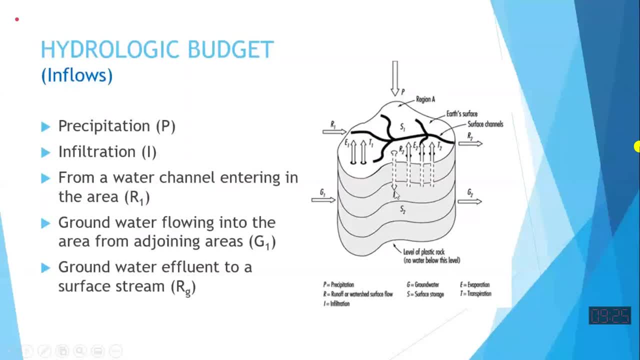 for ground water and it will be considered outflow for surface water. for a system of water, it will infiltration, will be considered inflow for ground water system and it will be considered as outflow for surface water. so if it is infiltration is mentioned over here, it means it is with respect to the ground water. 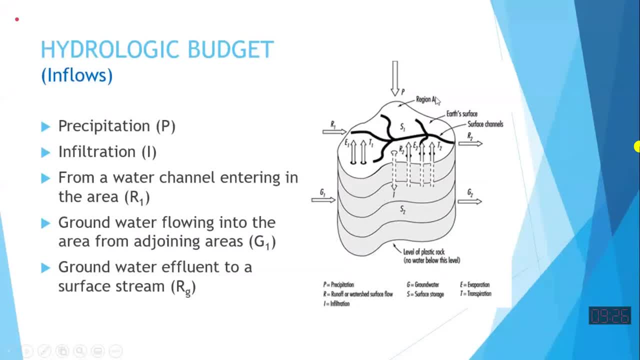 so because we want to make the hydrological budget for all this part, ground water and surface water. although we can make budget for surface water separately, we can make the budget for ground water separately and then we can combine them together. so what are the possible inflows? 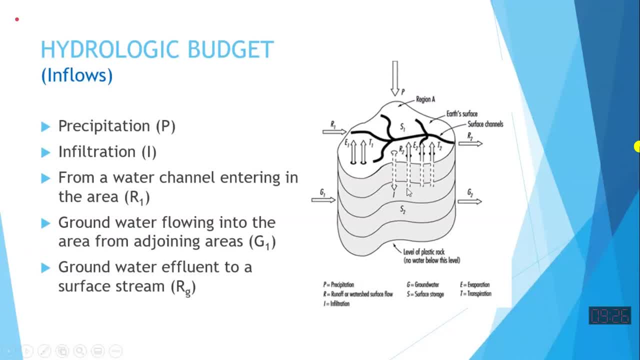 for surface water. what are the possible inflows for the ground water? all the inflows are mentioned over here. so precipitation is inflow for the surface water. infiltration is inflow for ground water. any water which is coming to the surface through the surface bodies, like rivers. 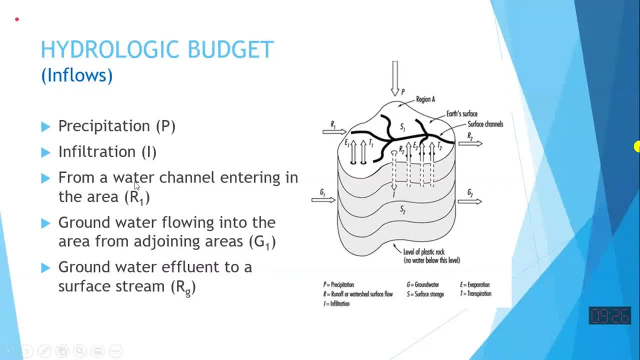 so that will be considered as the inflow water from a channel entering into the area that is shown over here and written over here. so water entering into the channel from the surface bodies, that will be considered as inflow ground water flowing into the area from it joining. 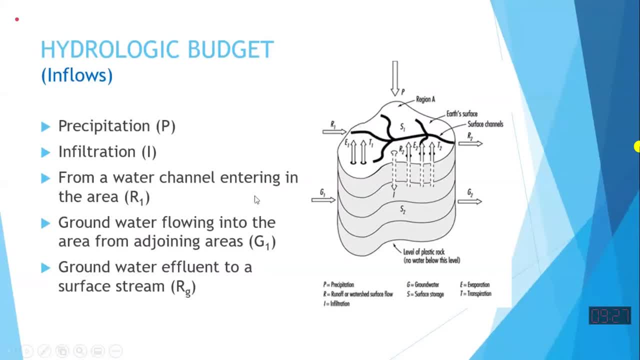 like surface water flows to the area, underground water also is flowing, although not with the same speed as the surface water is flowing. ground water is moving with a very slow speed because of the pores, because of the friction within the soil. so, although it is moving towards the lower gravity, 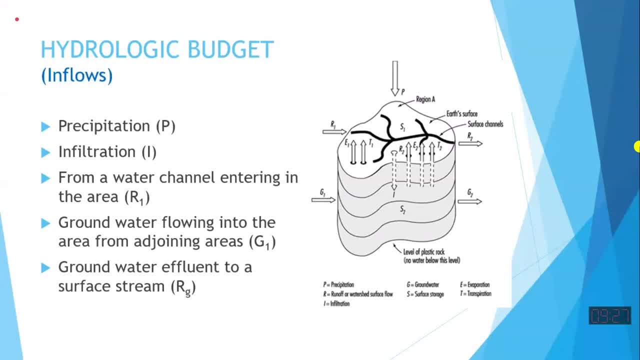 lower water levels in the ground so, but it is flowing. so any water which is coming to the boundary of this area, so that will be through the soil, underneath the soil, so that will be considered as a ground water flow. similarly, if there is any ground water, RG. 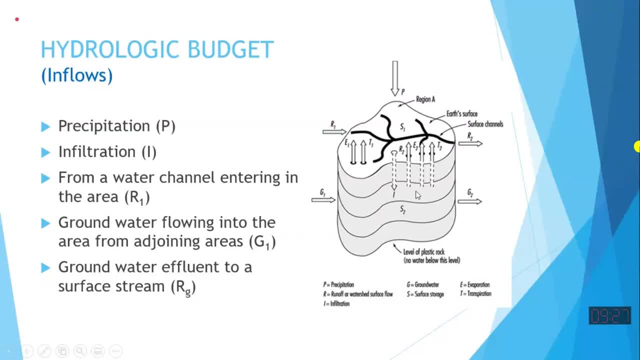 ground water effluent to a surface stream. if some water is moving from the ground to the surface, it has represented that through RG. so that will be inflow to the surface flow, that will be outflow for the underground system. so these are some of the inflows. 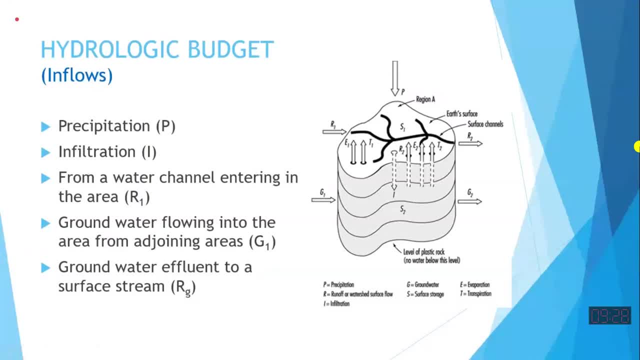 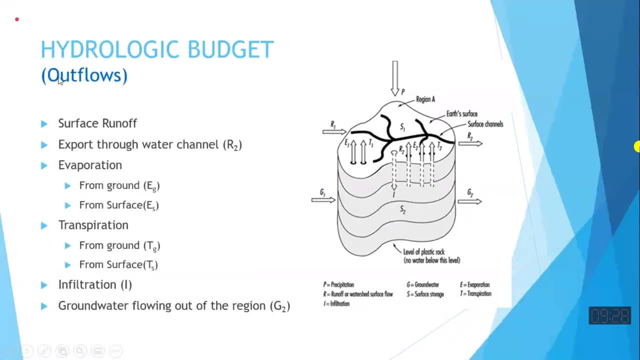 which are possibly affecting the budget of this area. why not? evaporation is mentioned because evaporation is not inflow to the surface or ground. evaporation is outflow. so that will be mentioned in the next slide when we will be moving to that. so next slide is showing mostly the outflows. 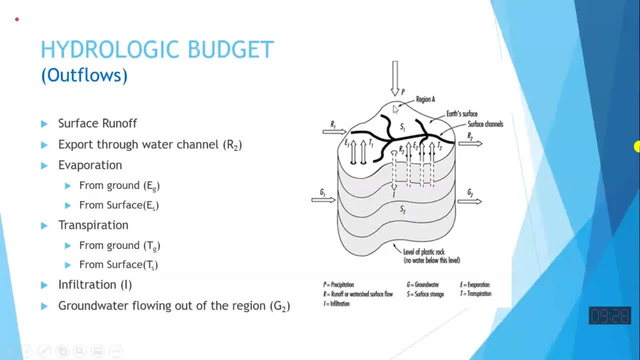 now, precipitation is not represented over here. now only the outflow components are mentioned over here. so any water which is going out of the system through the surface, that is, a surface runoff, or through the channel, so that will be considered as outflow from the system, any ground water which is flowing out of the region. 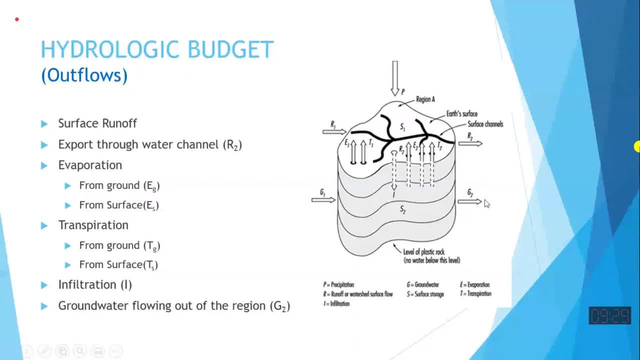 G2, so that will be considered as outflow of the system. so evaporation from the ground and evaporation from the surface water, from the ground water and the surface water. if evaporation occur from the soil moisture, we say this is evaporation from the ground. 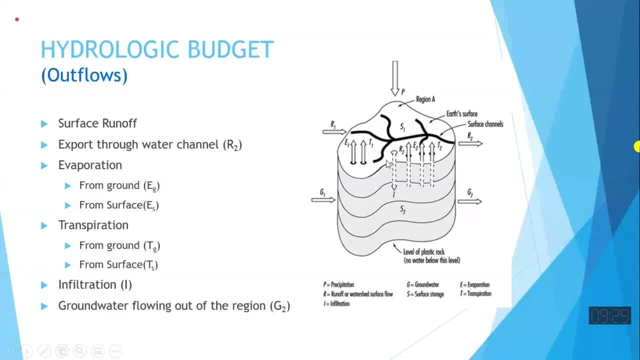 if evaporation occur from the water body, like rivers and the ponds and the streams, so we say this is a surface evaporation. so these are considered as outflow evaporation, either from the soil moisture, that is, the evaporation from the ground, or evaporation from the surface. 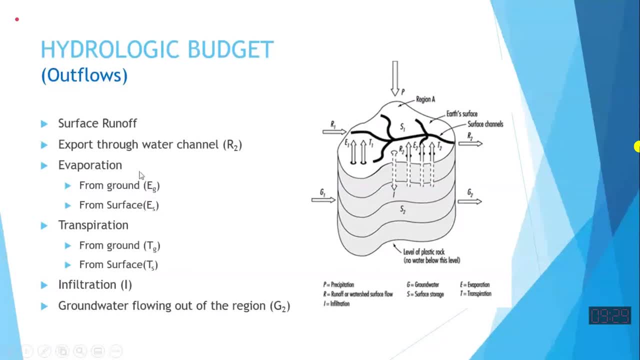 so that will be the outflow transpiration. if there is a tree over here and water is evaporation through the leaves of the tree, so that will be considered as outflow. infiltration will be considered as outflow for the surface water and it will be considered inflow for the ground water. 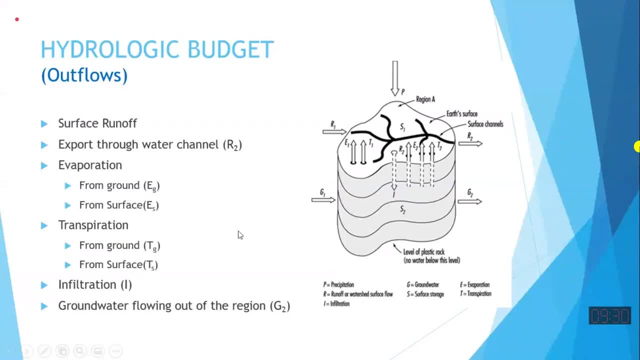 and this ground water I have already mentioned. so just make a sketch of the system, make the boundary of the system and then identify all the possible inflows and all the possible outflow. that is the first step of budgeting: make the system boundaries clear and then identify the inflows. 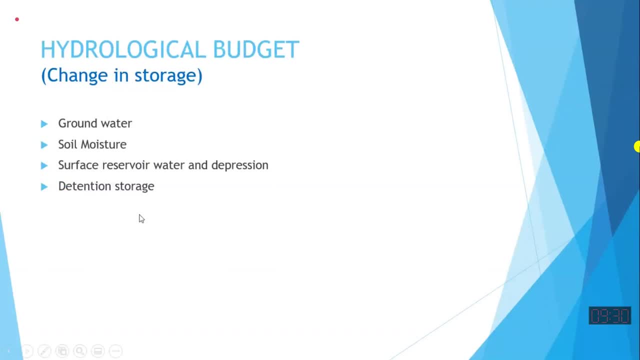 and outflow. then you have to identify what are the possible storage where water remains for certain time. what are the possible storages? so in ground water? water remains for certain time, so ground water quantity increases or reduces in soil, moisture, upper part of the earth or the ground. 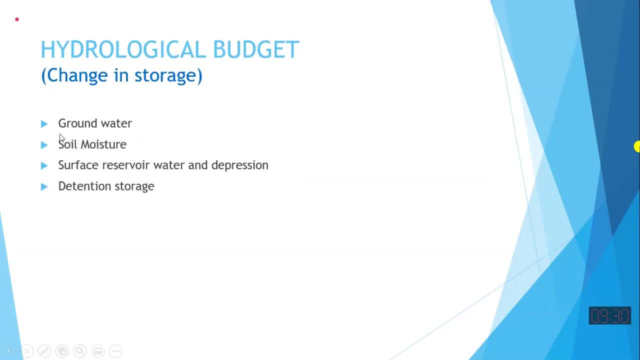 in which water is not saturated but it has the moisture in it. so that is the soil, moisture, surface reservoir, water and depression. so these are the storages at the surface. it can be natural depression, it can be manmade reservoirs, detention storage also some kind of reservoir. where would detain water? 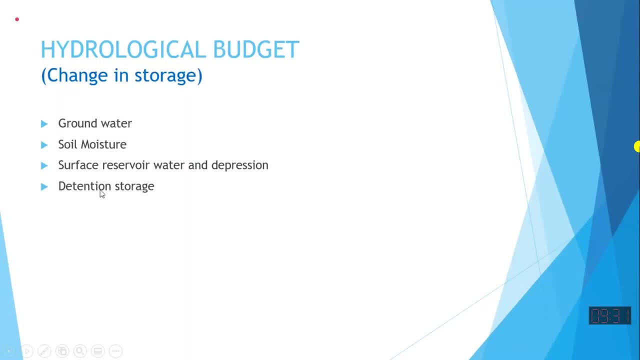 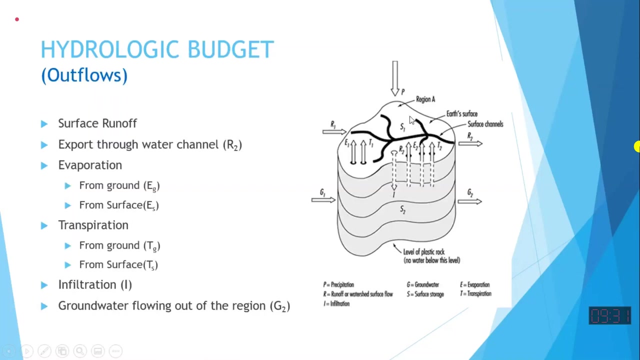 so all of these storage we have to identify in the system so that they can be properly accounted for. other component which you can talk that, why not we are mentioning the biological water over here, that is, theoretically it is there. why not we are mentioning the water present in the trees? 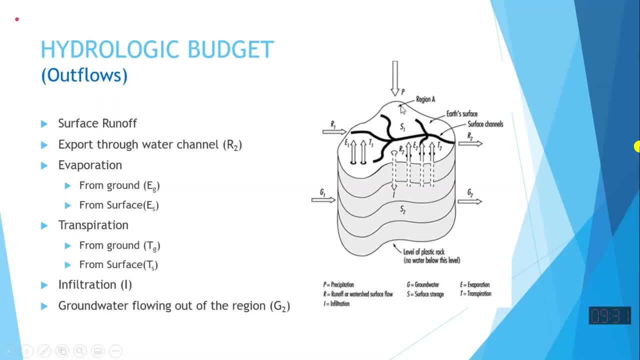 that is theoretically present over there, but these are highly difficult to identify, to measure, and the second thing is their quantity is very small. so that's why some of the small quantities of water storages, those are not mentioned over here. so when we have identified all of these, 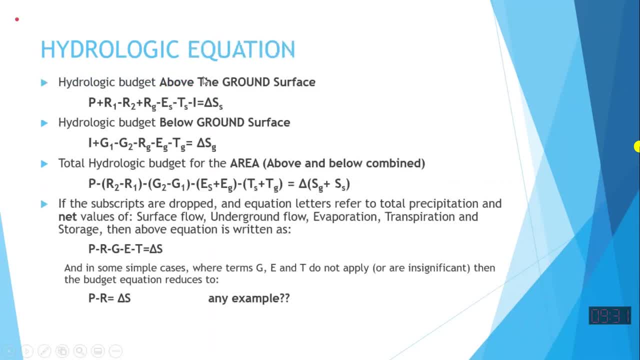 we can write the budget equation, hydrological budget equation for, for the system above the ground surface, for the system below the ground surface, and then we can combine them together and that will be hydrological budget equation for the complete system. so that writing this, if you understand. 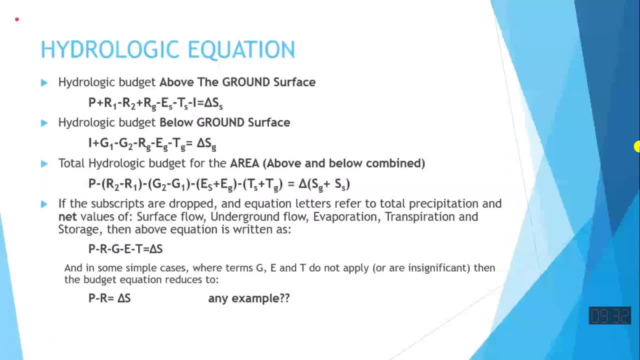 you can write budget equation for any problem which are assigned to you. for example, we can say that in a farm field so much water is applied, so much water is released is going out of that farm. infiltration is negligible. tell me how much is evaporation. so such kind of problem can be assigned. 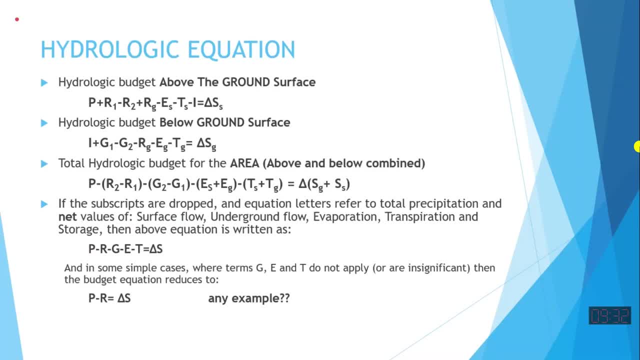 and you can then writing the budget equation. you can see how much is the volume of the inflow, how much is the volume going out. if infiltration is negligible, let us say, then the difference of these two will be the evaporation, something like that you can write. 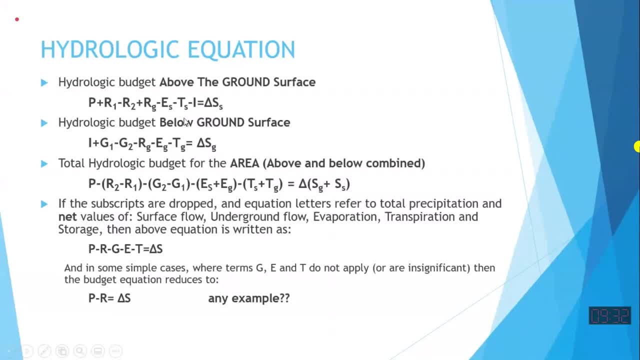 and you can estimate that. so writing this equation, if we have water, budget equation is nothing but statement of inflows and outflows and the change of storage. you have all and this is another name. water budget equation is another name for law of conservation of mass. we believe that mass cannot be created. 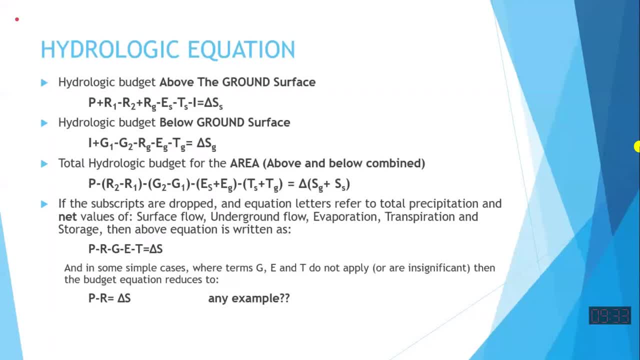 cannot be destroyed. so we believe that within a system, whatever is inflow minus whatever is outflow, the difference should be the change of storage of that mass. so that is what we are writing, so that is the theoretical background at the back end of this equation. so whatever is inflow, we write them. 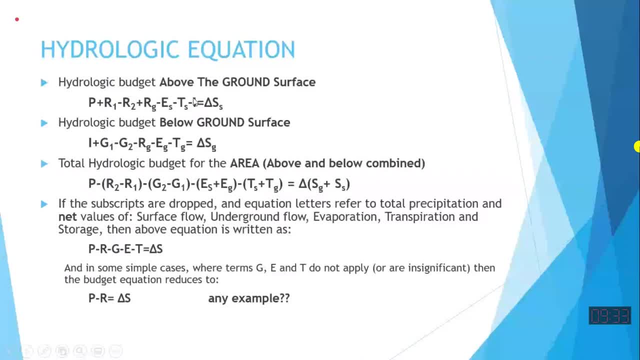 whatever is outflow, we write with the negative sign. so difference of these two, inflow minus outflow, will give you the change of storage. that storage can be storage in the soil. that storage can be storage in the depression, that storage can be any storage in that area. 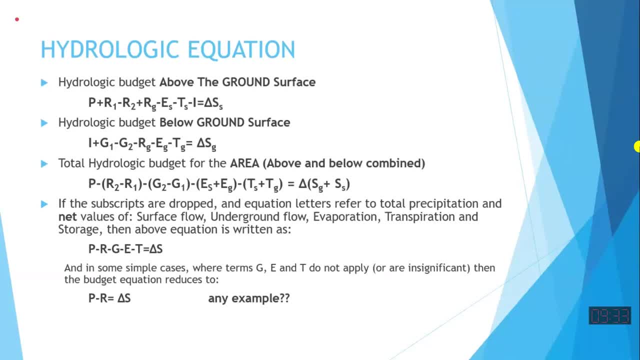 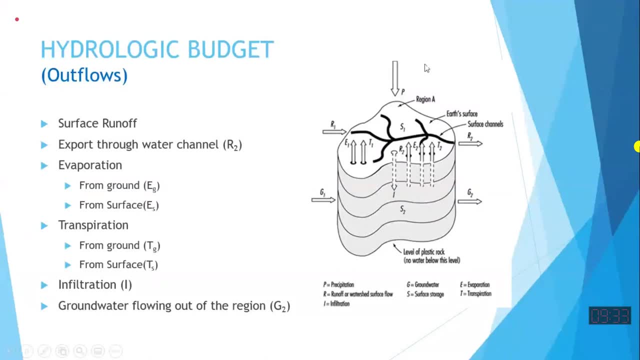 in that system. so if we consider the surface water, if we consider the surface water, so we are then not considering the atmosphere, we are not considering the ground. now bring in your mind this surface, ground surface. so I will ask you to identify what are the inflows. 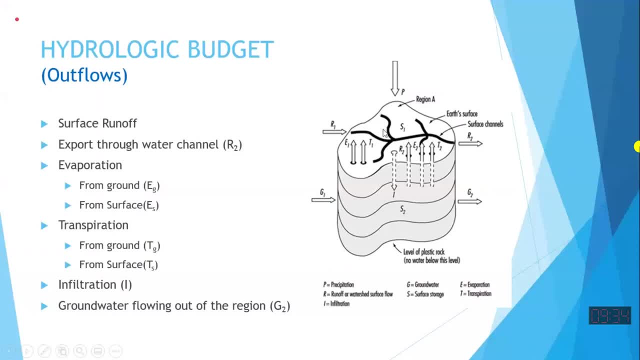 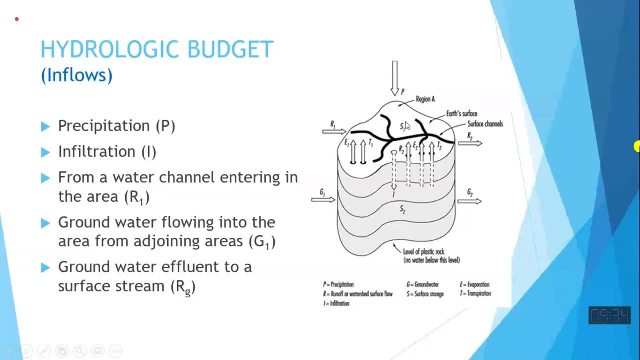 so anybody will tell me only for surface flows, what are the inflows. maybe I go to the previous slide, so anybody will tell me what are the inflows for this surface water and tell me with their symbols. so precipitation is inflow, R1 is inflow. 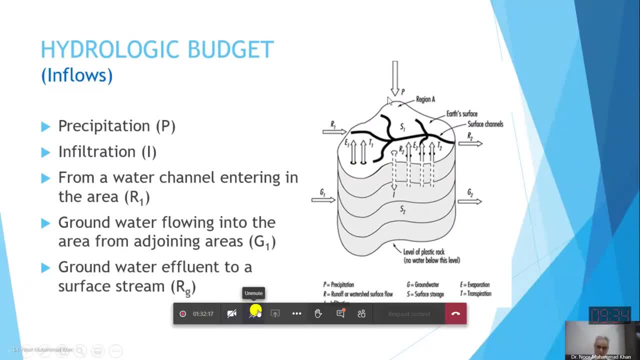 any other inflow: RG component of the ground water which is coming to the surface. actually, what are these? these springs or springs? those are the components which we have to take into account. so RG is ground water component which is coming to the surface, so that will be inflow. 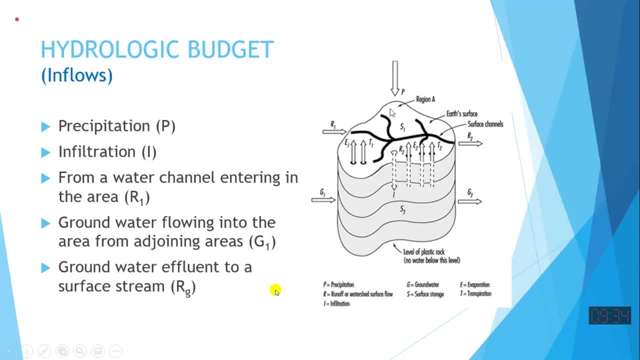 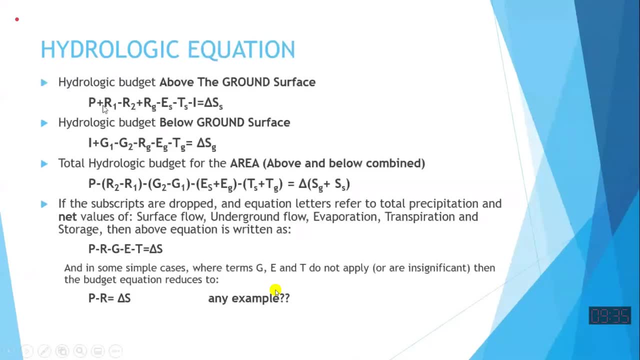 any other inflow, any other inflow. so these are the three inflows. so now, if I see the equation, so this: P, R1 and RG are with the plus sign. so these are inflow to the system. you can write them together: P plus R1 plus RG. 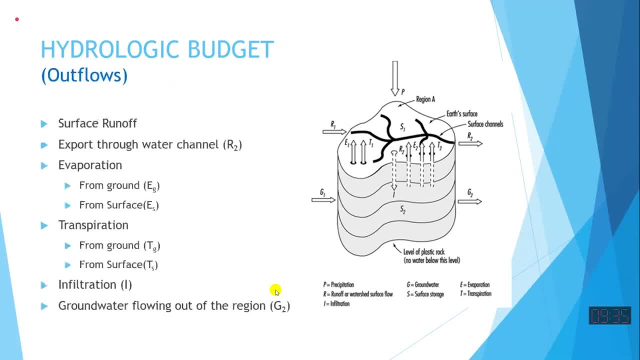 now try to see what are the outflow from the system. and the system we are talking is surface water system, not the ground water. so for this surface water system, what is the outflow? what will be the big outflow? evaporation, evaporation, transpiration or infiltration. 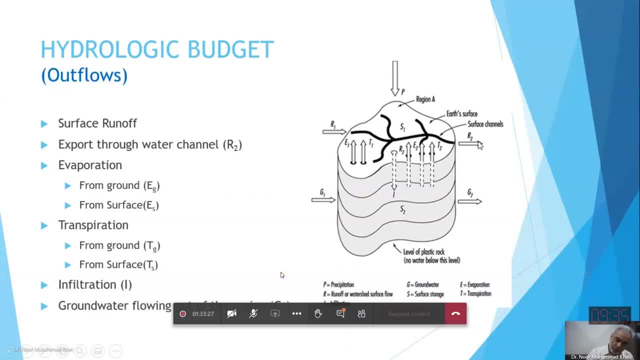 or surface runoff, R2 or nothing else. ok, so evaporation, transpiration, infiltration, the RG which was coming up, it's opposite is infiltration. infiltration is outflow, R2, the R1 inflow, it's inverse or it's parallel. R2 is going out, so writing. 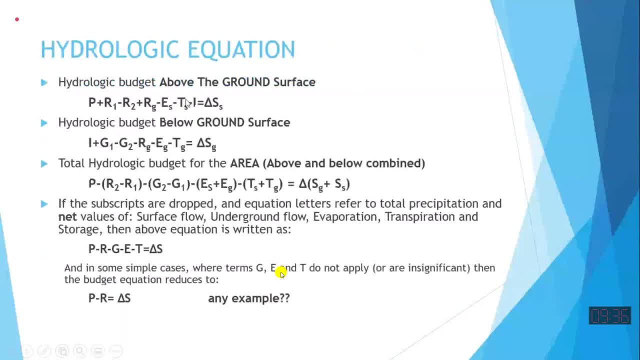 these three terms: evaporation, transpiration, infiltration or surface runoff with the negative sign. so writing inflow with the positive sign, writing outflow with the negative sign. so that is the difference of inflow and outflow. so that should be the change of storage in the surface. 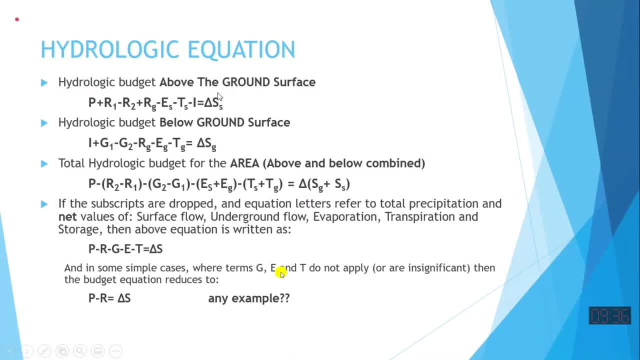 not all storage in the whole system. ground is not included. it is above the ground and also we are not making into account, we are not making the budget of atmosphere. atmosphere water is not included. what is the difference in the storage of the atmosphere? we didn't take that. 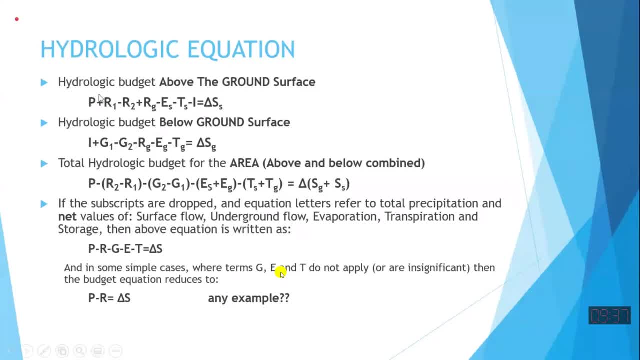 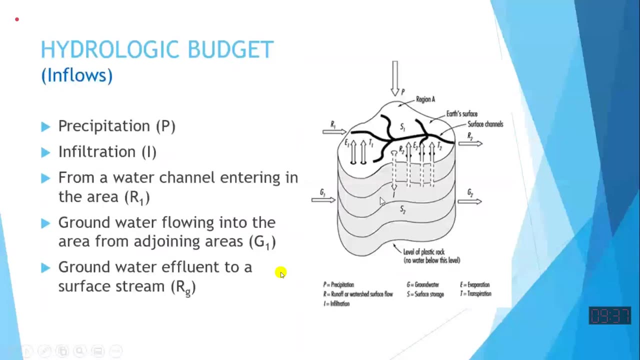 so we are talking about the water on the surface. so inflow minus outflow is change of storage. similarly, you can write the equation for ground water. so if we go to the figure again, what is the inflow to the ground water if you give it label? 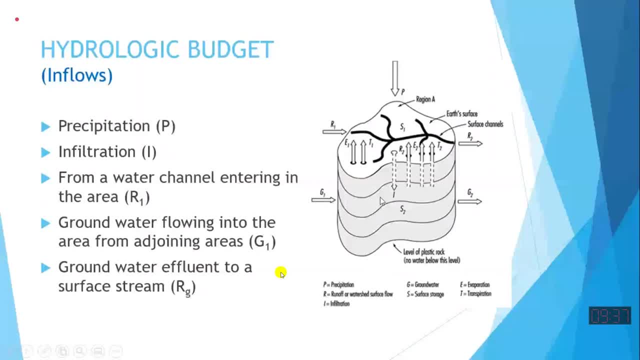 so inflow, major inflow is from infiltration. so here precipitation is not directly helping the ground water. precipitation comes on the surface, then it infiltrates only. the infiltration is the inflow to the ground from the top, then on the side lines ground water which is coming to the ground water. 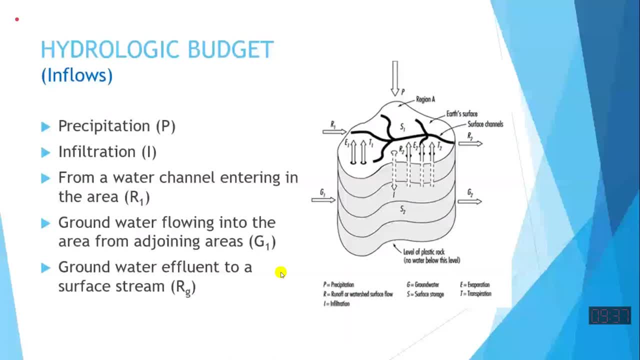 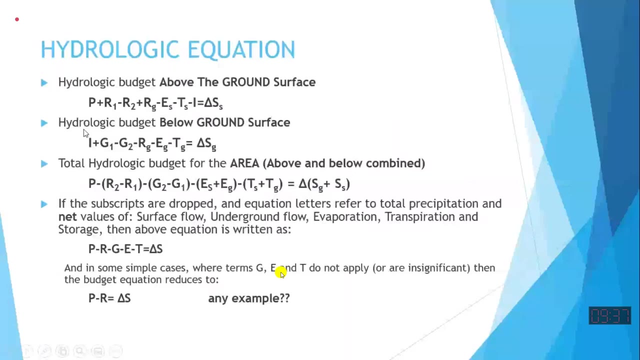 body. that is the inflow. if there is any other inflow, then tell me so. so let us see what inflows are written in the equation. so i and g- infiltration and the ground water coming to the ground water body- is inflow. all the rest are the outflows. 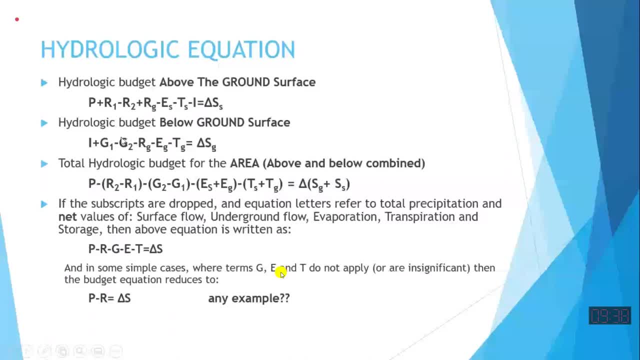 from here. if i say this is the ground water moving out of the system, this is the ground water which is being released to the runoff, surface water, rg, which was inflow here, then each evaporation from the ground, soil moisture, which is evaporation from the ground. 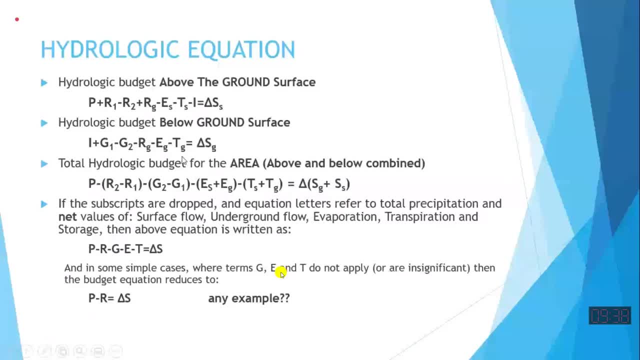 or if there is any vegetation on the ground transpiration. there are sometimes ground water vegetation. is there a small component transpiration from the ground. so these are considered as the outflows. difference should be the change of storage of the ground water body, change of storage when we add left hand side. 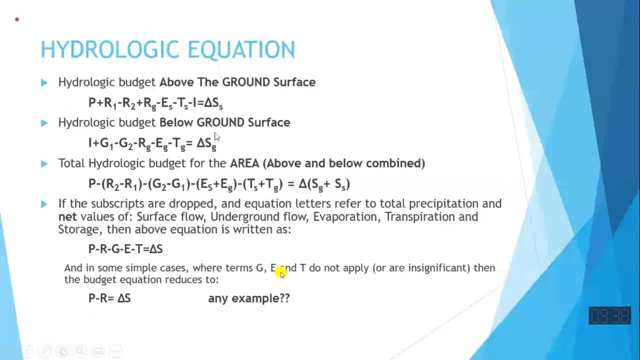 with the left hand side and the right hand side with the right hand side. then we get the total hydrological budget equation for the surface plus ground water system. so that becomes- and we have grouped together the similar things- precipitation minus difference of runoffs. outflow is written. 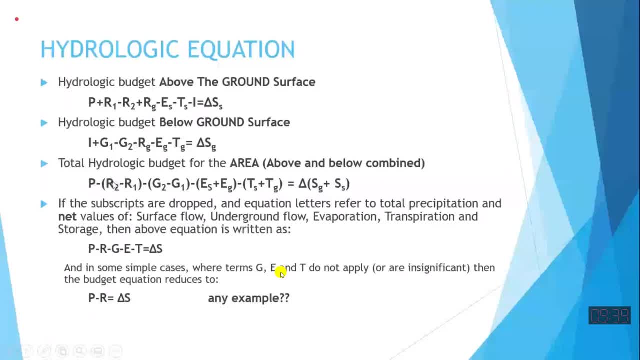 first: r2 outflow. surface outflow is written first and inflow is written with the negative sign. what does it mean? r2 minus r1, if i want to name it, this is the net surface runoff going out of the system. if i say r2 minus r1, 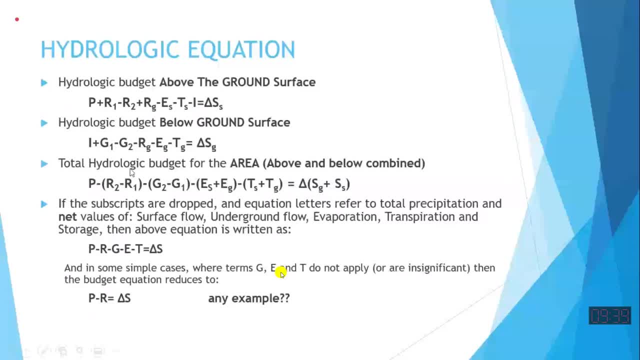 this is the net surface runoff going out of the system. so if it is, r2 is more and r1 is less, so this value will be positive. so it means i am giving positive sign to the higher quantity of water going out. so it means this is a kind of outflow. 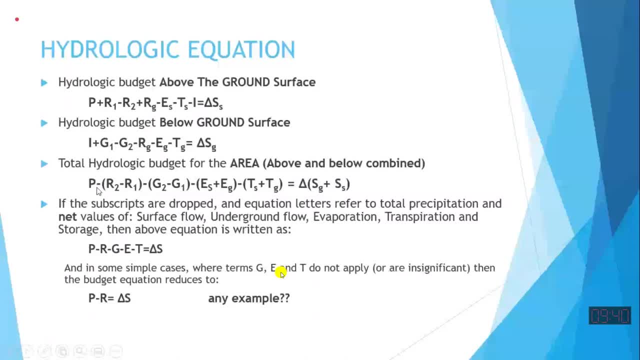 so that's why this negative sign is coming over here. or simply you write them and then you can. if you have written positive sign over here, this should have been then r1 minus r2. simple as this. if you want to keep positive sign, then this: r1 minus r2. 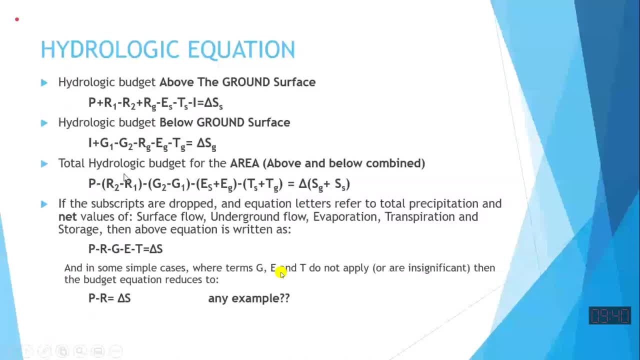 will be positive, it will not matter in your budget equation. but what we have used here is we have made outflows and minused them, so these components are made as net outflows. so then if, for example, sometimes surface runoff is less and surface inflows, surface runoff going out is less, 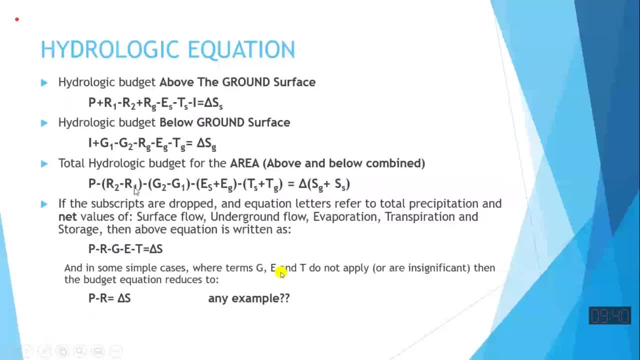 surface runoff coming into the area is more so, then this will be become as a negative. automatically. mathematically this will become negative. so negative multiplied by negative will be overall, this will become input to the system. ok, we have to pay attention to this sign. if you are writing, 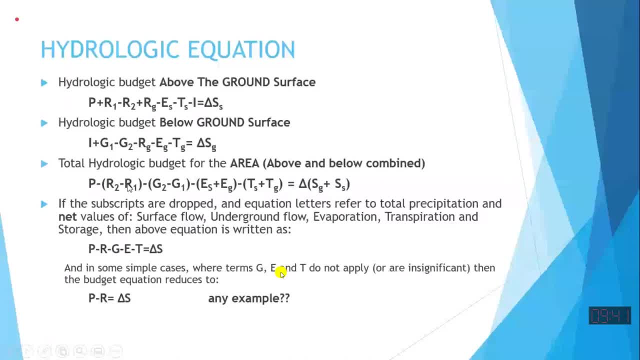 r2 minus r1, then outside should be negative. if you are writing r1 minus r2, then out should. the multiplication at the outside of the bracket should be positive. both way you can write, so result will not matter, but you should be writing it knowingly. if you are writing, 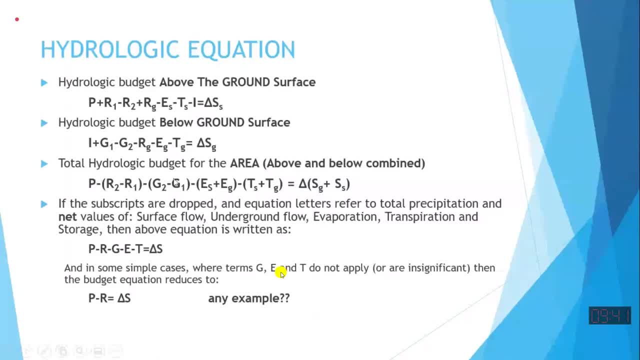 the net outflow as a positive, then it should be negative. ok, now see this: g2 is outflow of the ground water, so that is written first, minus inflow of the ground water, so that is written next. so that is subtracted, so it is net outflow of the ground water. 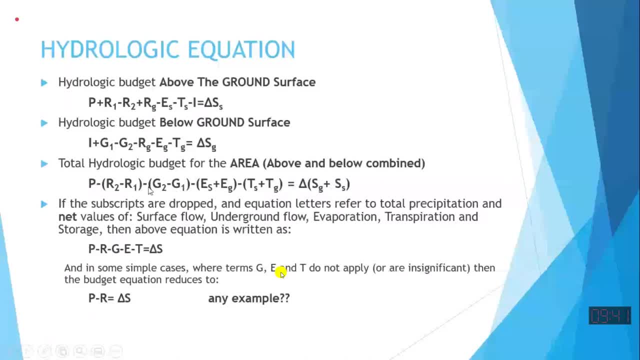 so this should be given the negative sign, and similarly evaporation, similarly transpiration, and on the right hand side we had both of them: change of storage. so this is the complete equation for an area considering ground surface and ground water and the surface water, ignoring effect of 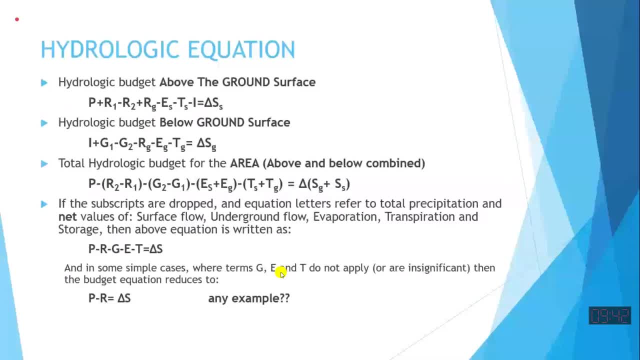 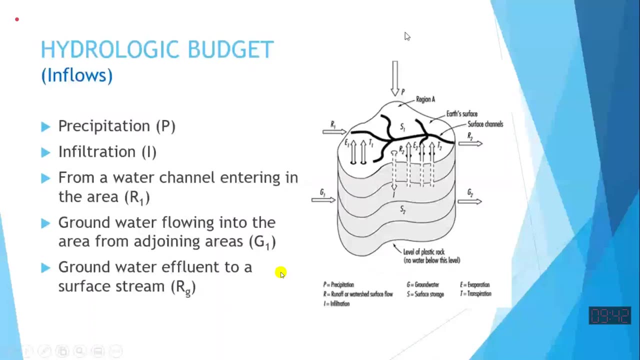 atmospheric water. so if i add atmospheric water also, so then this will be the whole hydrological cycle for that area. so then it will be a closed system over a. no, that will not be. if area is only this one, i cannot say this will be closed system because this: 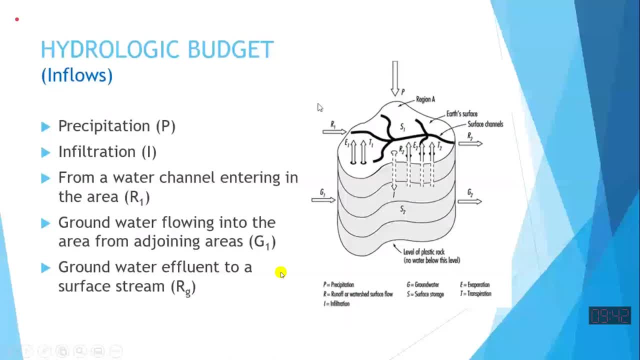 precipitation is not only because of evaporation from here. so this precipitation is occurring over here because of, maybe, evaporation from this area and evaporation from surrounding area also. so we cannot say this is closed area, even if i include that atmospheric water into it. but if i increase this area, 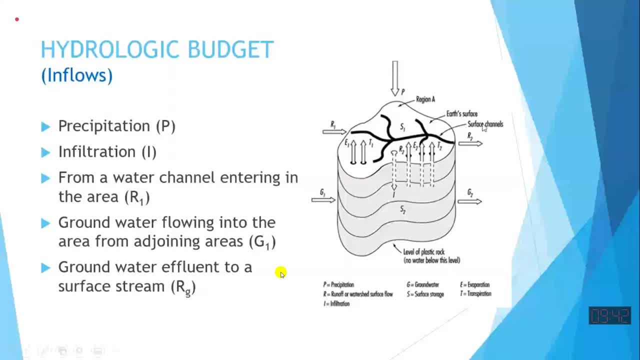 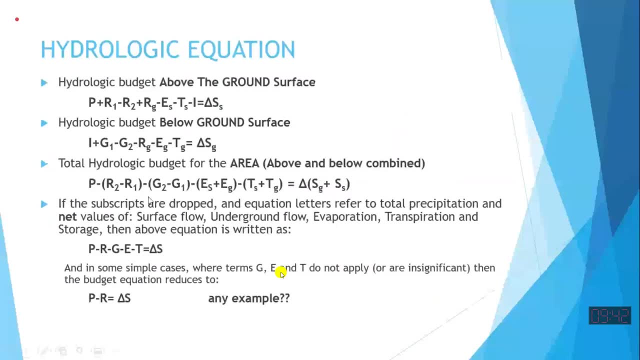 to the whole globe. so then we say this is a closed system. how to write a hydrological budget equation? please carry out your own experience: make a watershed label, all the inflows and outflows and the storage is over there, and then write hydrological equation without seeing this. 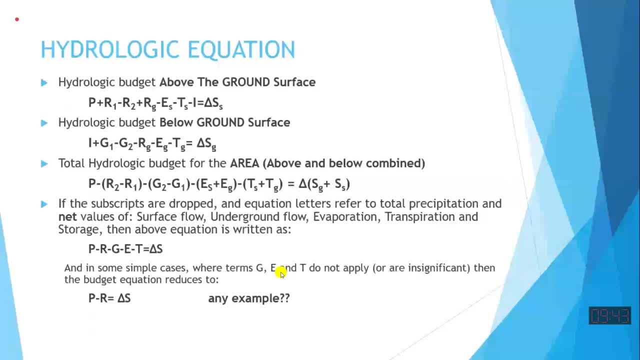 slide: write hydrological equation for surface water. write hydrological budget equation for ground water. add them together and write the complete equation. so the same equation is written in another form, in this, in a simplified form. if we say, net outflow of the surface runoff is represented by r. 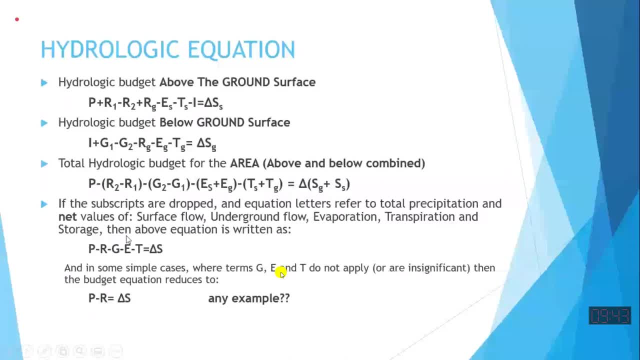 if net outflow of the ground water is represented by simply g, if net outflow through evaporation from the surface and the ground is represented by e and if t is the total transpiration and if t is the total. so evaporation is not net, it is a. 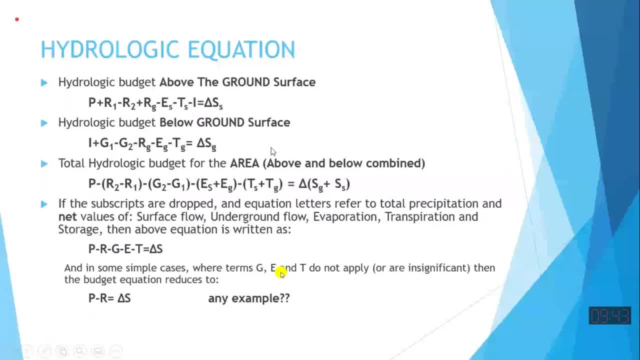 total evaporation and total transpiration is written as t, so then we can say that inflow minus outflows, net runoff, net, ground water, total evaporation, total transpiration. so above equation. this equation can be written in a simplified form as: p minus, r minus, g minus. 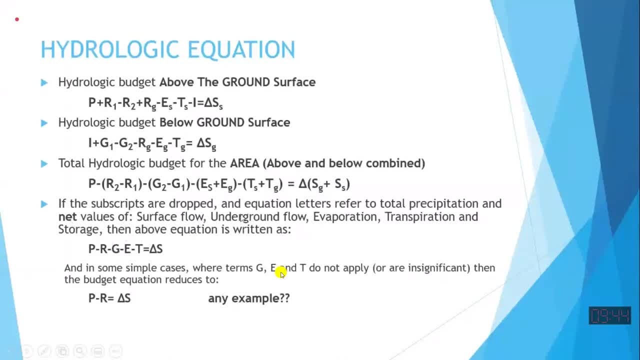 e minus t is equal to delta s. so same equation is written in another using another nomenclature of five different processes. so r for runoff, net runoff, or you should keep in mind, r means outflow minus inflows of the surface, g means outflow from the ground, 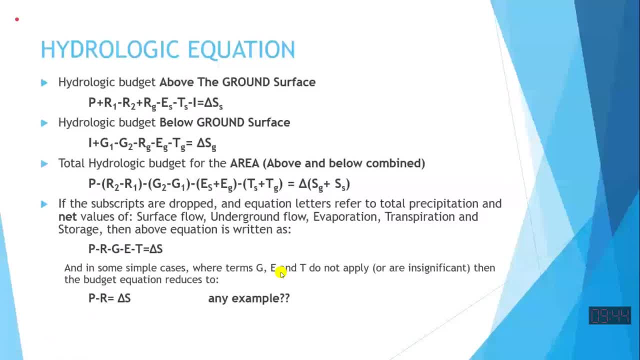 water bodies to the surrounding ground water bodies, minus inflows to the ground water body from the surrounding ground body. so and where is the i gone? because in these two equations i was coming here i was outflow, over here i was inflow. so that is balanced. 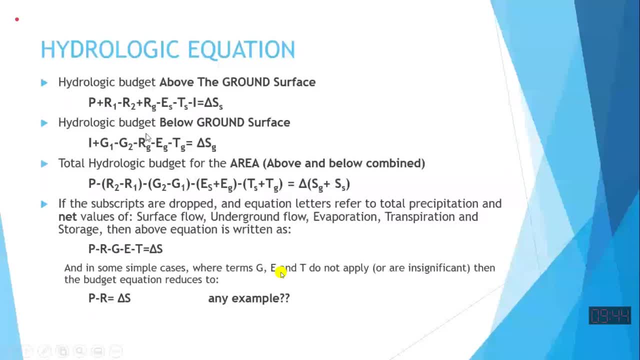 out when we are writing the equation for both system together. i infiltration is not going out of the surface plus ground water system. it is moving from surface to ground and then rg is coming from ground to surface. so both of them have vanished away while we are writing this. 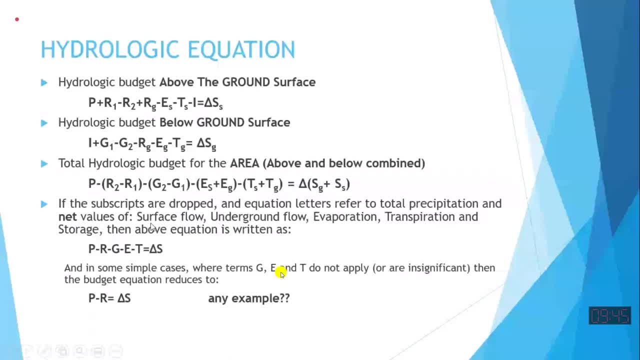 equation together. so sometimes this evaporation, transpiration and the contribution of the ground is very small. if that is the thing we can say- g is zero, e is zero, t is zero- then we can say that precipitation minus surface runoff is equal to change of storage. so 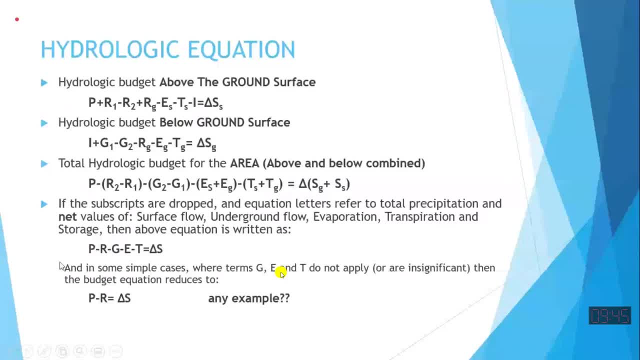 these equations can be simplified in special cases, not always, but in special cases. this case, special case, any example comes into your mind where i can say transpiration is not there or evaporation is neglected, any system which comes into your mind. for example, you have a canal body. 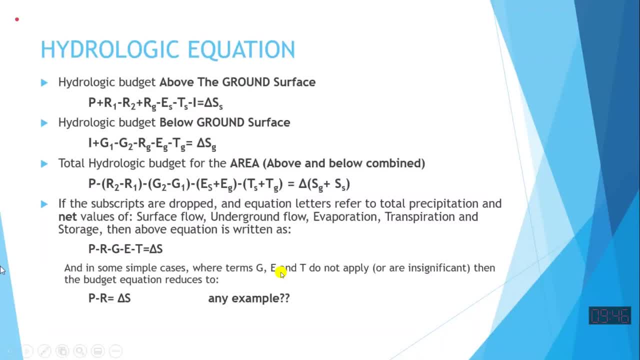 for example, you have a reservoir, small reservoir, and you are writing its water budget equation for, let us say, few hours or few days. so usually if i am writing equation for reservoir and if i consider that there is no seepage out of that reservoir- although it is not true, 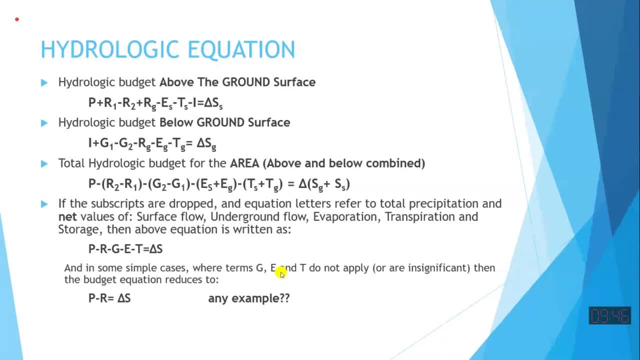 seepage occurs through the reservoir underneath. if i assume evaporation within one hour or one day, the time period for which i am analyzing is ignorable. whatever is the precipitation in that reservoir minus net outflow of the water to the reservoir will be equal to the change. 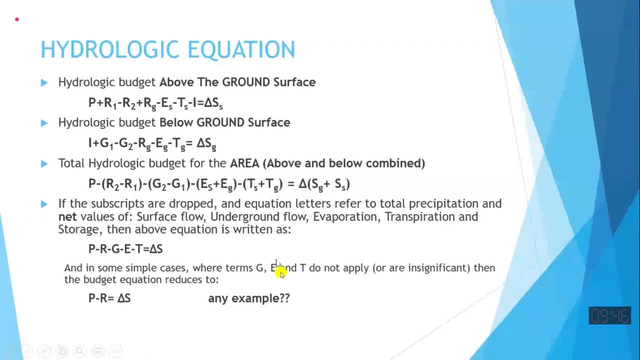 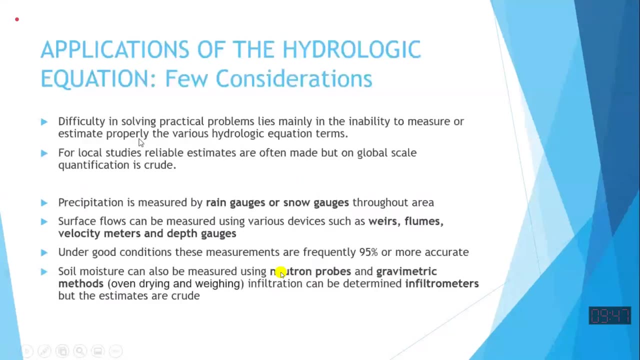 of the storage of that reservoir. such things can be written in simplified cases, so you should be able to write hydrological budget equation, please. ok, while we apply the hydrological budget equation and what problems or difficulties we face and where it can be used are highlighted in these two slides. 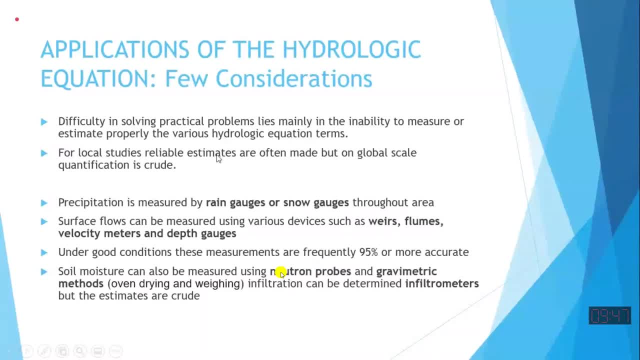 sometimes we are not able to measure different components. for example, it is difficult to measure evaporation which is occurring from a catchment. evaporation from a catchment is difficult to measure. how can i measure how much is evaporation happening? so alternate way we are doing. 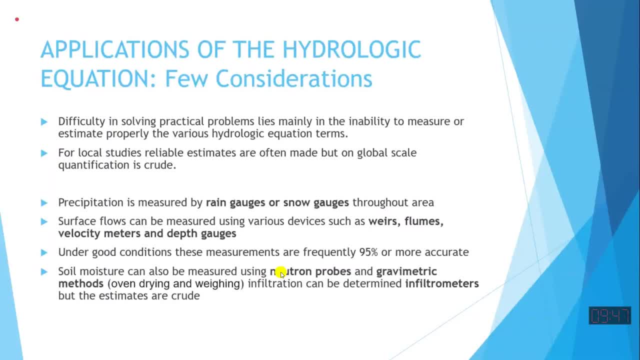 that we assign. we place in that catchment pan evaporator 1.5 m diameter, 1.2 m diameter. we fill the pan with water and we daily measure how much is the reduction of water in the pan so that we use to estimate evaporation from that area. 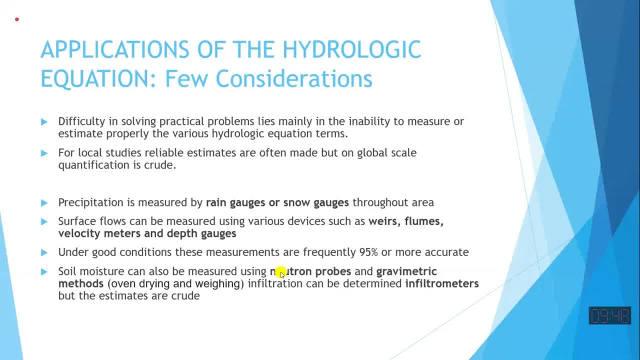 similarly, it is difficult to estimate transpiration, so detailed studies are then there. we tell them to measure evapotranspiration- we call them lysimeter studies are carried out. so we have to give you a message that some components of the hydrological budget equation are easy to measure. 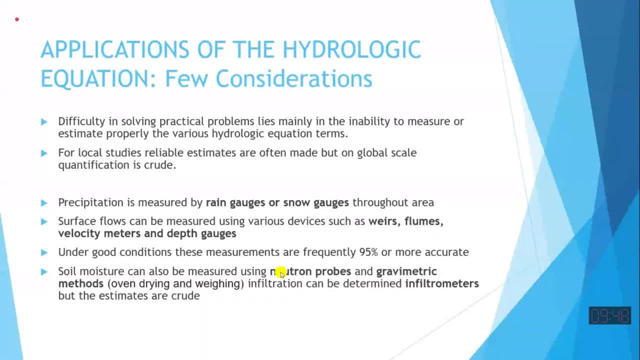 but some components are difficult to measure. for example, rainfall accurately is difficult to measure but to much of the extent we can estimate the rainfall using the rain gauges. rain gauges are small pans, 8 inch, 10 inch diameter pans, which collect the water, and every day we measure. 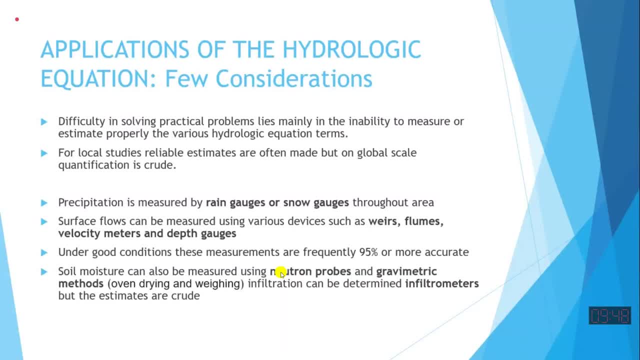 how much depth of water is coming in that area of the pan rain gauge. so that rain gauge is for that 10 inch area. so we don't have all the surface covered with the rain gauges and we cannot do it. it is highly costly and we don't need it. 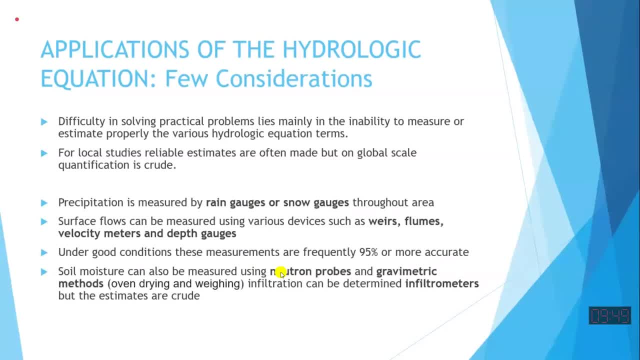 rain does not change much. but we estimate from observation in a rain gauge and we assume that surrounding area will be having similar rainfall. so from that we estimate rain. similarly we estimate snow from the snow gauges. the surface runoff we can accurately measure. to much extent we can measure. 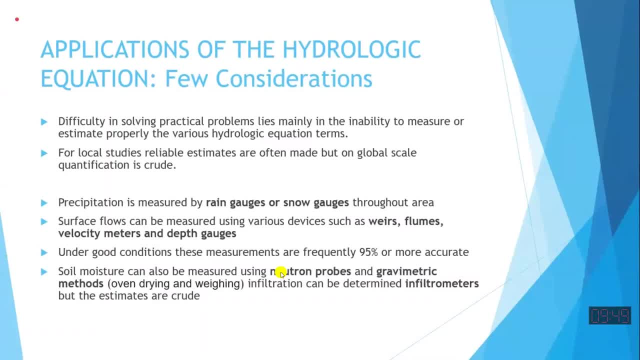 we can have gauges installed on the rivers. they give us the velocity of the river and then we also measure the cross sectional area of the river, velocity multiplied by area. but we cannot measure the flow of the ground to much extent. how much water is coming from the surrounding area? 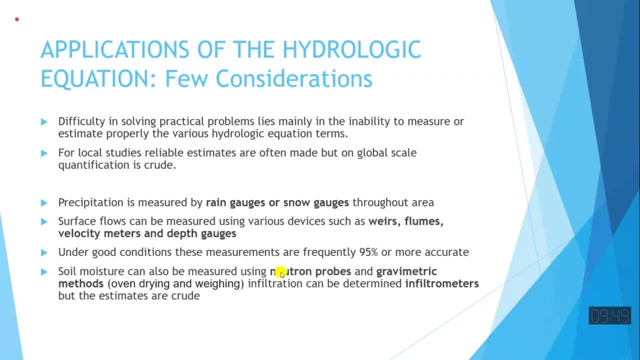 in this part ground water, so that we have to rely on estimates accurately. we cannot measure. we see. what is the water, ground water depth at this place. what is the ground water depth at this place? so from the level difference, we estimate the gradient or slope of the ground water surface. 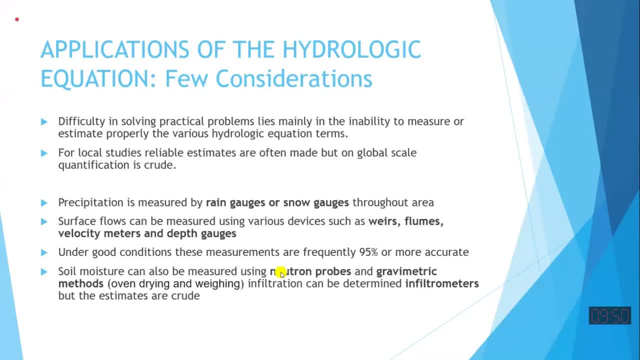 so that slope is usually used to calculate ground water flow using Darcy equation KIA. I is the gradient, K is the permeability of the soil- how much is soil permeable- and A is the flow area. so those are estimates for ground water flow, sometimes soil moisture. 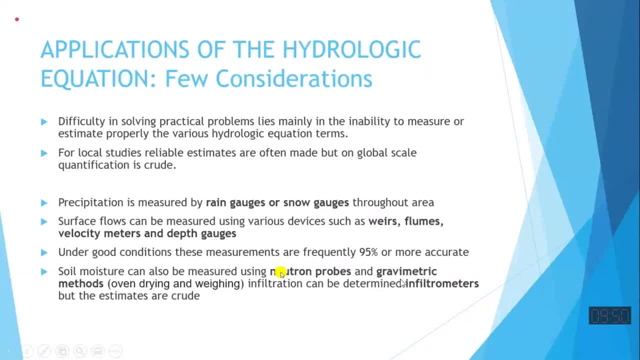 we have to estimate to see the change of the storage in the soil. so the method of moisture content we have told in the class is called gravimetric method, so that can be used to estimate the soil moisture today, tomorrow, day after tomorrow and to have the idea how much. 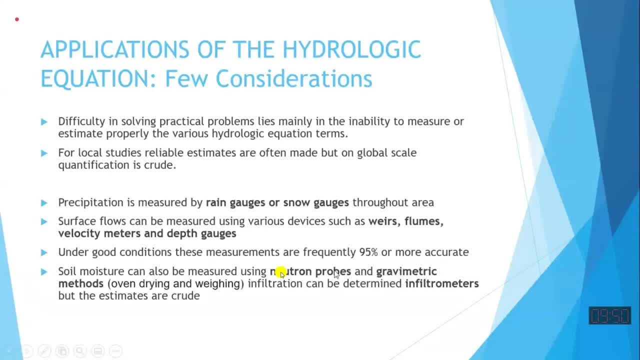 is the storage change in the soil. sometimes we use neutron probes. this is the modern apparatus. neutrons are used to estimate the moisture quantity available in the soil. those soil which have more moisture have more hydrogen. so neutron speed is reduced in that and from the speed of the neutron 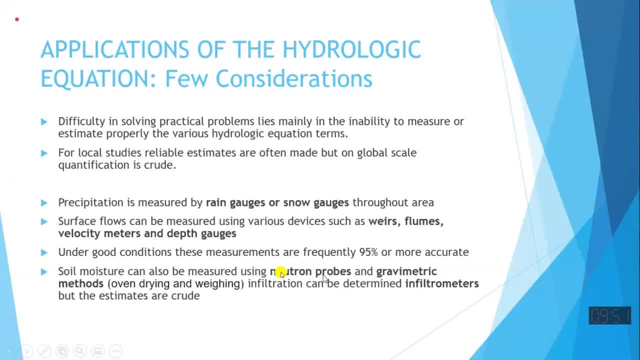 or the reflectance of the neutron, we can have the estimate how much water is available. but more simple method is this moisture content measurement using gravimetric infiltrometer. sometimes we use to estimate infiltration. this is simply a steel ring one and a half meter diameter. 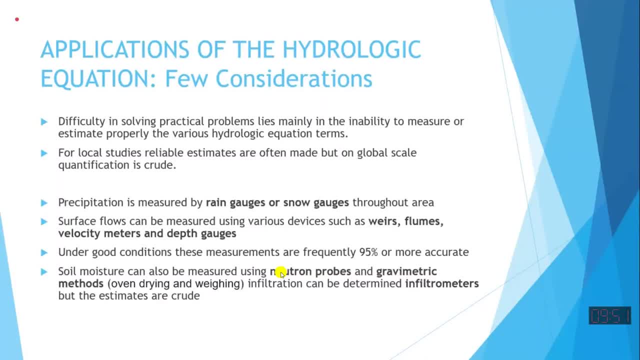 steel ring, we put it in the soil at the surface of the soil, we insert it into the soil and we measure the water and every day we see how much water is going down into the soil. or every hour we see how much water is going down. so from that measurement, 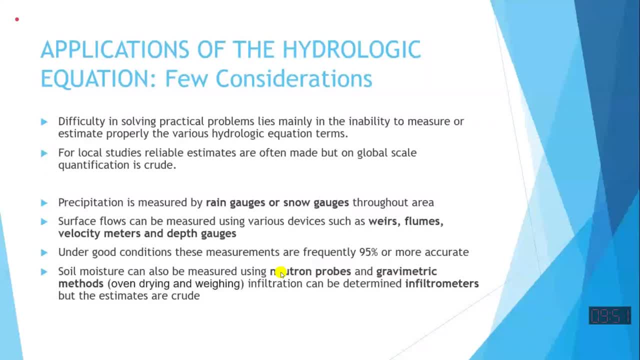 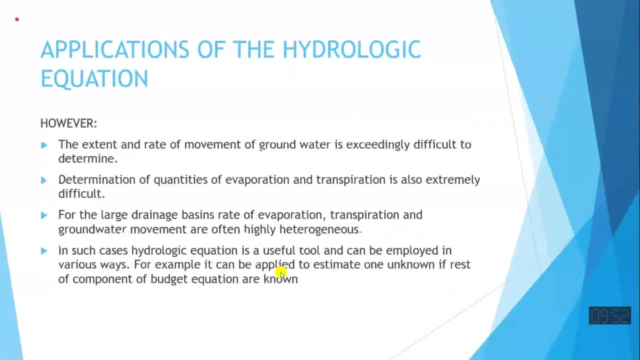 we estimate this soil has so much infiltration capacity so that can be used to estimate the infiltration of the whole area infiltrometer. so we have equipments to measure some of the components to measure. determination of the quantities of evapotranspiration is difficult to measure, so if we have to estimate, 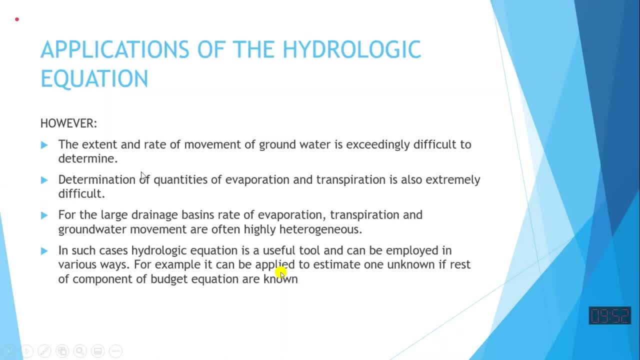 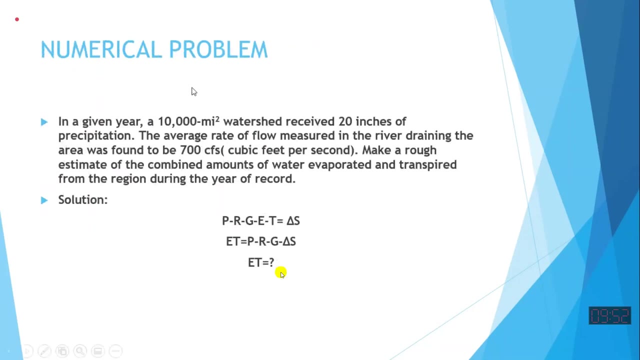 these things, for example evapotranspiration. so sometimes hydrological budget equation are used. we measure all the rest of the things and we estimate the unknown thing from the hydrological budget equation. so one of the such problem is given over. here there is a certain area. 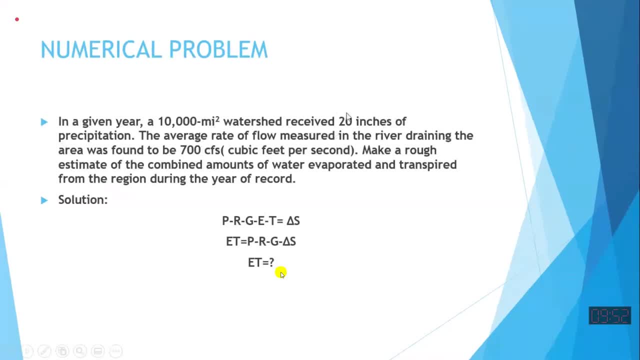 and it has received precipitation. 20 inch rate of flow measured in the river draining, the area was found to be 700 Q6. so in that river rate of flow, which is rate of the flow measured in the river draining, the area, so outflow, is given 700 Q6. 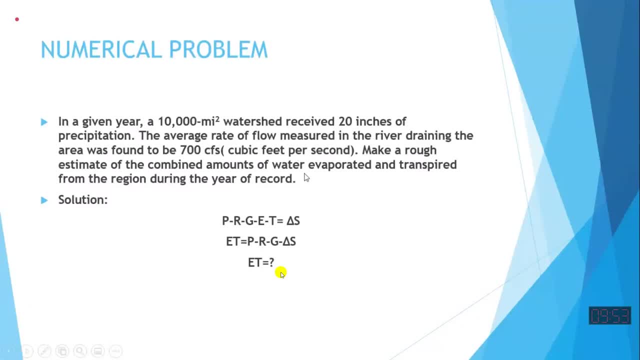 make a rough estimate of combined amount of water during the year. so they are saying that tell us how much will be the estimate of evapotranspiration from the region. now, if you see they are not telling what is happening to the ground water, so it means they are assuming that. 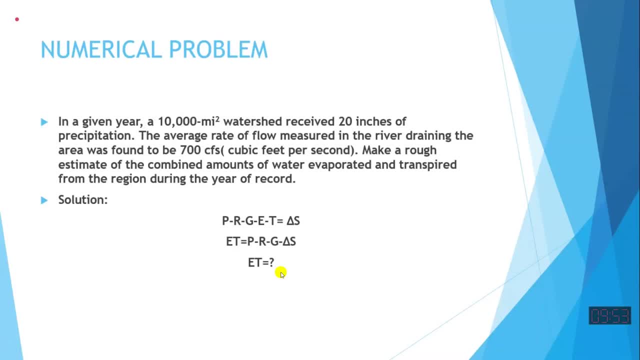 ground water over the year remains constant. and what happens normally? in the monsoon season ground water rises and in the dry season ground water goes back down, and over the year we say that the ground water changes negligible, at zero. so if that is the case, then we don't need the estimate. 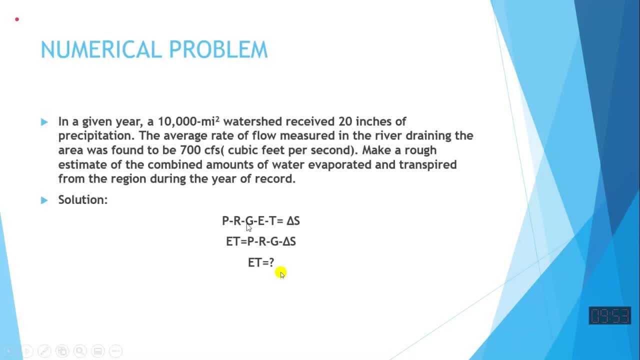 of the ground water. so they have used the equation of the budget that precipitation minus net runoff minus net ground runoff, groundwater contribution minus evaporation minus transpiration is change of storage. so in this catchment we assume that soil moisture and depression storage and these things over the year. 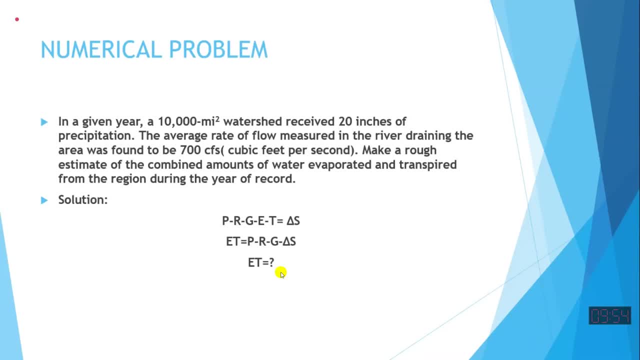 they are not varying. they are varying from day to day, but from the 1st january 2019 to 2020, within the year, the overall storage is in the area remains same as the previous year. so then change of storage we can assume is zero. 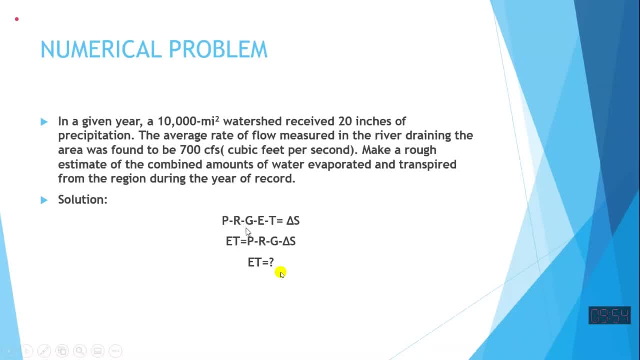 so then precipitation minus surface runoff will minus e and t will be equal to zero storage change. so when this we can write, then e plus t can be estimated. e plus t together can be estimated writing this equation: p minus r, minus g, minus delta s. so this can be solved. 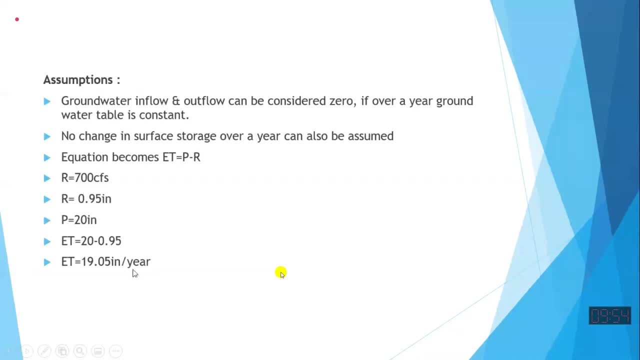 and answer will be 19 inches per year. so what are the assumption? ground water, inflow, outflow are considered zero. no change in surface storage. so we have taken delta as zero. similarly, g is taken as zero. so the rest are the things. we have changed the units. 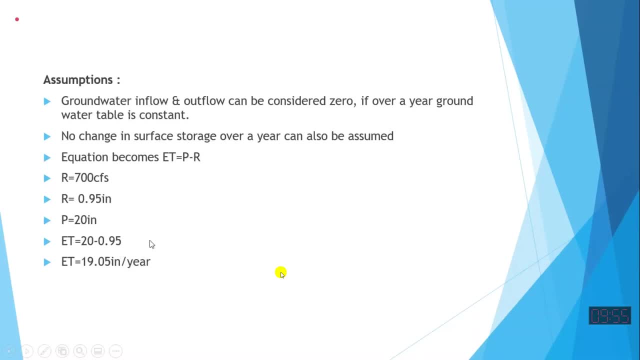 and finally, everything is computed in inch units. rainfall is already in inches. surface runoff: 700, q6. you have to convert it into inches. this q6 need to be converted into inches for one year. how much is water coming? you can calculate 700 into the seconds in a year.